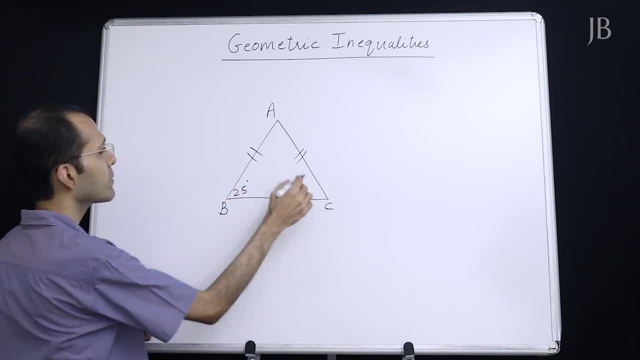 degrees. Angle B is 25 degrees. How much will be angle C? 25 degrees? because angles opposite to equal sides are equal. Now, this 25 degrees is opposite to AB, and then you have another side, AC, But the two sides are equal. If two sides 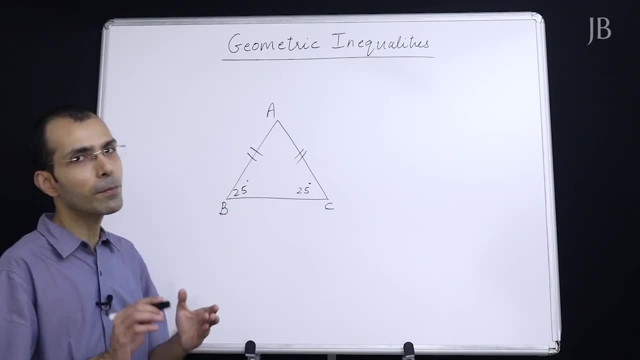 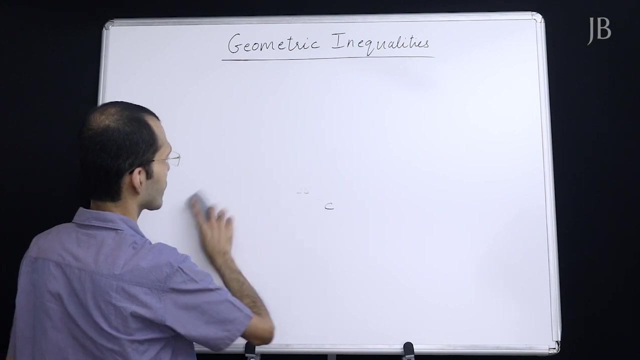 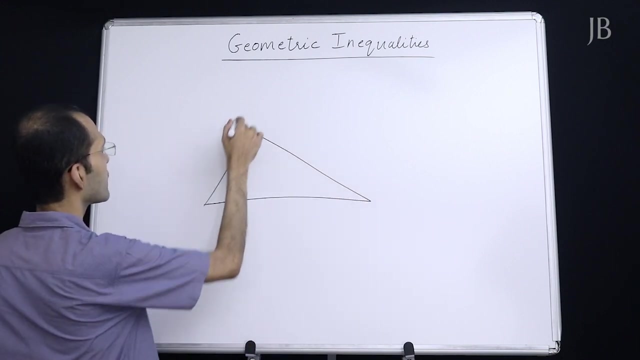 are equal, angles, opposite to them also will be equal. This you know very well. However, what happens if one side is greater and other one is shorter? Then let us see what happens. Quite interesting. Take this triangle. Say PQR, Now QR is. 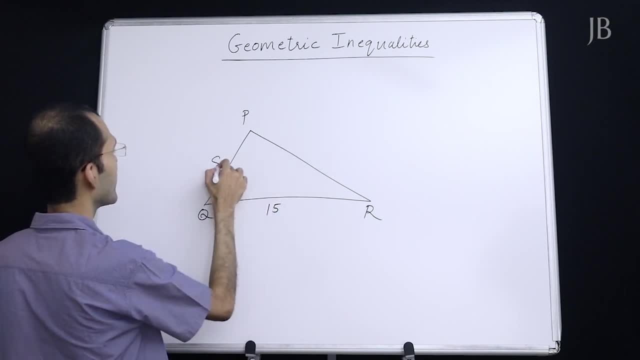 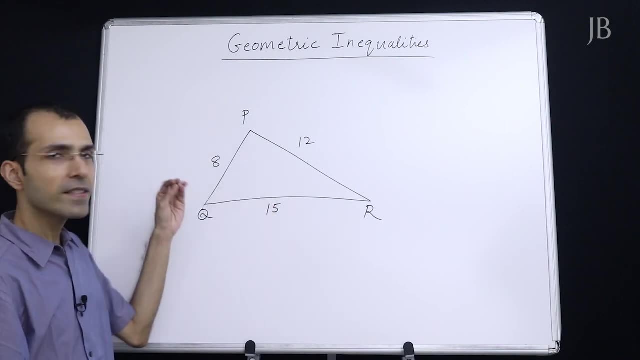 suppose 15, PQ is say 8 and this is say 12. So scale in triangle, PQ is 8 centimeter, QR is 15 centimeter and PR is 12 centimeter. Let us denote the angles by X, Y and Z. 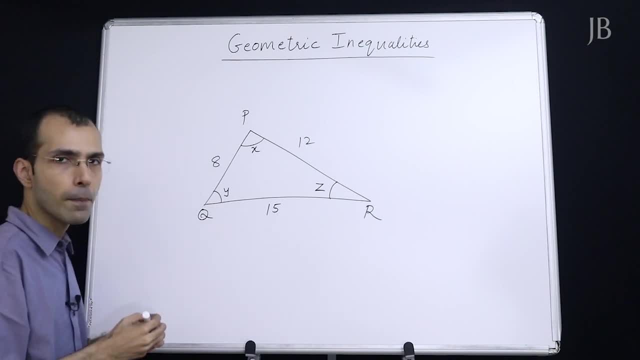 X, Y and Z. Now we wish to find out which angle will be the least smallest. Okay, it's a scalene triangle. Now, in a scalene triangle, all angles cannot be equal. All angles will be different. So x will not equal, y will not equal z All. 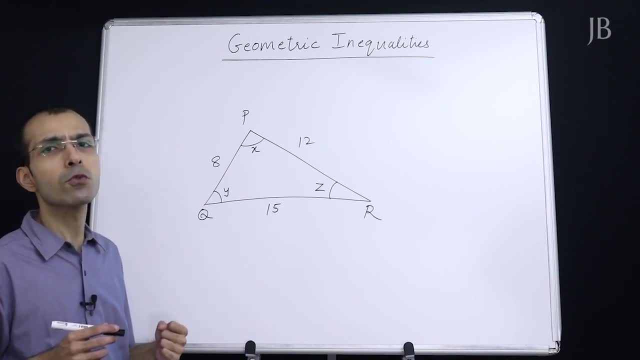 angles will be of different measures, But we are curious to know that which angle would be the greatest. Now, one thing is that you actually construct this triangle, Okay and see, but then there should be some theory right which will tell us which angle is greater. 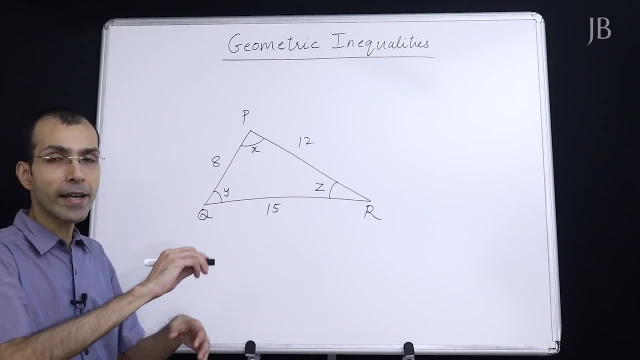 which angle is the smallest, which is the greatest, without you actually having to construct the triangle every time. So the concept is simple. It says: angle opposite to greater side is greater, Simple Angle opposite. So this is the first concept. Okay, if you wish, you can take down this concept by pausing. 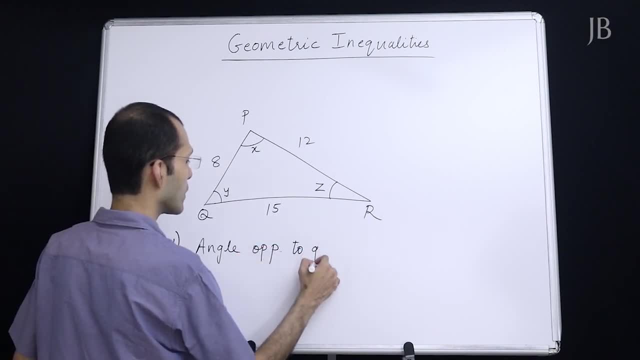 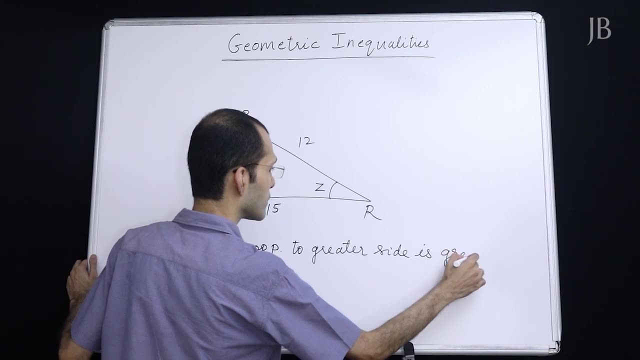 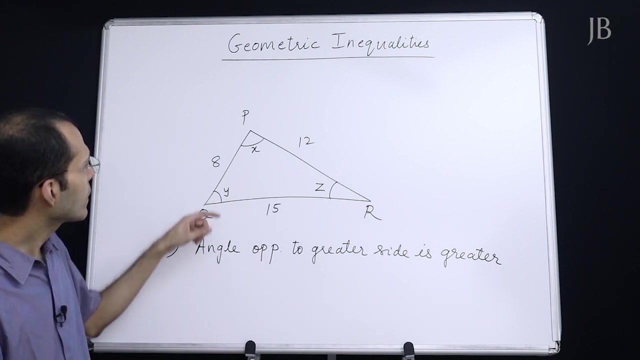 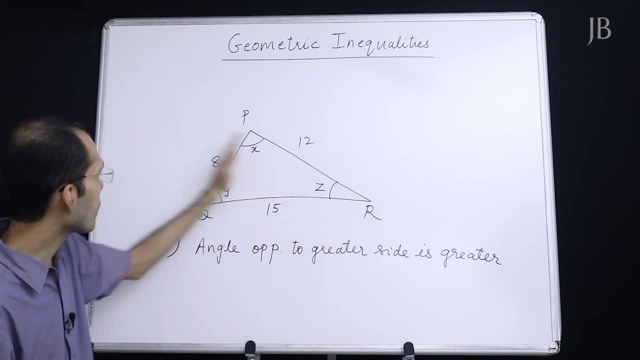 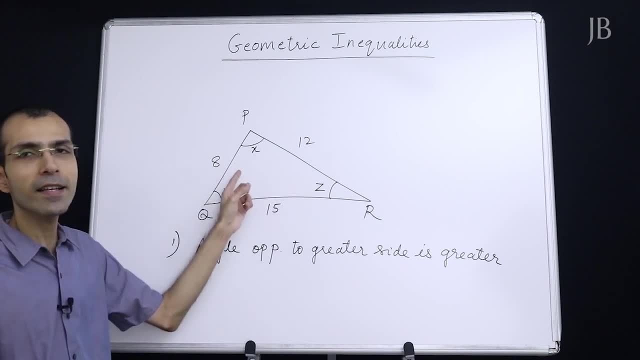 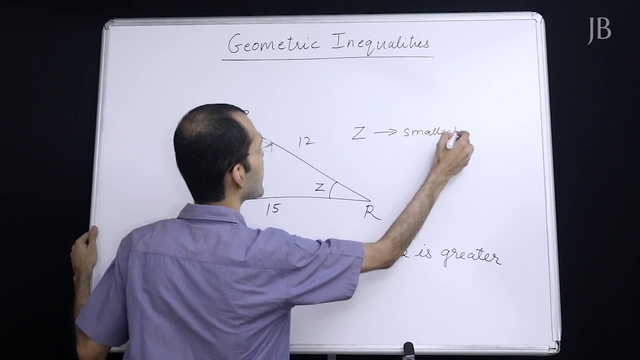 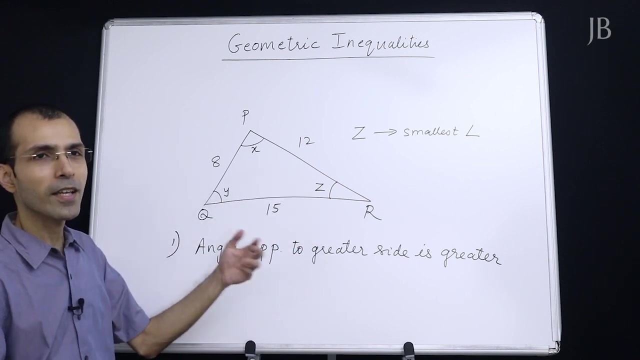 doubt. Which is the angle opposite to 8? z. So here z will be the smallest angle. z would be the smallest angle. How much it is, we do not know. There are ways of finding out, okay, but we are not using that like the sine rule and the cosine. 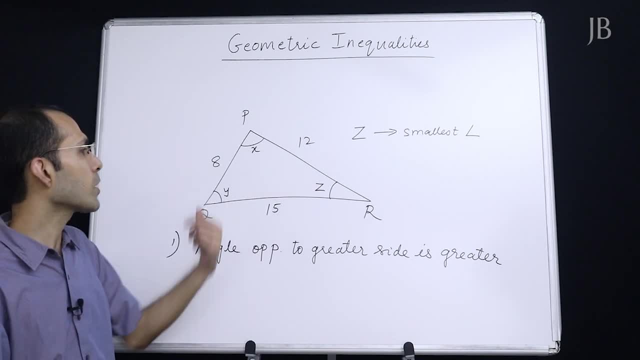 rule and all which will come in class 11th, We can find out what would be the measure of angle z, because your normal regular trigonometry, what you use in school, can't be applied here because that can be applied only for right angle triangles, but actually trigonometry can be applied even for non right angle. 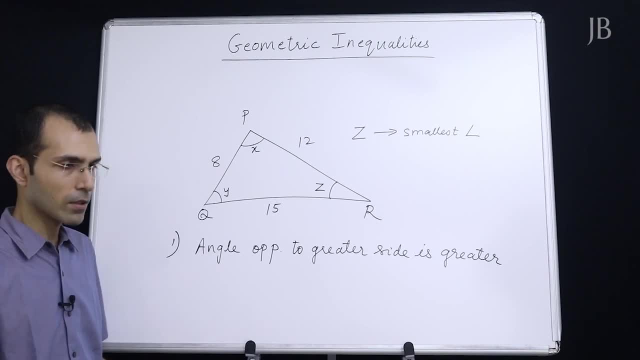 triangles And you are not aware of those formulae because they are not there in our curriculum. They will be covered in class 11th and 12th. Okay, otherwise we could have worked out angle z and x and y easily, if we know. 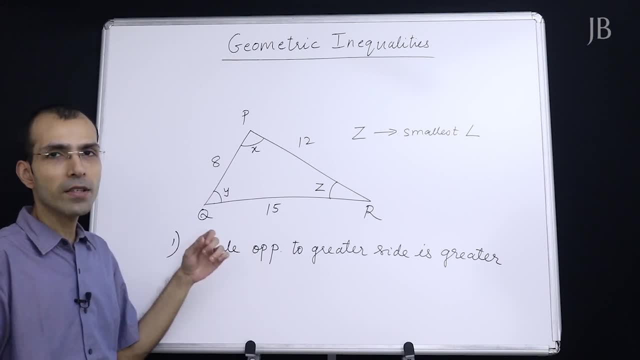 all this Fine. here we are interested, not interested in knowing the measures of the angle, We are simply interested in knowing, out of three angles- x, y and z- which one will be the greatest, which one will be the smallest and the left over. 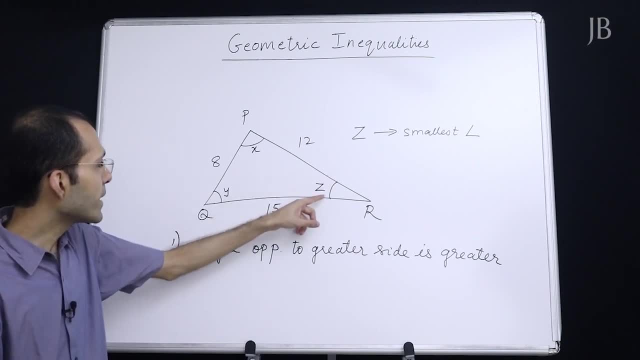 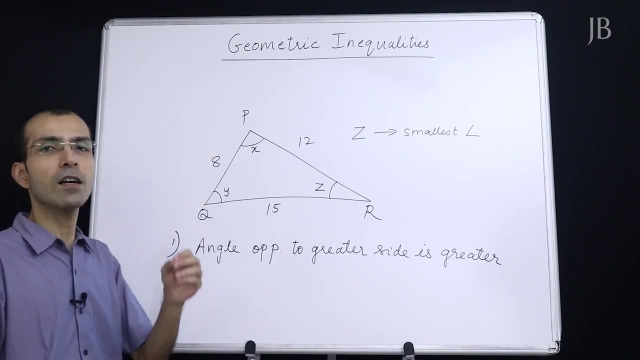 will be in between. So here z is opposite pq, that is 8 centimeter, and pq happens to be the smallest side in this triangle. So what is opposite to pq, z? So z will happen to be the smallest angle. Okay, which is the biggest side here? 15, right, 8, 12 and 15 may say. naturally, 15 is. 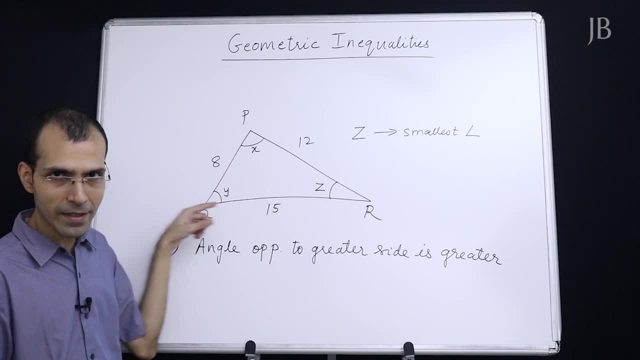 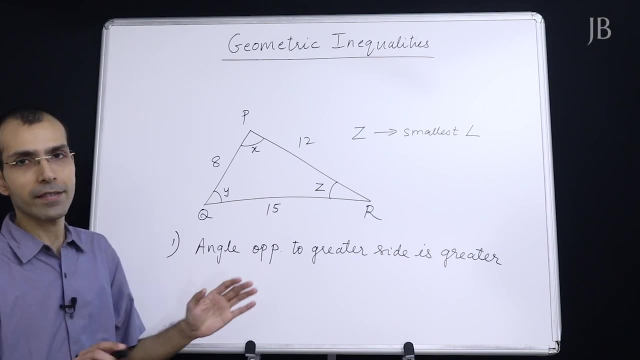 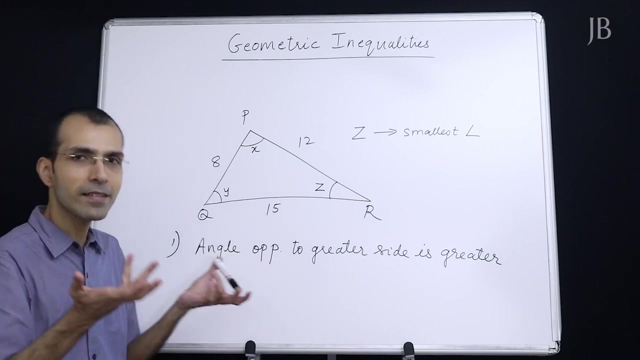 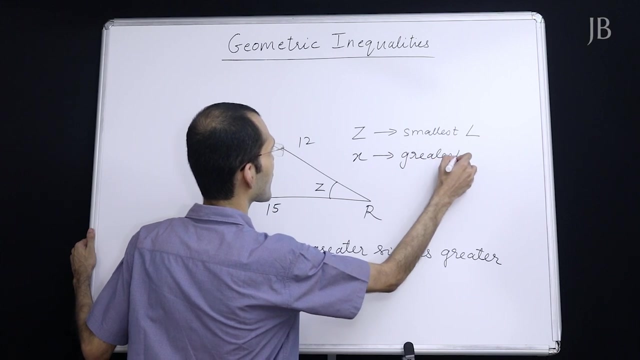 the biggest side. If 15 is the biggest side, which angle is opposite to 15? x. So x would be the greatest because side wise 15 is the greatest side. So angle opposite to greater side is greater. So here x would be the greatest greatest angle. and in 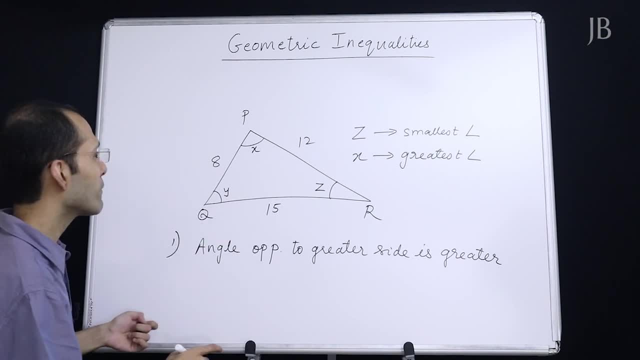 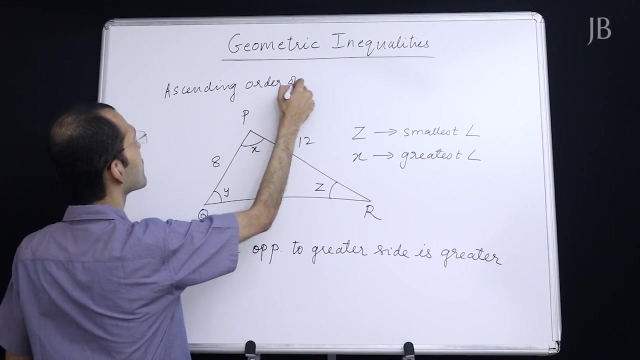 between will come y in between. So if we wish to arrange this in ascending order, if you wish to arrange x, y, z in ascending order of their magnitudes, ascending order means small to big, So which is the smallest? So ascending order, ascending order of angles, So which is the smallest? here we 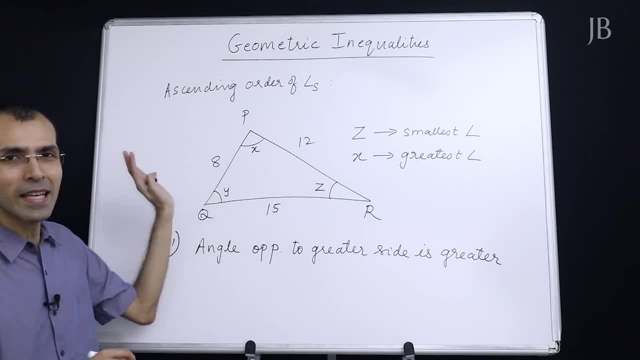 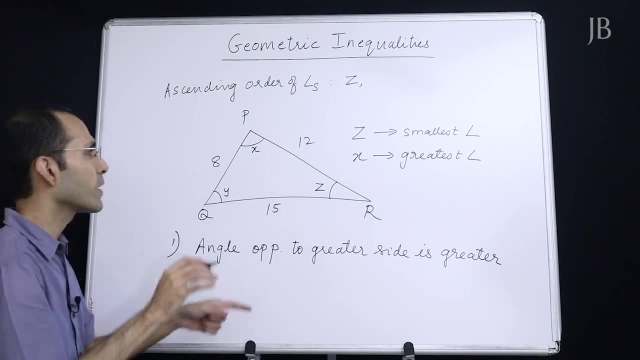 decided z because z is opposite to 8 and 8 happens to be the smallest side, So z angle z also will be the smallest of all the three. What it will be, we are not concerned, But it will be the smallest and which is the greatest angle. 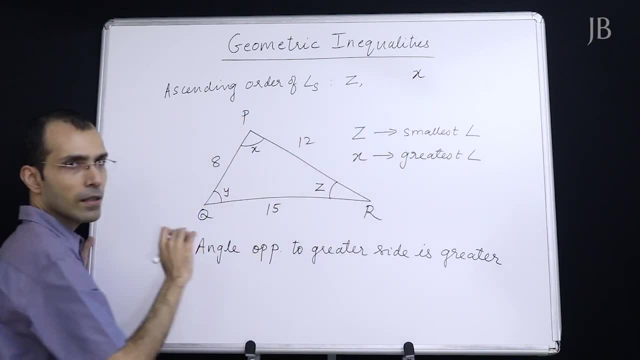 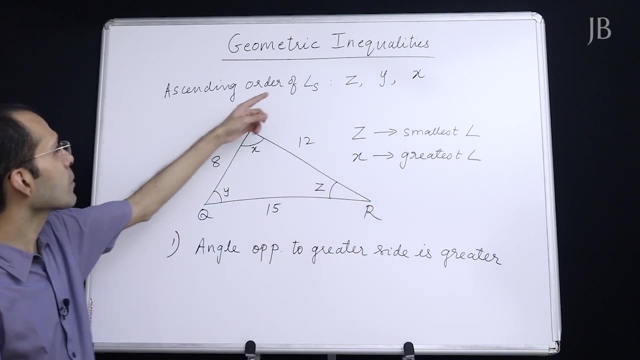 x And in between will come y, that is the left over angle. So in ascending order of angles, magnitude of the angles, if you go it will be z, y and x in this particular case. So what is the concept? angle opposite to the greater side is greater. We also have the converse of this concept. 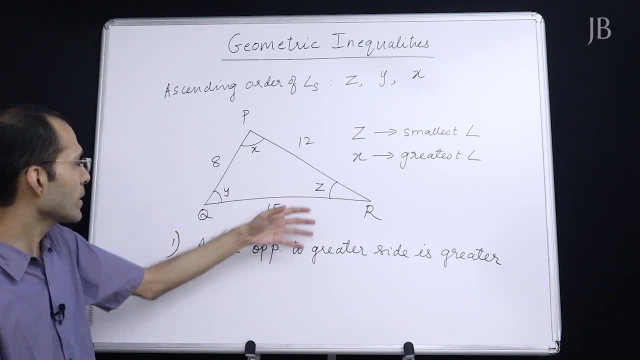 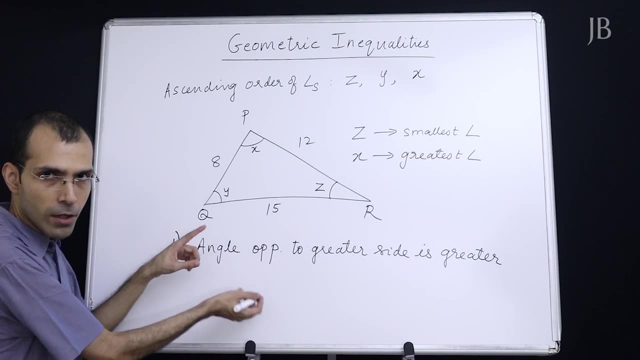 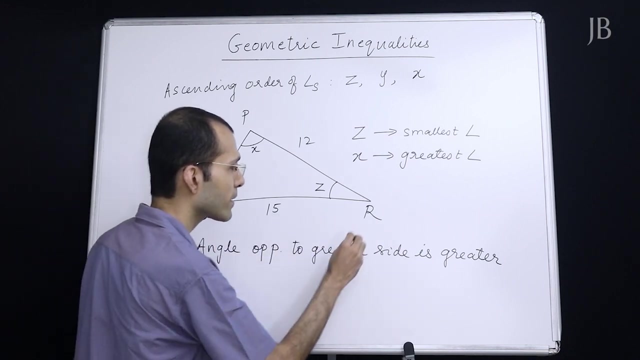 Is this clear? first of all, Right here, sides were known and we drew some conclusion about the angles. Now we will have converse of this concept. First, understand this concept one more time: Angle opposite to greater side is greater. So here there were three sides. 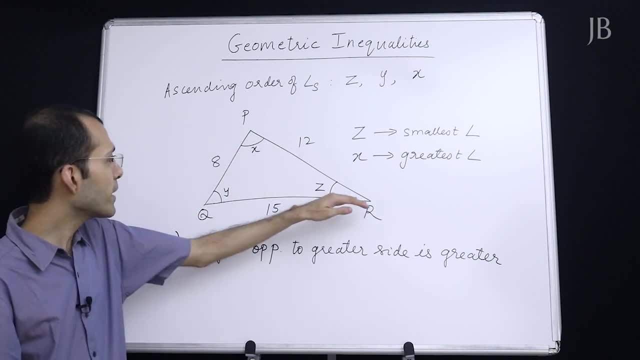 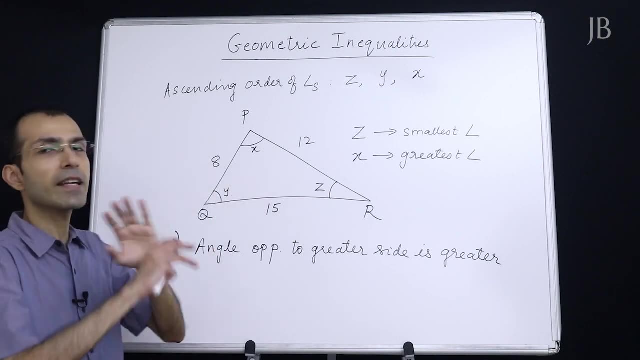 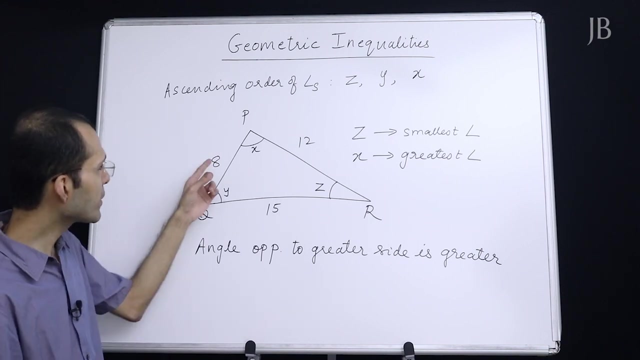 8,, 12 and 15.. 15 was the greatest side, naturally, So opposite to that angle is x. So x would be the greatest angle of all the three. 8 happened to be the smallest side, Which is the angle opposite to it, Z. So Z will happen to be the smallest angle. 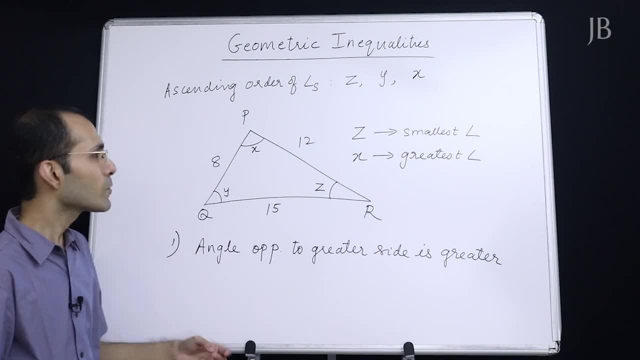 And then we will have converse of this concept, We also have converse of this concept. We will have converse of this concept, We will have converse of this concept, And then the left over will be in between them naturally. So sometimes they can ask you arrange the. 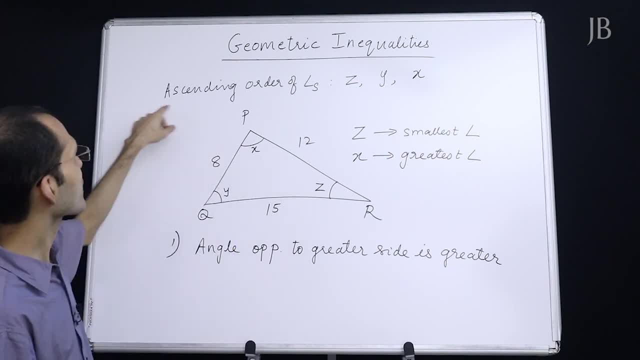 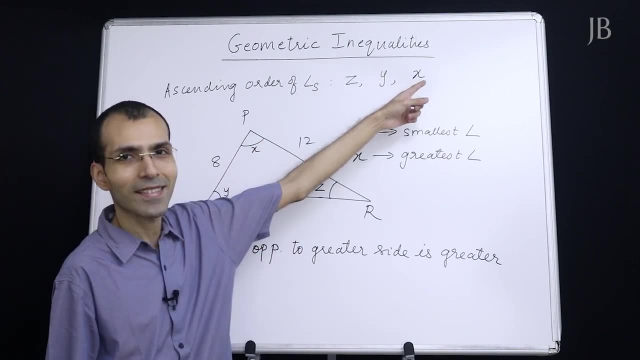 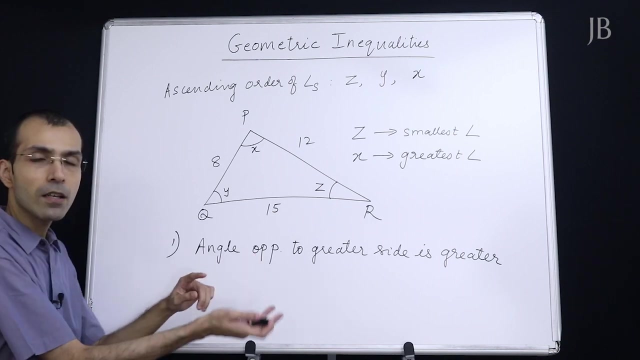 angles in ascending order of their magnitudes. So ascending order means small to big. So smallest was Z, The greatest was x, In between y and we are done with it. So this was first concept. Now we will study converse of this concept. What would be the converse of this? 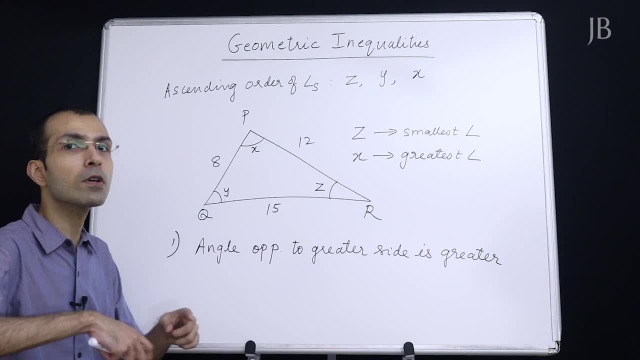 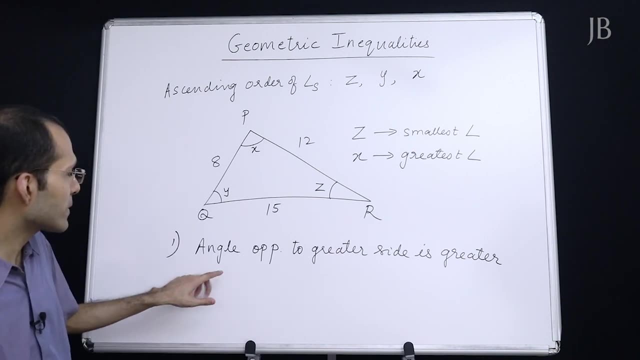 Side opposite to greater angle will be greater. Now we will give importance to side. The original concept is: angle opposite to greater side is greater. The converse of this concept will be: side opposite to greater angle will be greater. So let's have a look at that. 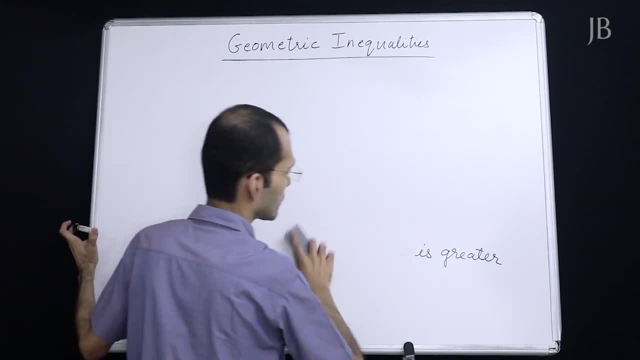 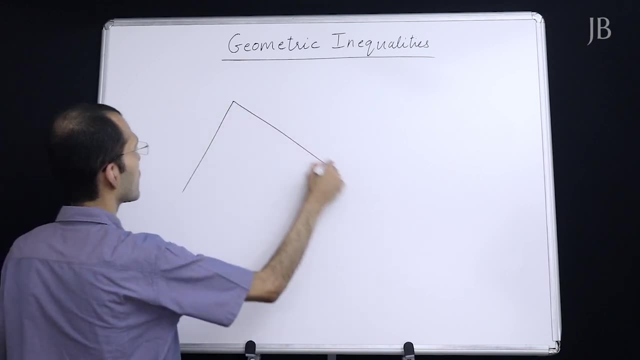 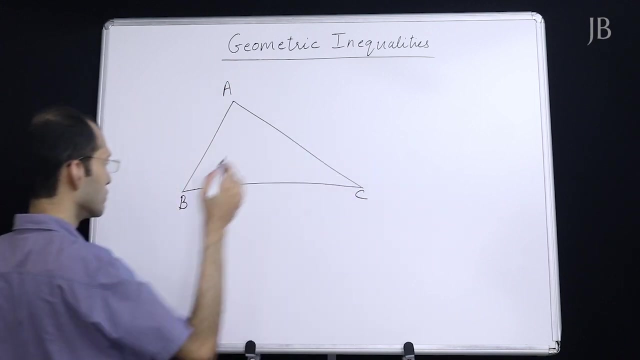 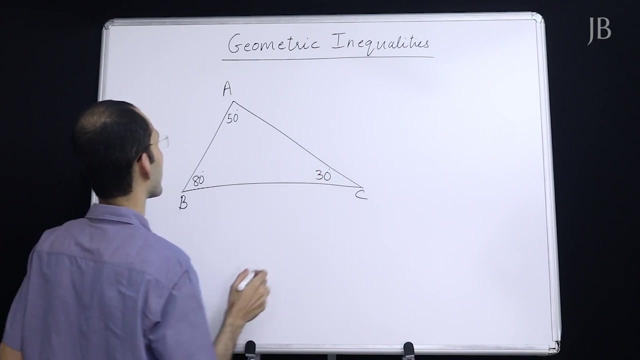 Okay, let's consider your triangle ABC, A scale in triangle. This time the measurements of the angles are given. So, say, this angle is, say, 50 degrees, this is 80 degrees. So naturally this will be 30 degrees, No 80, plus 50, 130.. This also will be 50.. Wait, let me change. 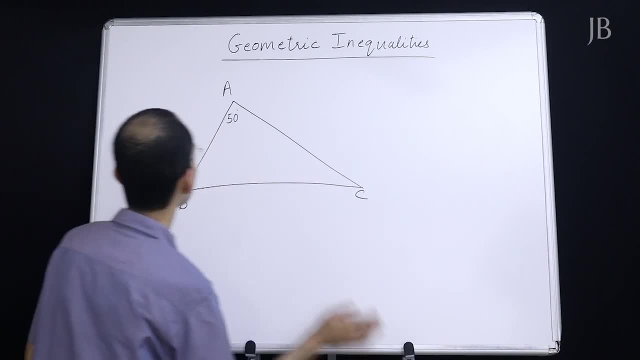 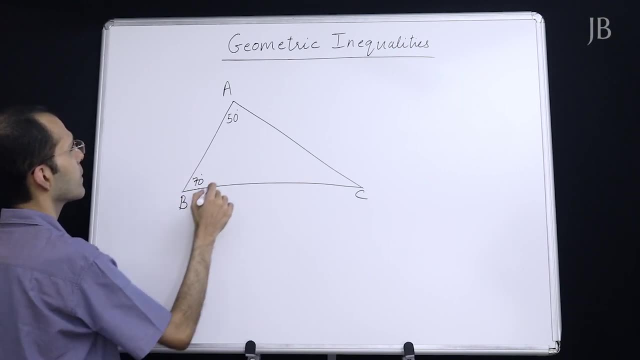 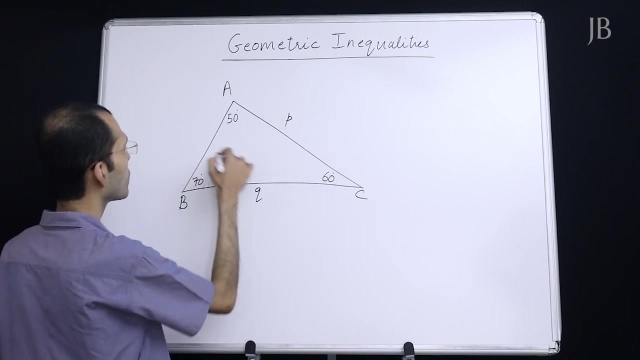 the measurement. See, this is 50 degrees, Let this be 70 degrees and this will be 60 degrees. then Some of the angles of a triangle, always 180. So this is fine. Now the sides we denote by, say, P, Q and R: See, initial setup is clear. You have a triangle ABC. 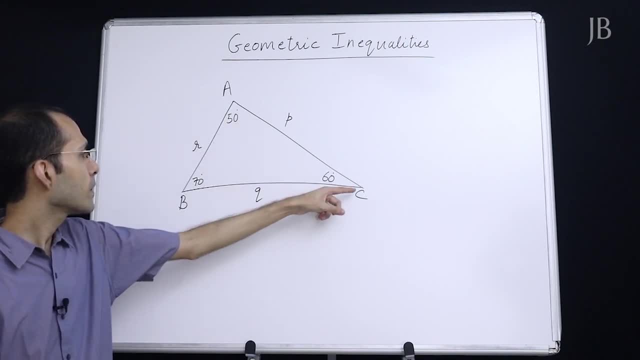 you have the sides P, you have the sides Q and you have the sides R. So P denotes length of segment AC, Q denotes length of segment BC and R denotes length of segment AB. Okay, and these angles are given. Now, which angle is the greatest here? Naturally, 70.. 70 happens to be the. 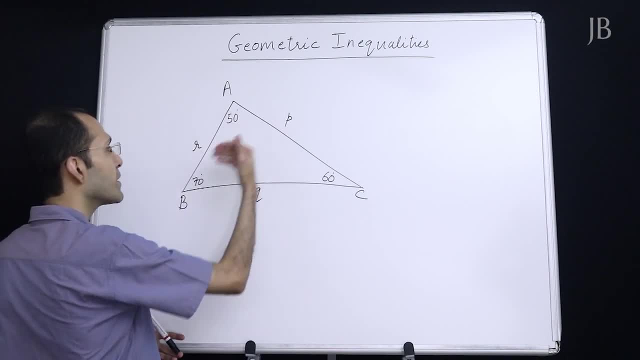 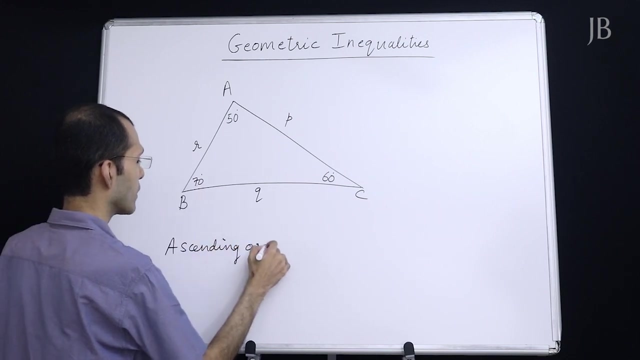 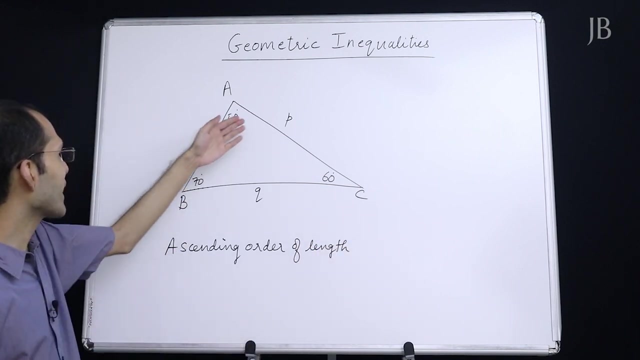 greatest angle, So the side which is opposite to it. the side which is opposite to it would be the greatest in length. So, lengthwise, ascending order, ascending order of length. Here we are now trying to find out. See, we know these angles. now The situation is exactly. 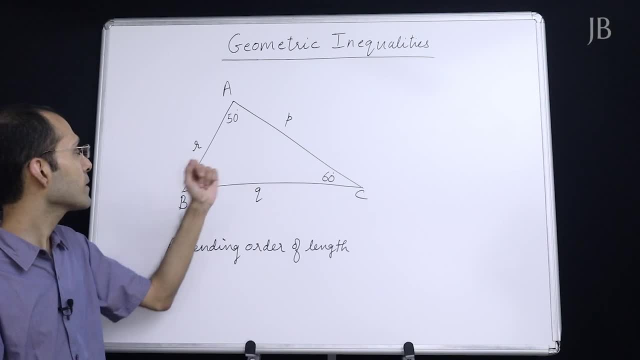 ulta of the first one. Here we know the angles. We just wish to find out which side is the smallest lengthwise and which side is the greatest. So what we do, simple: We catch hold of the greatest angle, Which is the greatest angle of 50,. 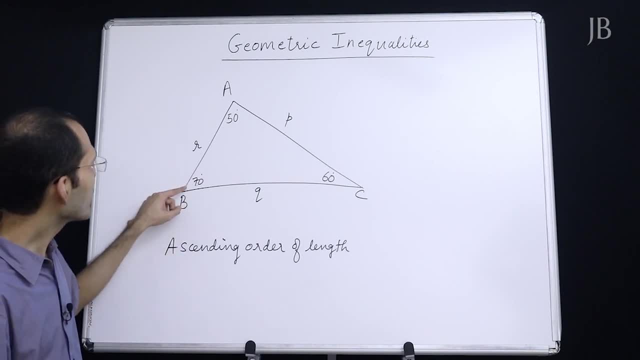 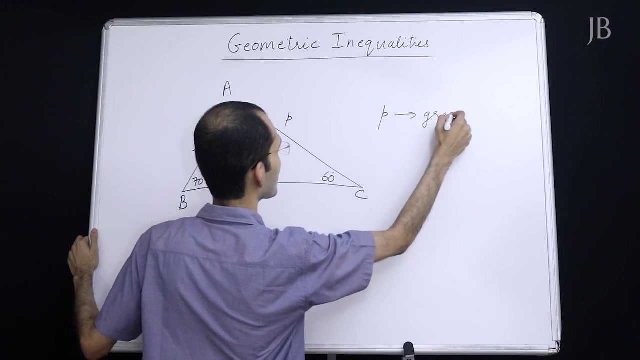 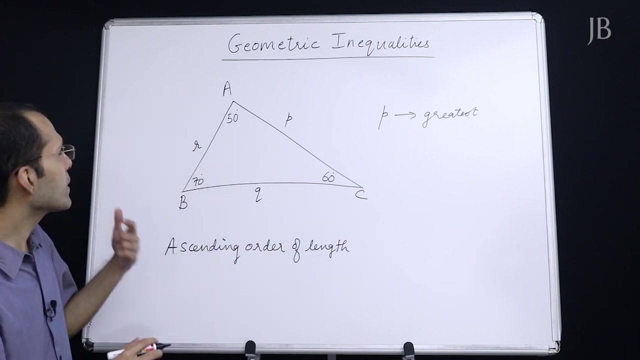 60, 70?? Naturally 70. Which side is opposite to 70 degrees AC and whose length we have denoted by small p. So p would be the greatest length. okay, P would be the greatest. Greatest means what? Greatest in terms of length? What would be the? 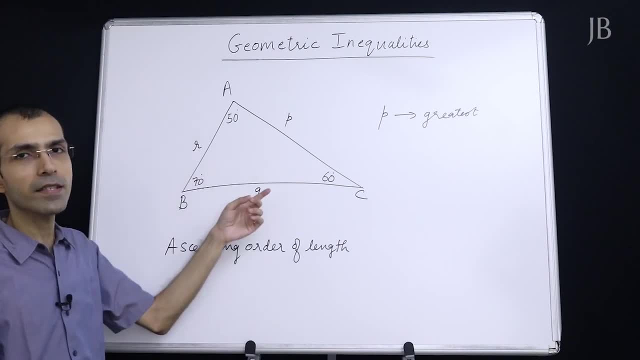 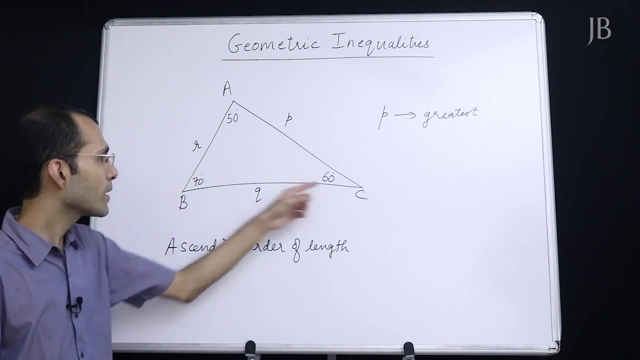 smallestamping angle. Which angle is the smallest here Out of 50,, 60, ,70, which one is the smallest? 50 degrees. no dispute in that degrees. Opposite 50 degrees. which side is there? BC, whose length we have? 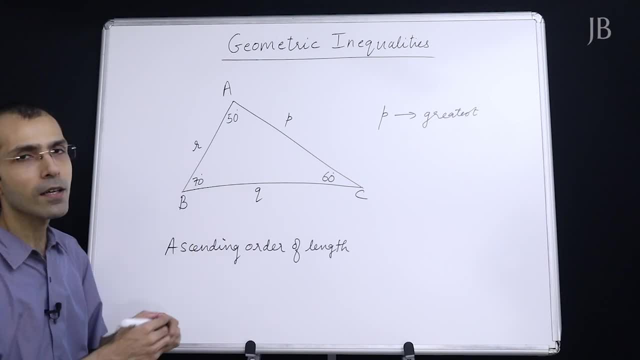 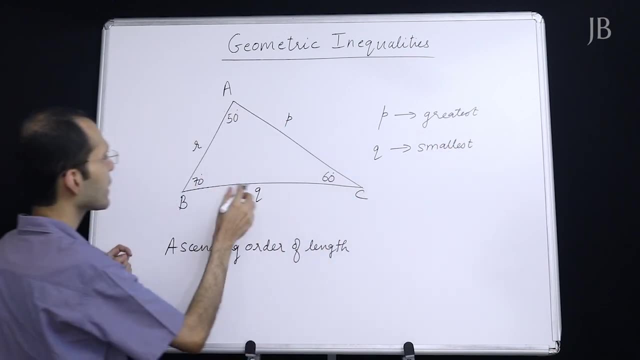 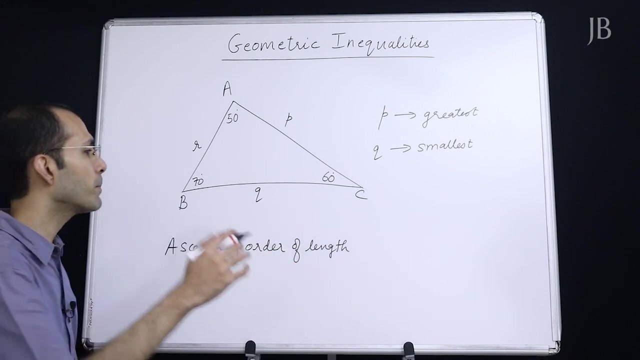 denoted by Q. So Q will become the smallest, Q will become the smallest side, And then naturally now R will come in between these two. So ascending order of their length. Ascending order means small to big, So smallest is what Q Greatest. 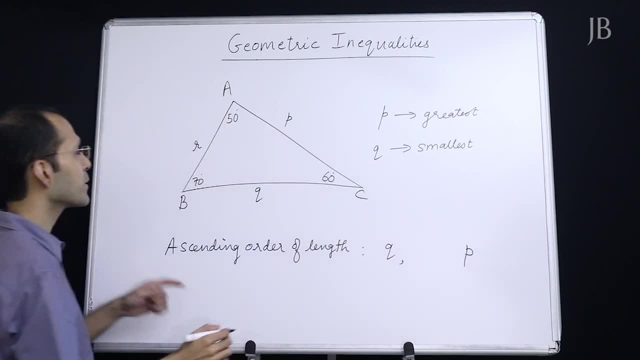 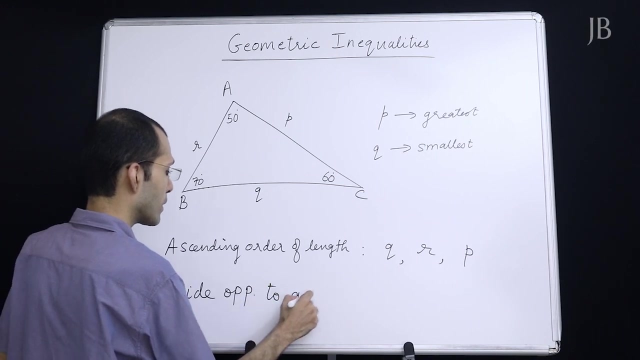 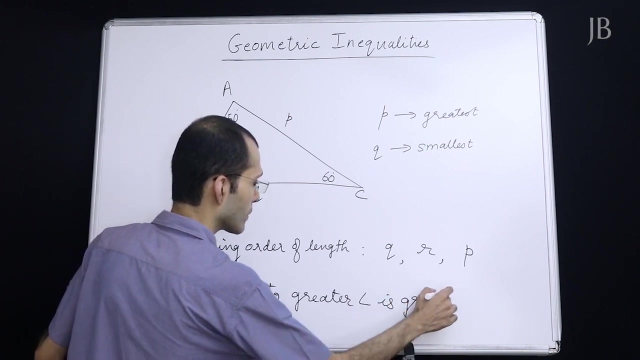 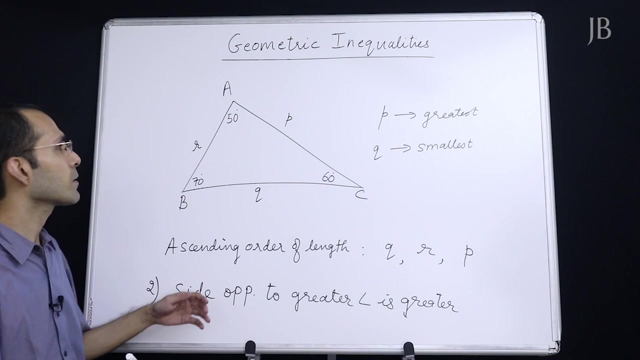 highest is what P. So what will come in between Q? Got this, So this is called side opposite concept, number 2.. Side opposite to greater angle is greater. Side opposite to greater angle is greater. Fine, So this completes with your first two concepts. Okay, and now one more. 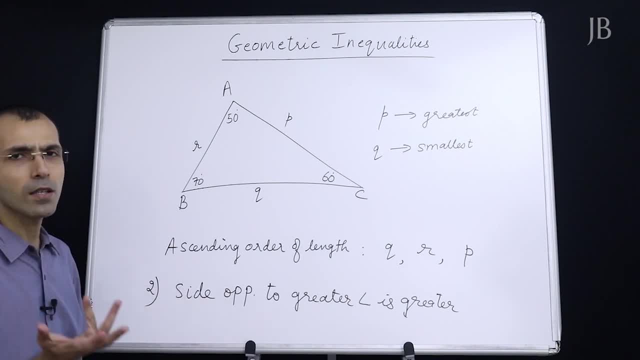 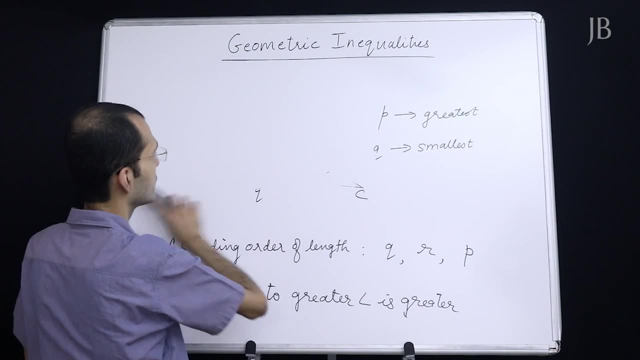 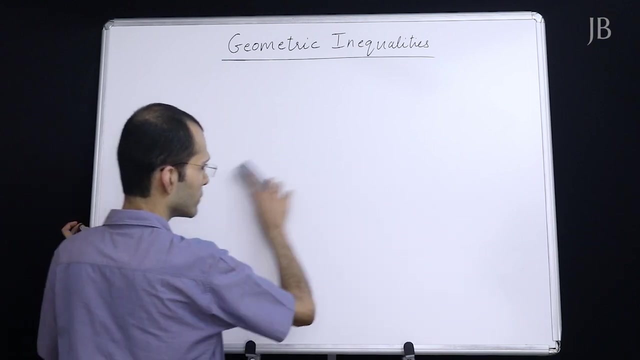 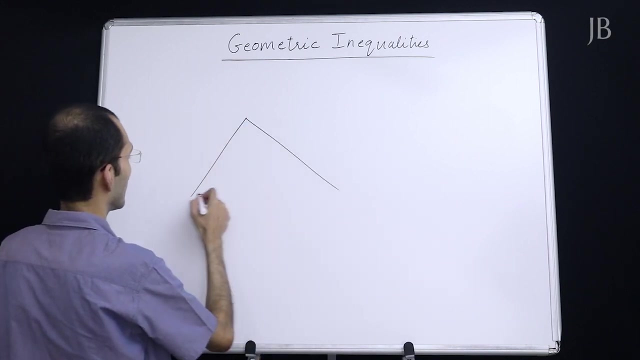 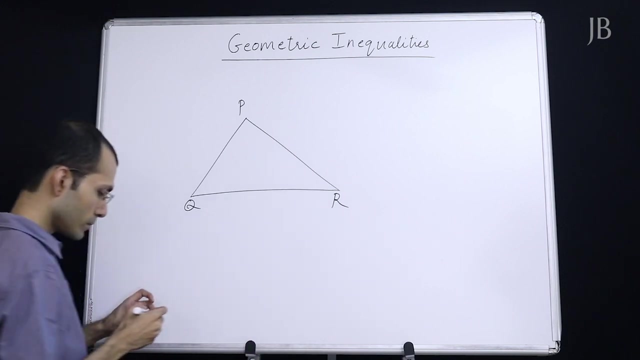 concept. and then we are done with the concepts and we'll take on some good writers and numericals. This is PQR, your triangle. Here for a triangle to exist in the very first place, sum of two sides of a triangle should always be greater than the third side, To be precise, sum of any. two sides of a triangle should always be greater than the third side. So what we're doing there is that- and these newspapers are coming out, Notice- simply two sides of a triangle go in either side, one hand, So 주는 the whole thing over your 1 side over the other. Such is the England's lei of laws, which includes De هlberg's law: elections. This is more than one in time. The second path, That's one in time, and too, we're not going to come back to that. This is 1 in time per classical algebra, since you cannot prove that, but only when you have testament space. This heights the א ende. 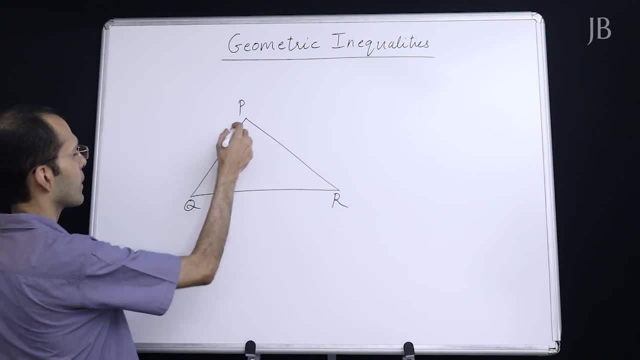 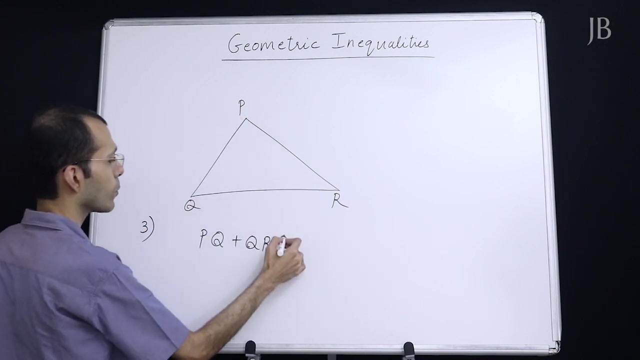 the third side. So if I mean some of any two sides, means we are talking about the length. So PQ, this is concept number 3. PQ plus QR should always be greater. You know the symbol: the open mouth. The open mouth stands for 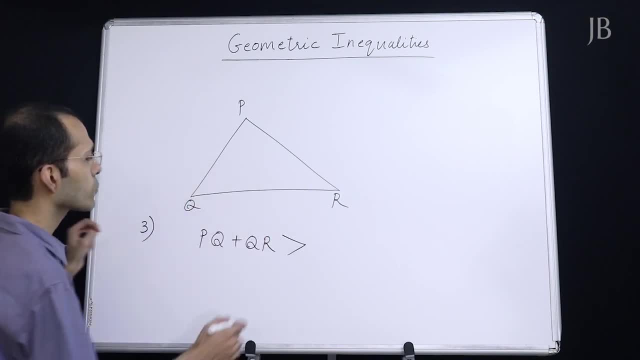 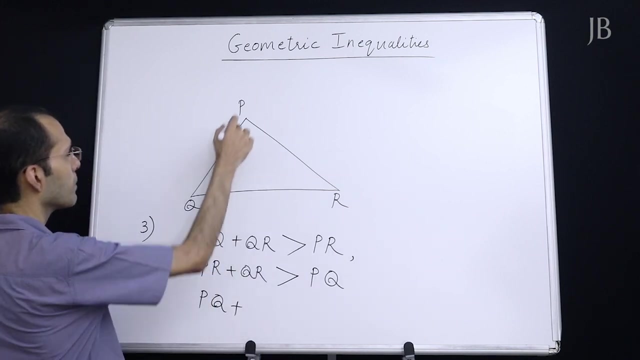 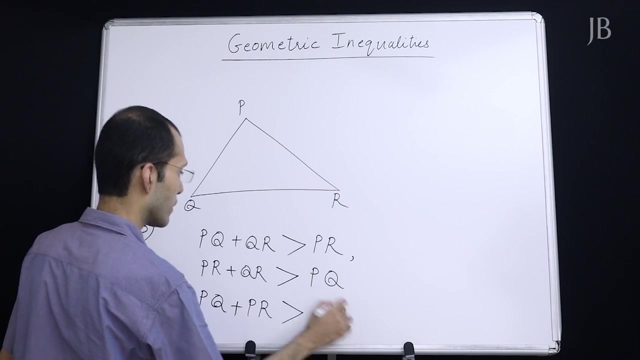 greater. So PQ plus QR should be greater than PR. Then any two sides you take PR plus QR. PR plus QR should always be greater than PQ. Then PQ, PQ plus PR should always be greater than QR, Otherwise the triangle will not exist. only So this concept is third. 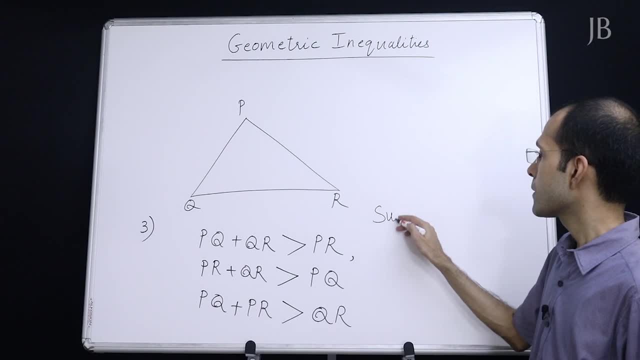 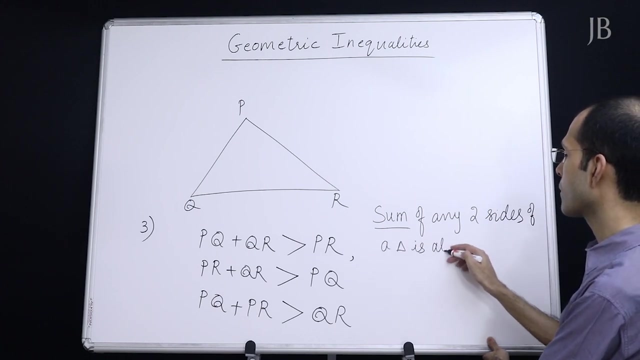 concept. It is formally written as sum of any two sides. sum. sum of any two sides of a triangle is always greater than the third side. it's always greater than the third side. Sum of any two sides of a triangle is always greater than the third side. 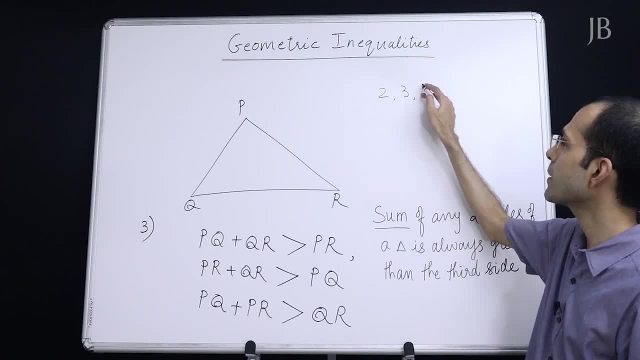 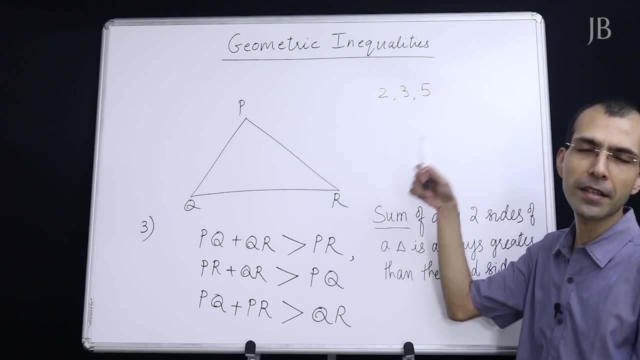 So if you have, if somebody tells you, can you have a triangle, can you have a scale in triangle whose sides are 2 centimeter, 3 centimeter and 5 centimeter? Can such a triangle exist real life? No See, let's assume such a triangle exists for some time. Okay with. 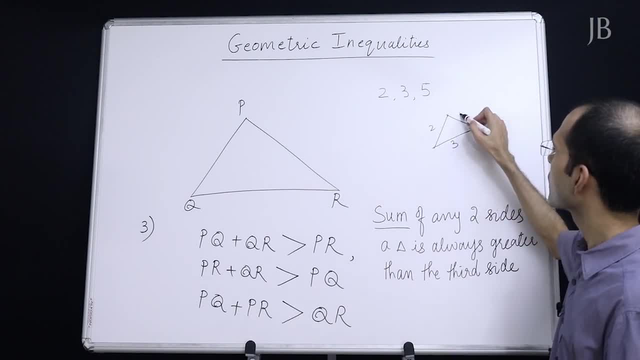 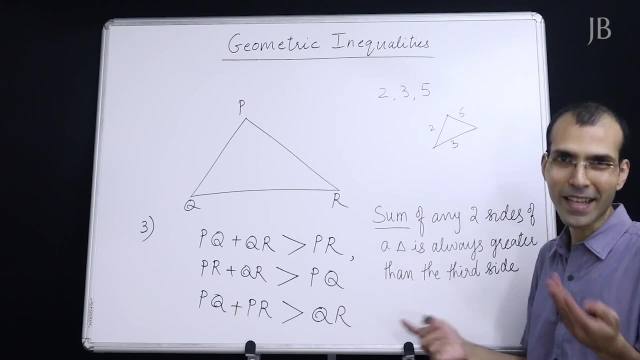 2,, 3 and 5, a scale in triangle. Now let us see whether it satisfies this condition. For a triangle to exist, some of its two sides, the lengths we are talking about, should always be greater than the third. Now, 5 plus 3, 8.. 8 is 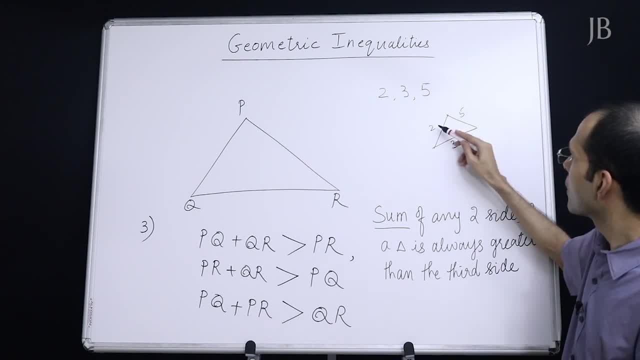 greater than 2.. Okay, good, 2 plus 5, 7.. 7 is greater than 3.. Good, 3 plus 2,. 3 plus 2, 5.. And this is coming equal to 5.. So this one condition is getting violated, So 3: 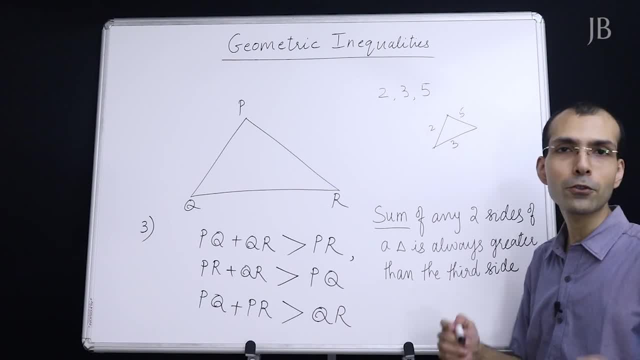 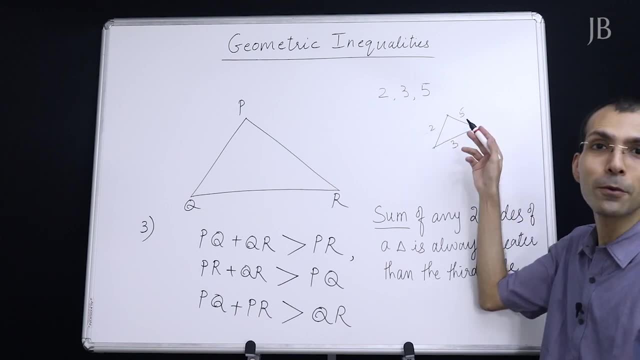 plus, because sum of any two sides of a triangle should always be greater than the third side. So now what happens? 3 plus 2 is 5.. 5 and 5, they are equal. So no, such a triangle cannot exist, If you. 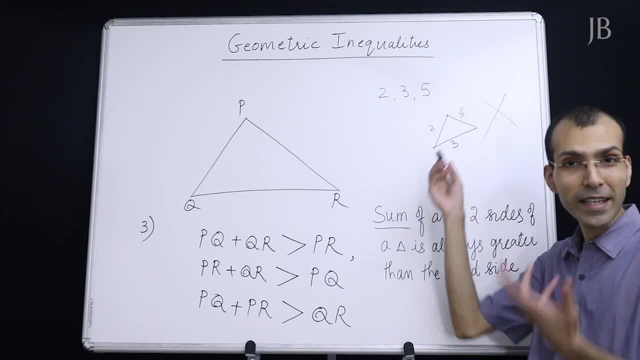 forcibly. try to find the area of such a triangle using your other knowledge of geometry. like Heron's formula, the area will turn out to be 0, indicating that the triangle cannot exist. Because how can the area of a triangle be 0? Some. 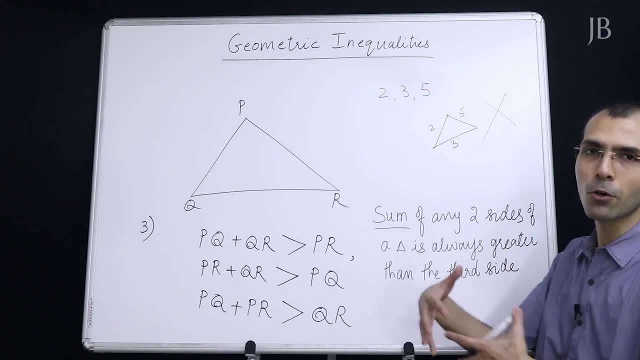 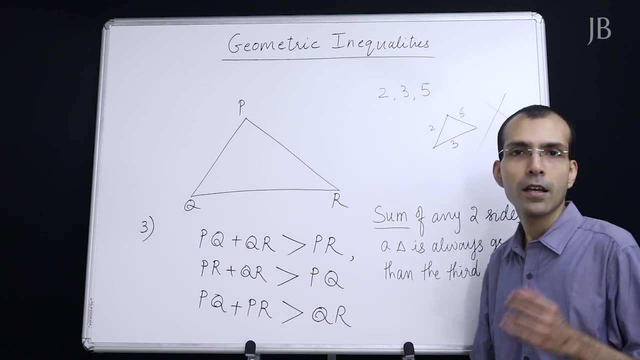 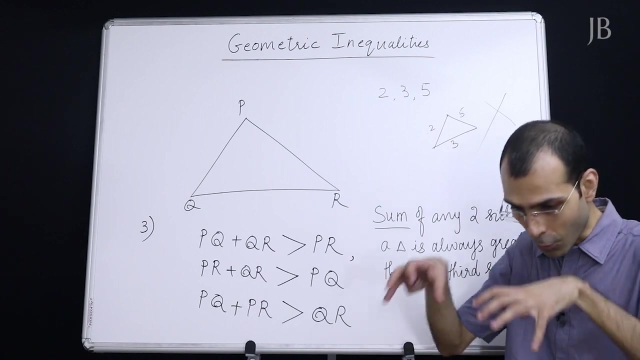 area, it will have right. So this is what you know. anywhere you go, things will match. So third concept is also now done. So keep in mind: angle opposite, angle opposite to greater side is greater. This happens for one particular triangle. You cannot. 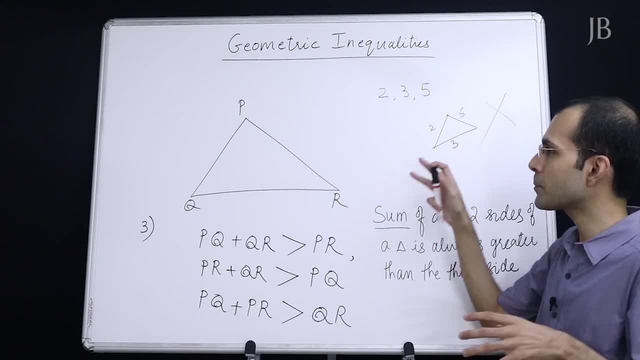 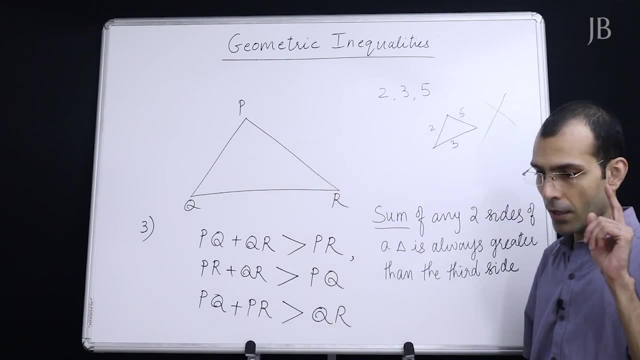 compare two different triangles like that, All these properties are valid for a particular triangle. So sum of any two wait angle opposite to greater side is greater. Then side opposite to greater angle is greater. And third, sum of any two sides of a triangle is always greater than the third side. So we saw here concept number. 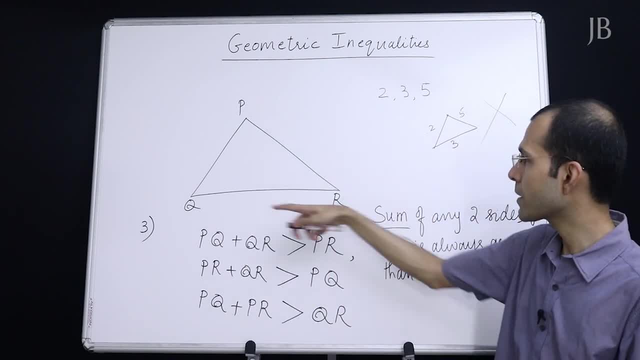 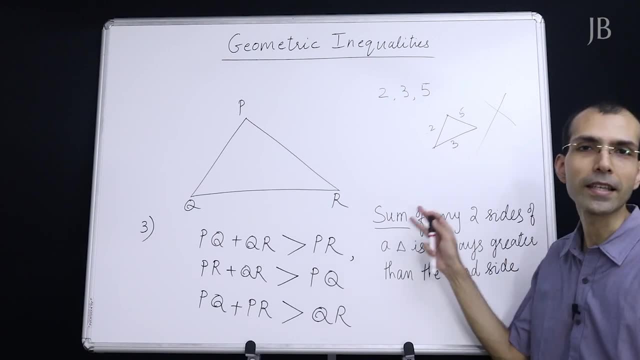 3, PQ plus QR is greater than PR. PR plus QR is greater than PQ, Then PQ plus PR is greater than QR, And this we have written it formally. So what I suggest is you first take down these three concepts from the board by pausing the. 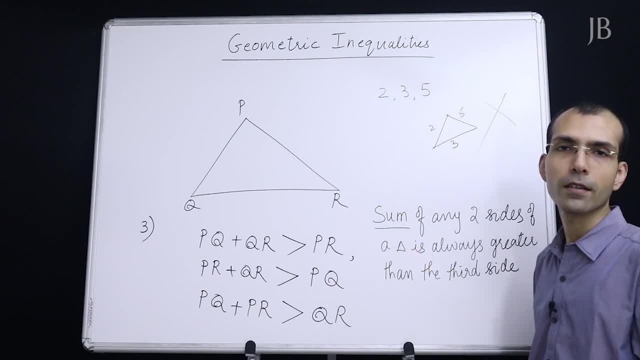 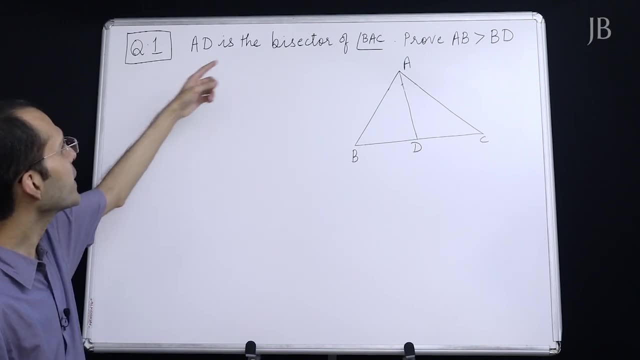 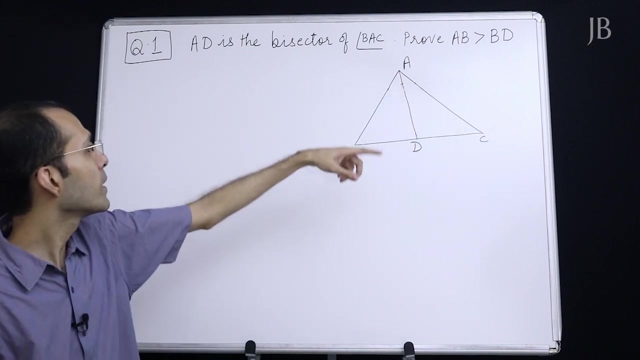 video, as per your comfort, before we take on to the numericals. Question 1. AD is the bisector of angle BAC Prove AB greater than BD. Now see here whatever three concepts you have studied. they are of course very important, but 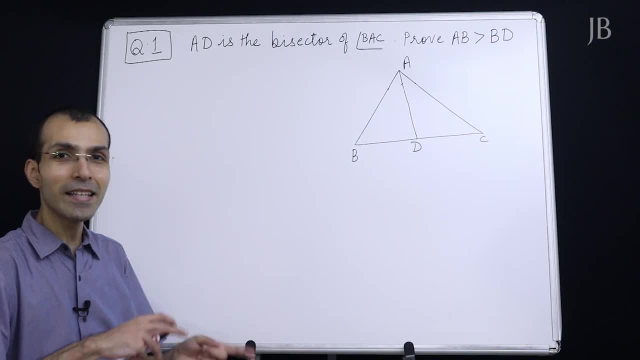 over and above. you will have to know the basic geometry concepts like linear, linear, pair. sum of the angles of a triangle is 180, then vertically opposite angles are equal. if lines are parallel, then alternate angles are equal, corresponding angles are equal, co-interior angles are supplementary, and so on. 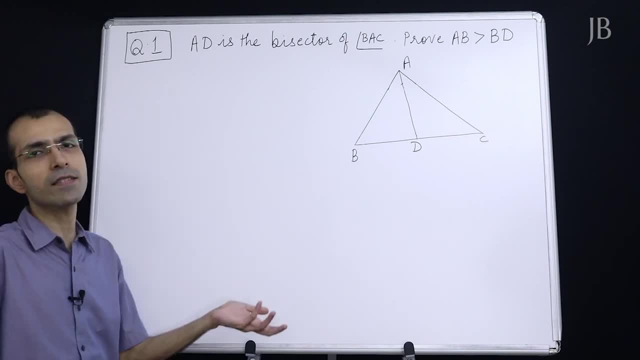 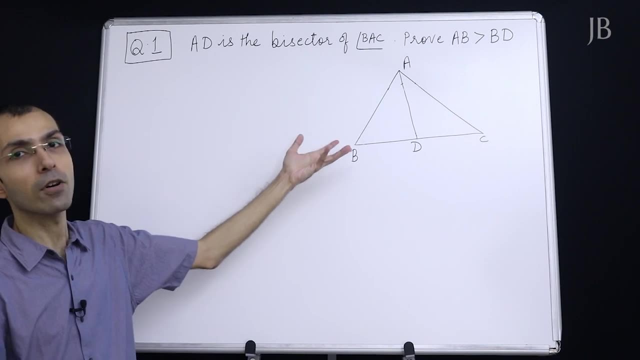 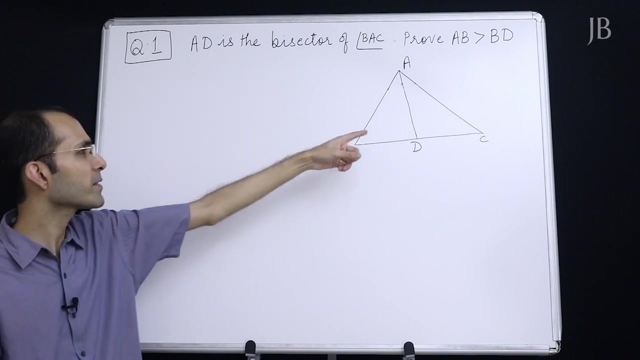 The knowledge of that is also essential, and in very advanced sums. knowledge of congruency is also essential, congruency blended with inequalities. This seems to be a fairly simple sum: small information and just two small triangles and one big triangle. This is simplest what can exist, I feel. 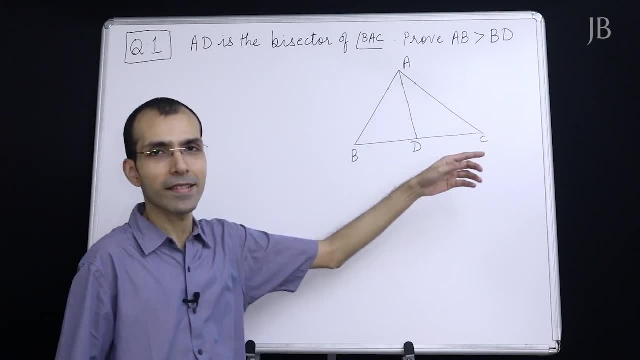 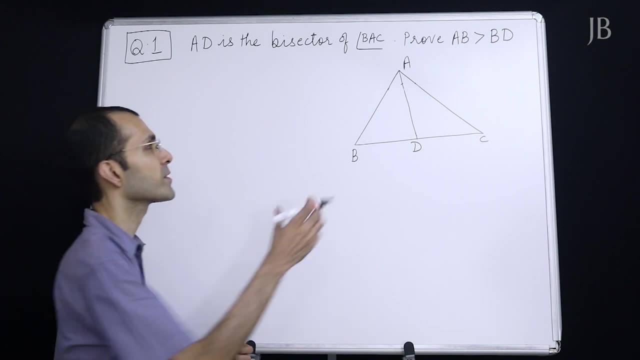 AD is the bisector of angle BSE, So AD is the bisector of angle BSE. Bisector means it divides the angle into two equal halves. So this is the angle BSE and AD is the bisector, So this angle will be x. 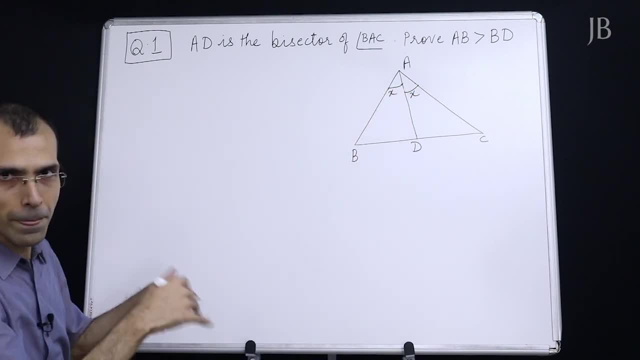 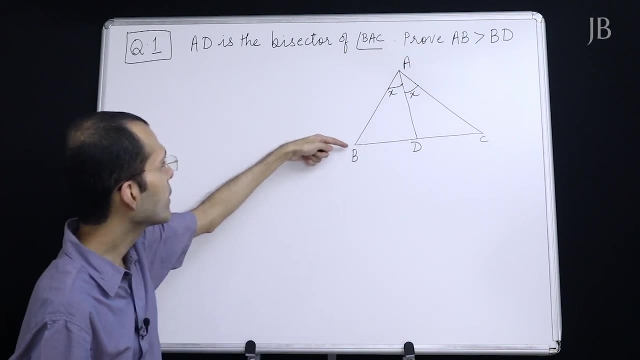 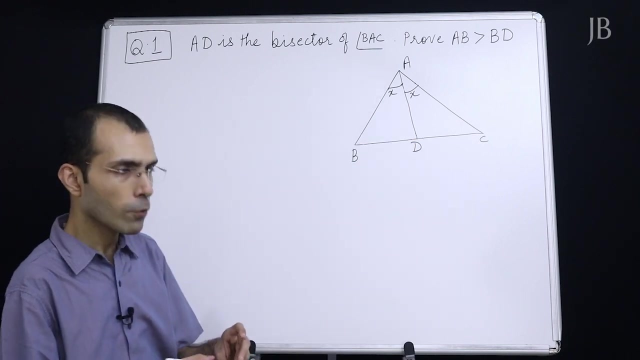 This angle also will be x. Use this x technique and all it helps you to make this sum easy. Prove that AB is greater than BD. Prove AB is greater than BD. Prove AB greater than BD means we have to prove that length of segment AB is greater. 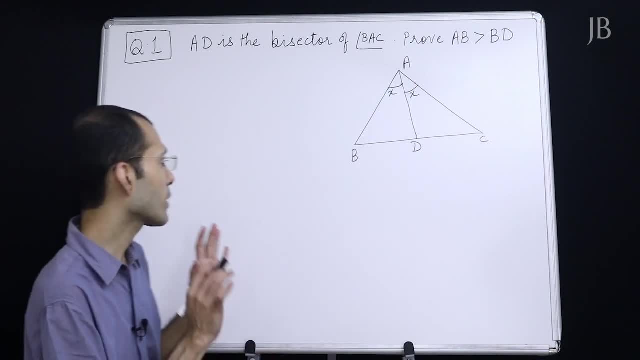 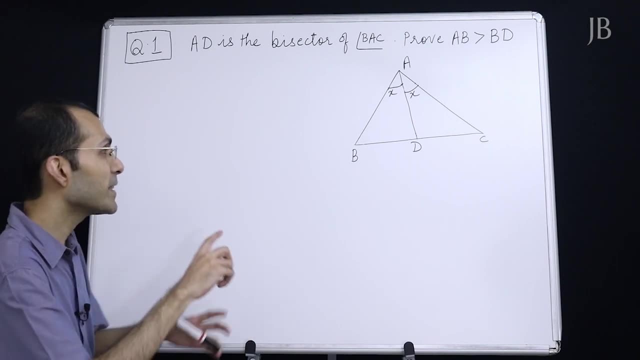 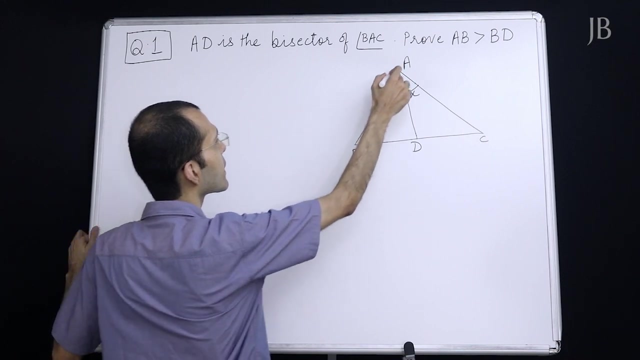 than length of segment BD. that's understood. Recall your concept. If one side is greater than the other, Then the angle opposite to that also will be greater. So if I have to prove AB greater than BD, I should catch hold of the angles which are: 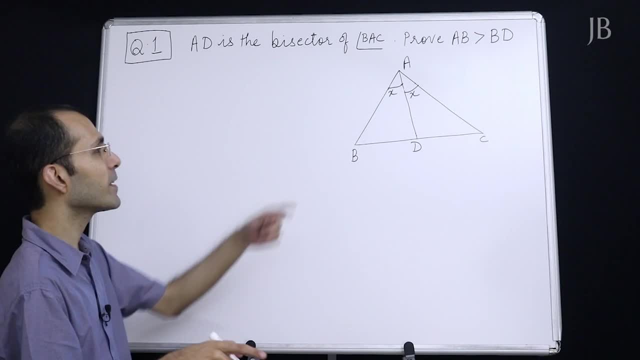 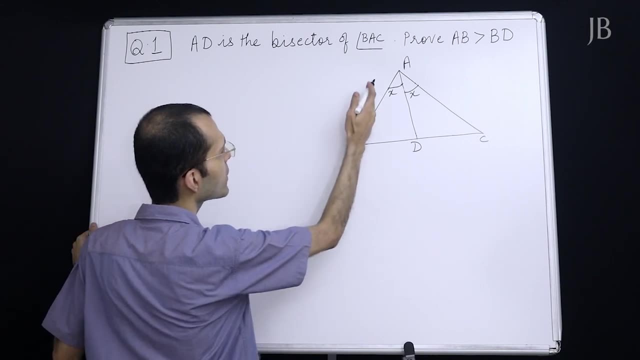 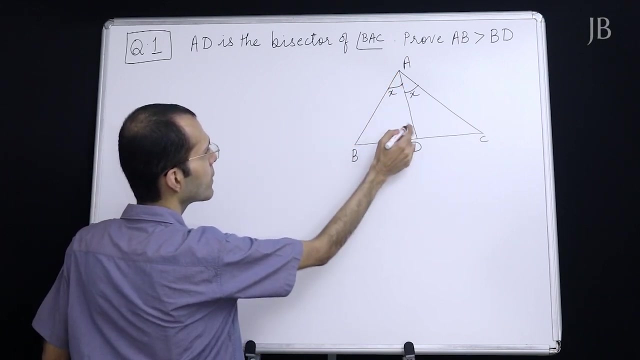 opposite to them and play with the angles and then this conclusion will automatically follow. So this is AB, which is the angle opposite to AB. Consider this triangle ADB. So this is AB. This is ADB. This is segment AB, Which is the angle opposite to AB. 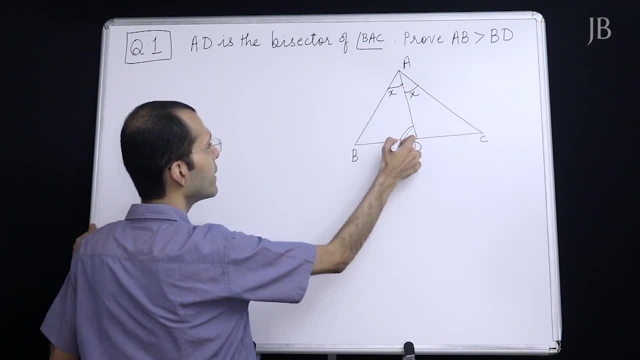 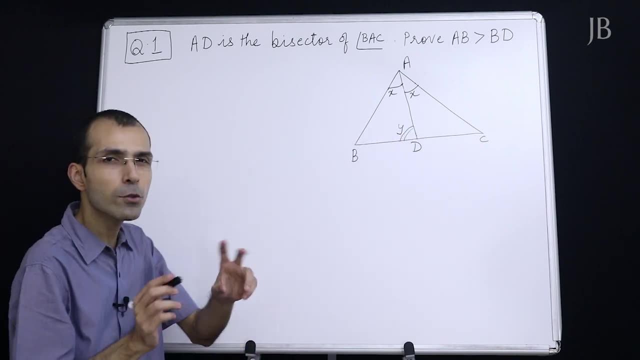 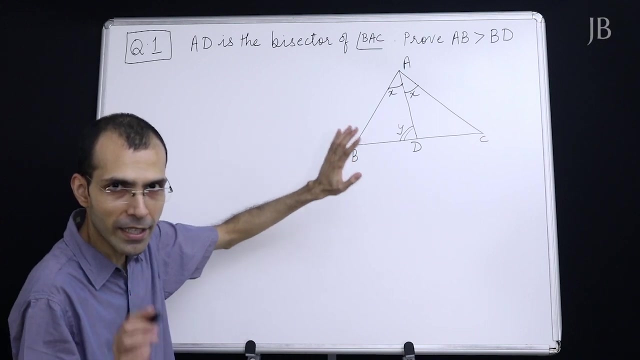 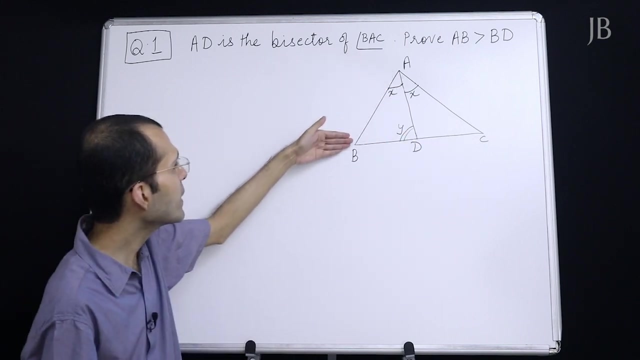 This angle Angle, ADB Agreed, So we call this as Y. We have to get a relation between which two sides, AB and BD. We have to get a relation between AB and BD. To be precise, we have to prove that AB is greater. 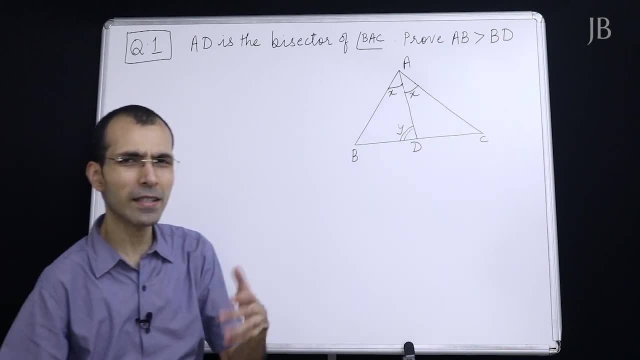 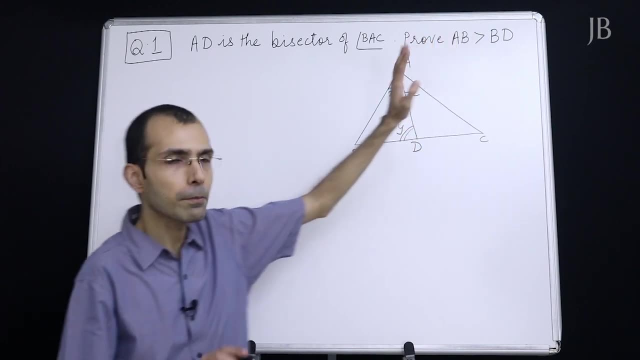 Open mouth means greater, The symbols we have studied in class 6 and 7, the crocodile mouth. So open mouth means greater. So prove AB greater than BD. So this is AB and this is BD, Which is the angle opposite to AB. 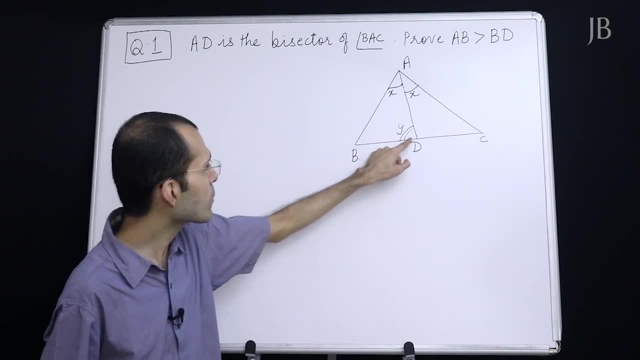 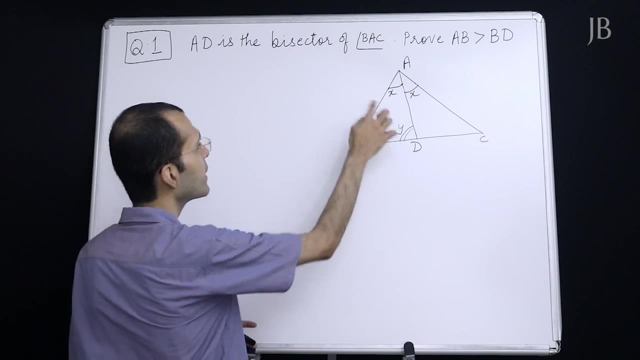 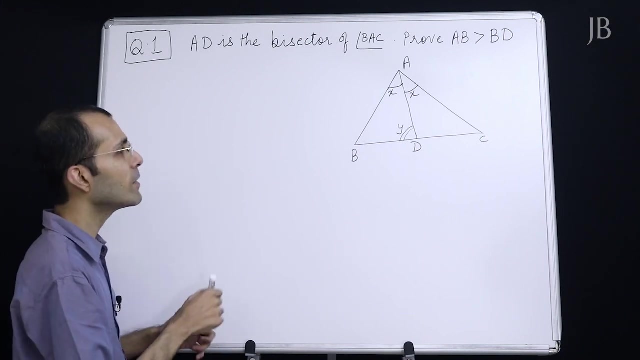 Y, We have marked it, Which is the angle opposite to BD X, Already marked. Now we want to prove AB greater than BD, So in this case we have to. So in other words, what we have to prove, We will have to prove y greater than x. We. 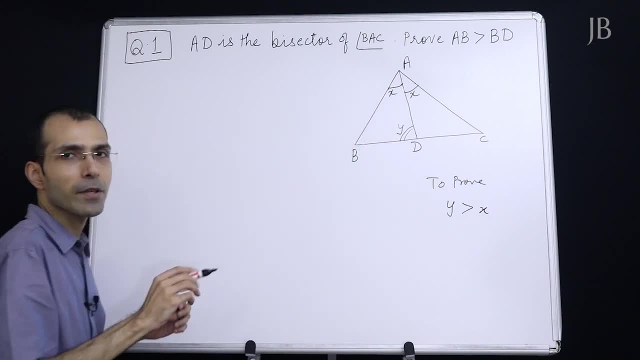 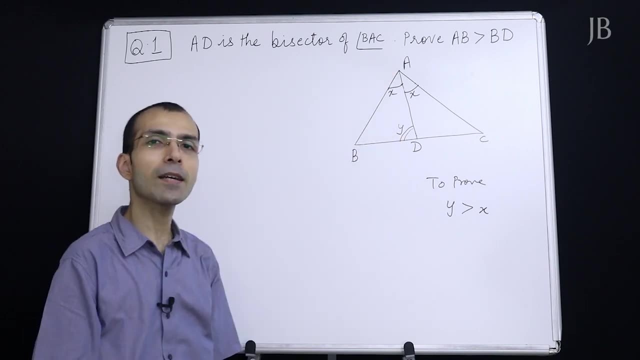 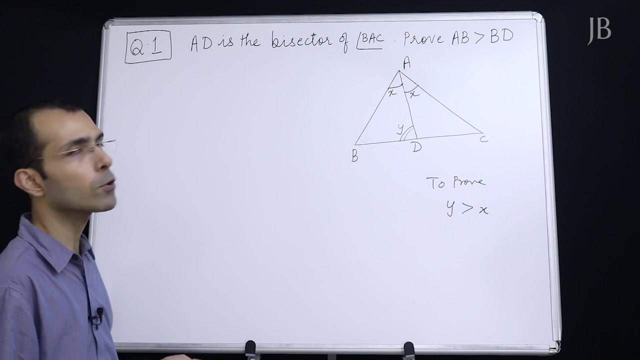 will have to prove this angle greater than this x, Because if we can prove this angle greater than this angle, the side opposite to this angle will automatically become greater. So the problem boils down to proving y greater than x. Now how to prove it? Very simple. 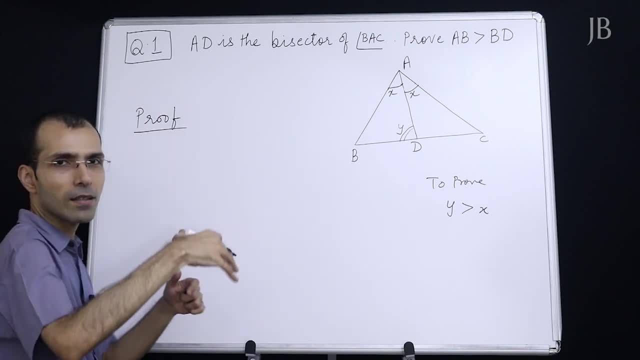 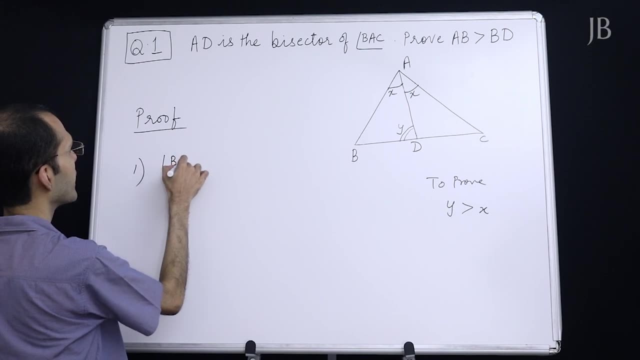 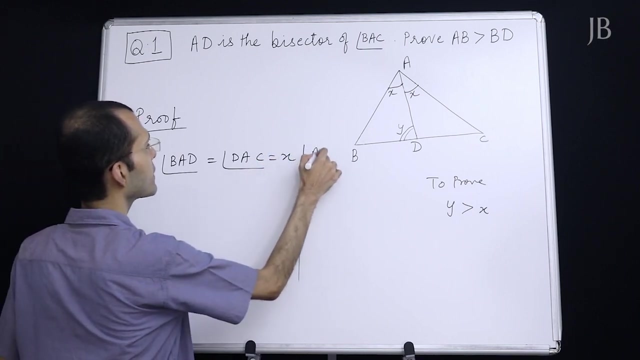 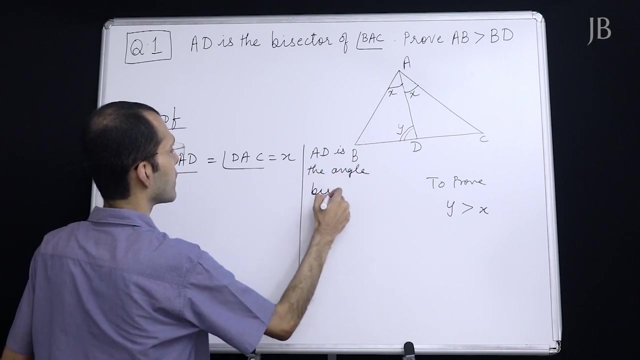 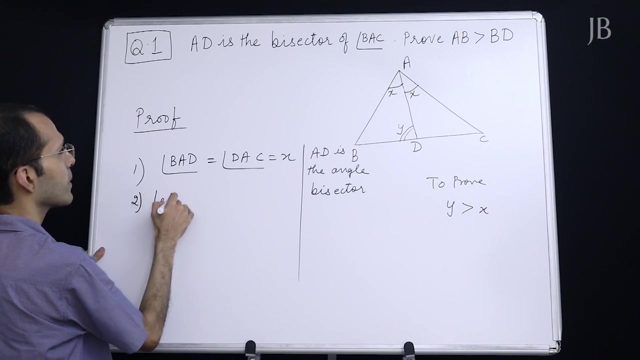 So little analysis is required and this is a little different from your other conventional geometry topics. We will write here: angle BAD equaling angle DAC equaling x. The reason is: AD equaling x. AD is the angle bisector. AD is the angle bisector. Fine, Then let angle AD be y Assumption: 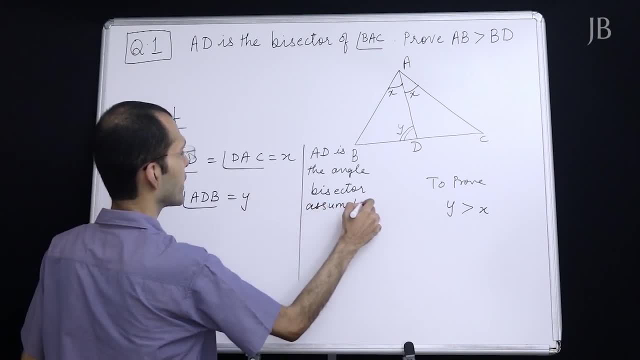 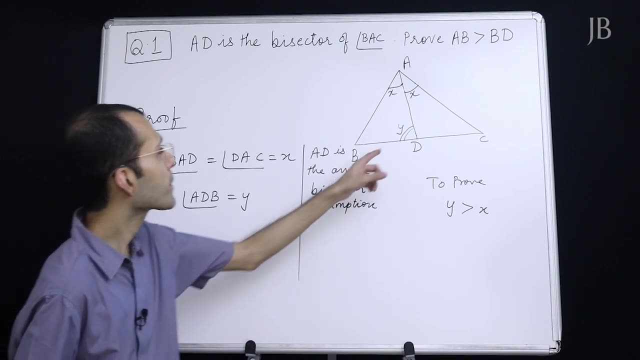 No, we cannot take it as x, We can take it as y. some other thing Is nature, some other thing- Y, so to speak- is a natural Gymorphism. So they think we cannot create a triangle. it is a particular form of triangle, But it cannot be just the angle. 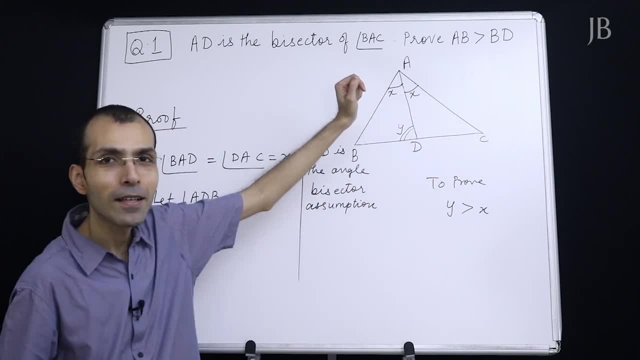 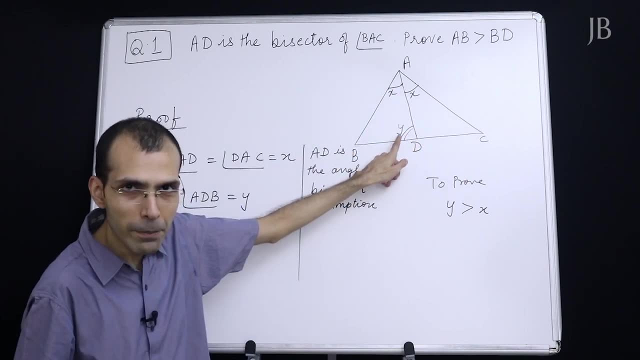 that we see on the paper. Wait, If you observe triangle ADC, look at triangle ADC. Can't I say that this y behaves like the exterior angle, Because this is the interior angle. This will become the exterior angle. Interior plus exterior should give you a straight line. 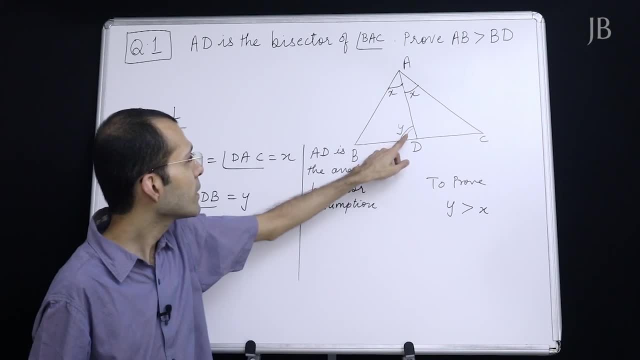 If you look at triangle ADC, if you look at triangle ADC, this y becomes your Y. For you, this y will become a natural key Because initially, since you began to show yourself as an imaginary vector, you use the Persian letter king, powerfulriers, hyper. 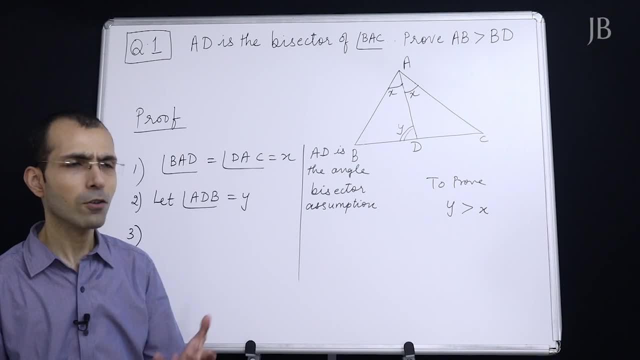 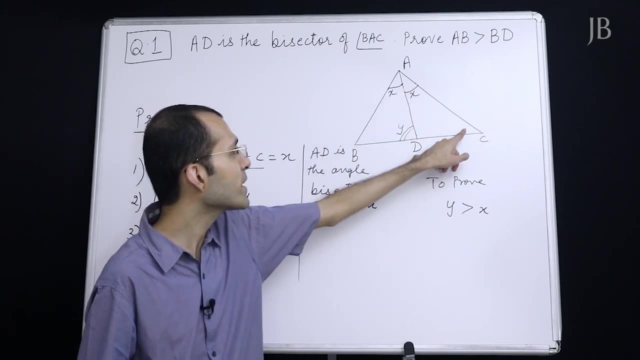 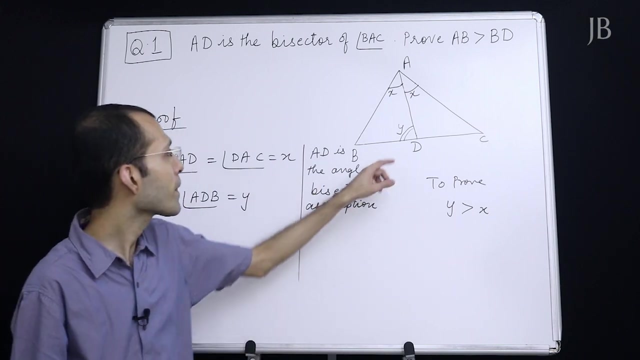 exterior angle and what is the concept for exterior angle? Exterior angle is equaling sum of opposite interior angles. In case you do not know this concept, please revise this concept first and then correlate here. Exterior angle is equaling sum of opposite interior angles. 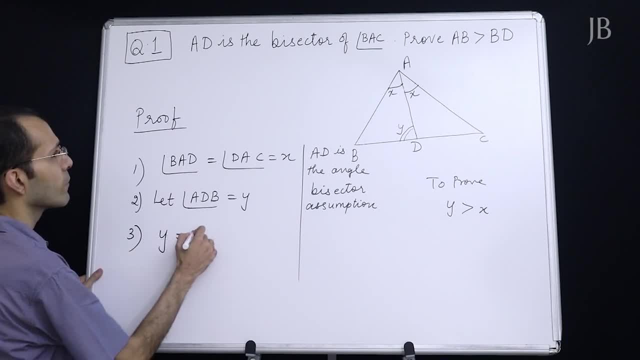 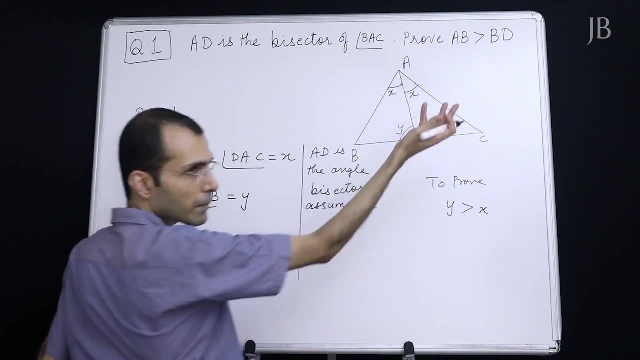 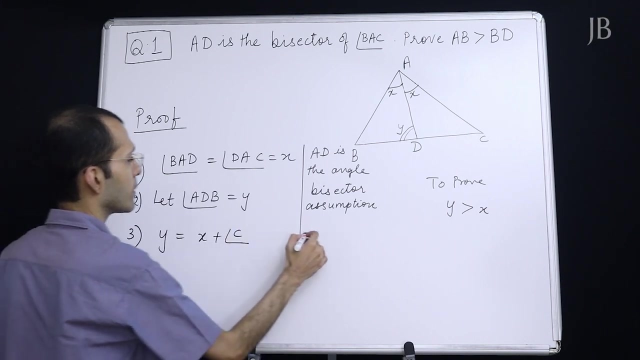 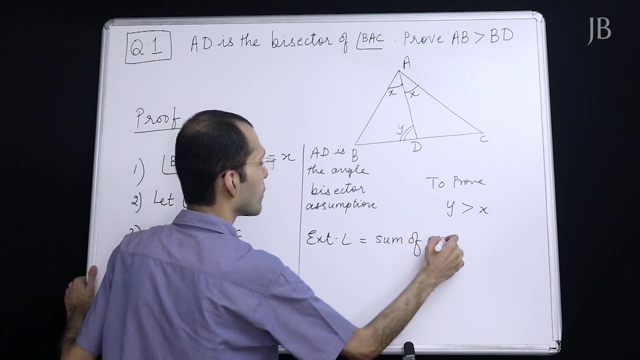 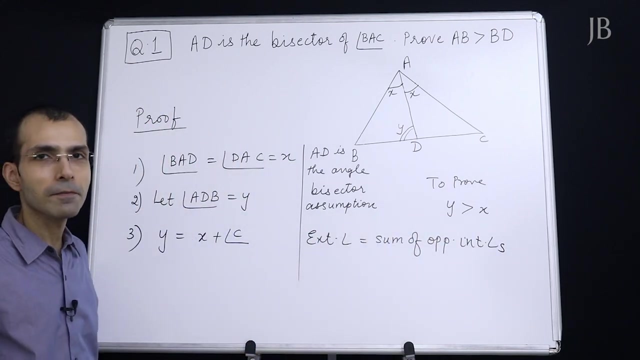 So I can say that y will be x, this x, and both of them are x only, but we are referring here. y is equaling x plus angle c. This is called exterior angle is equaling sum of opposite interior angles. And we are done. Have you realized The sum? 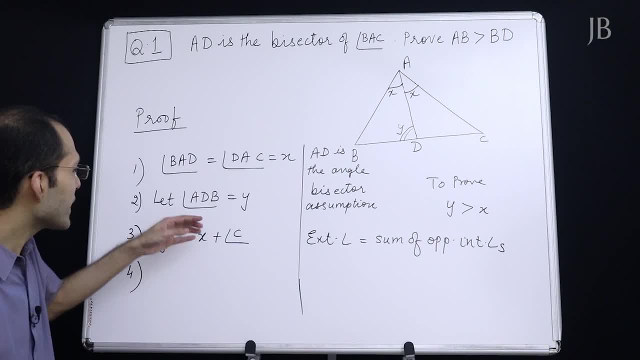 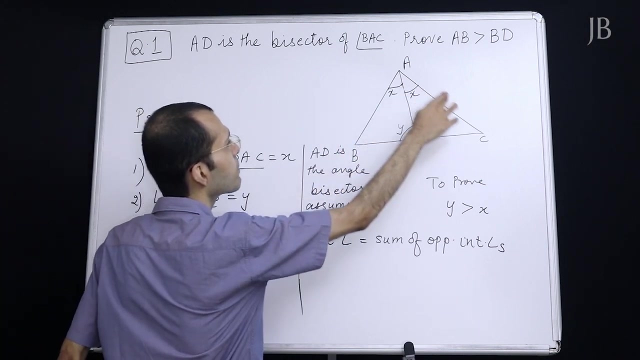 has come to an end. y is equaling x plus angle c. Whatever be the value of angle c, y will always be greater than x now Because y exterior angle- is equaling x plus angle c. So whatever is the value of x, 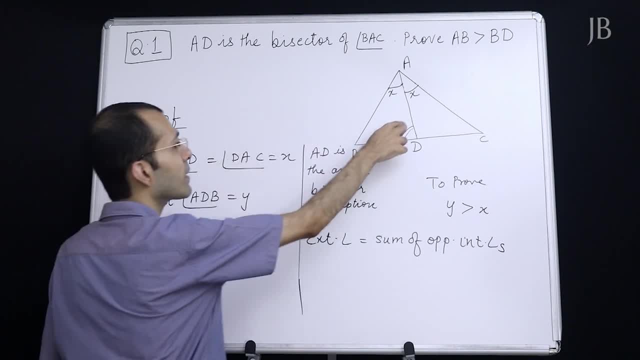 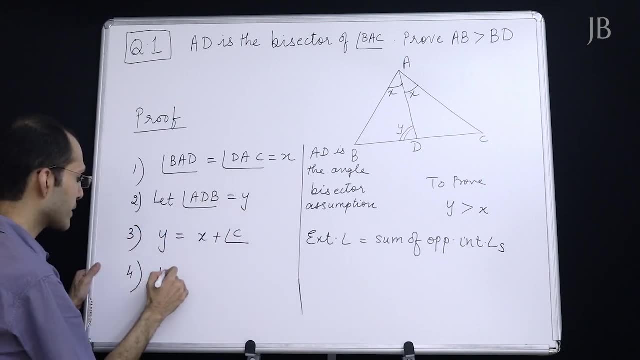 add the value of c to it, Then angle y will come. So y is equaling x plus c. So this implies y is clearly greater than x, Because x is x and y is x plus c. So this extra happens. So this clearly implies: 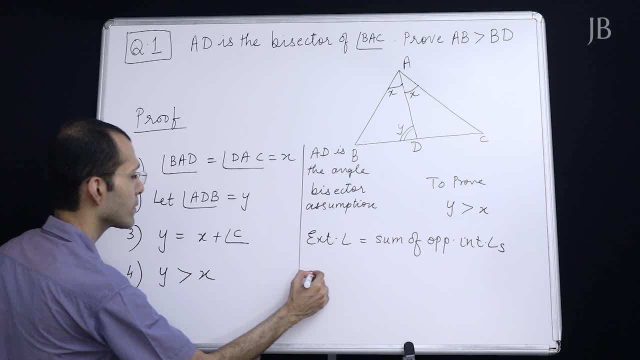 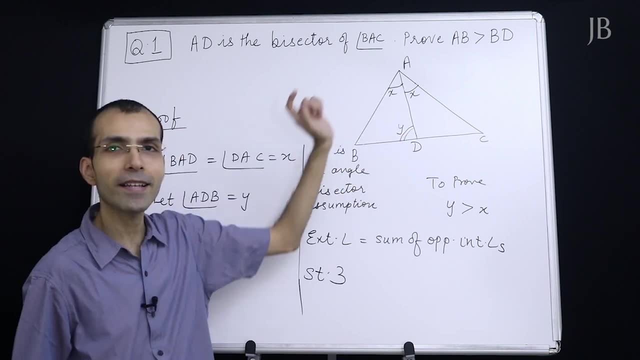 y is greater than x. How do we infer this From statement 3.. And that is what we had to prove. Now, we have proved that y is greater than x. Now, whether I take this x or this x, no harm, because both. 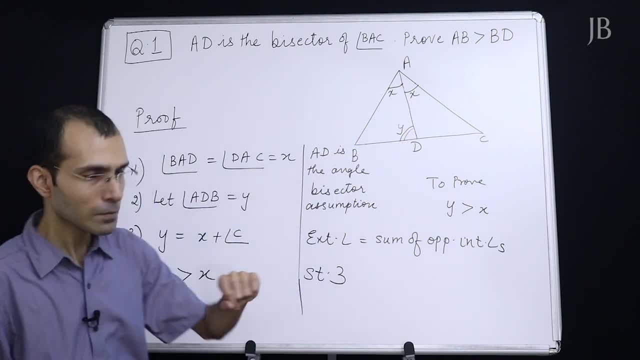 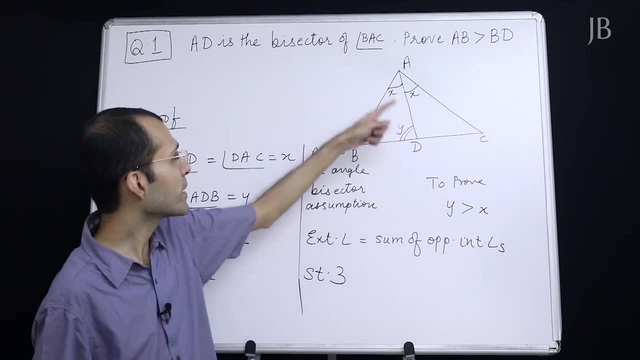 the x's are the same, so we can take advantage of it. So, while applying exterior angle property, we considered this x. We said y is equaling x plus c. But this is also x, only That means now y is greater than x. What is opposite to y? 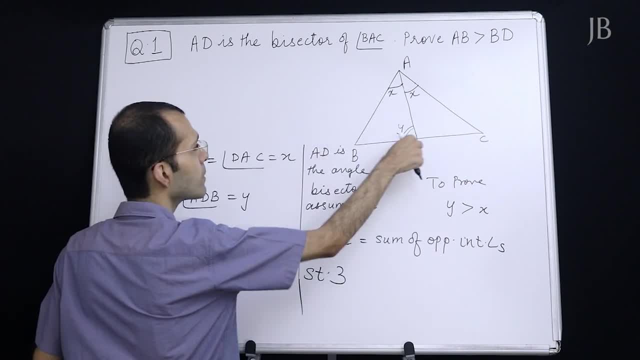 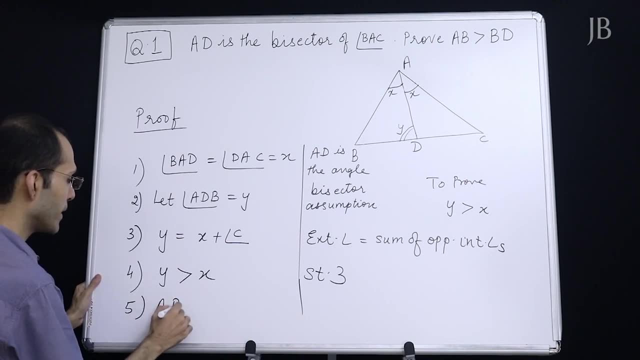 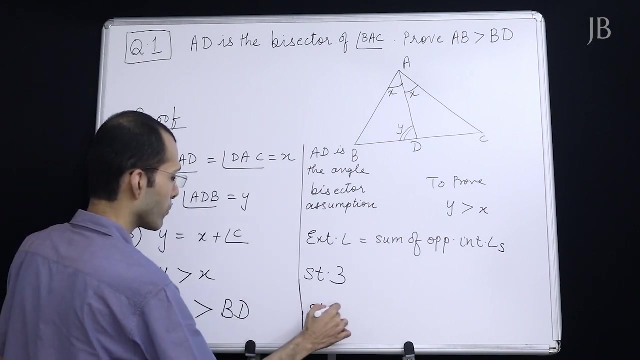 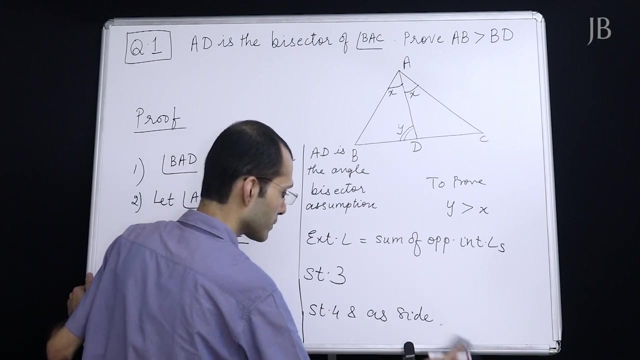 a, b. What is opposite to x, b, d. Who is greater? We just now proved y is greater. So this will imply a b greater than b d And the reason will be statement 4. and as sides side opposite, side opposite to greater angle. 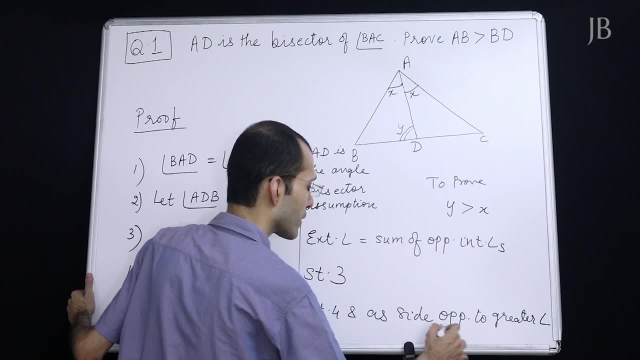 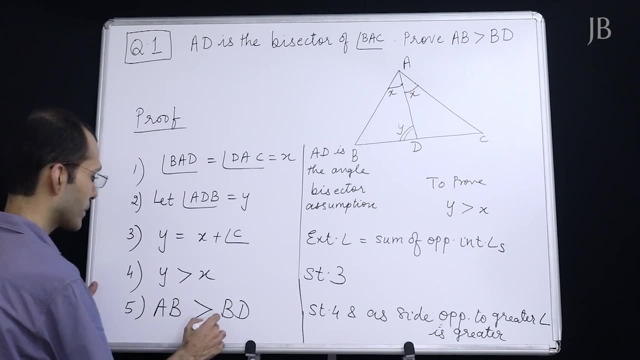 is greater. Got it, So proved, Hence proved. It takes a lot of time to explain and understand for the first time, but otherwise this can be done under a minute actually. Fine, so we have done with question 1.. Question 2.. 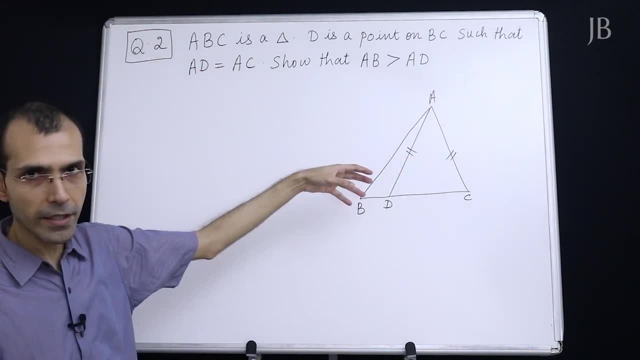 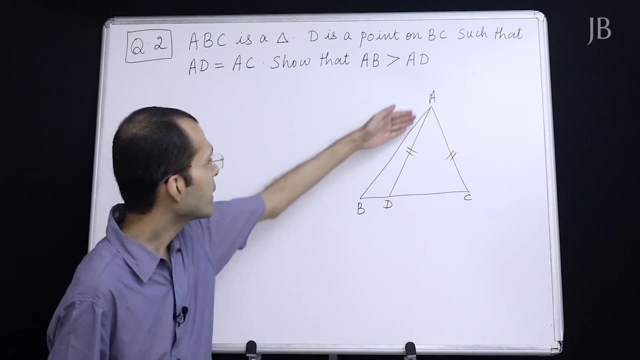 a, b c is a triangle. The diagram is already drawn and given to you. d is a point on b c, such that a d equaling a c. d is a point on b c, such that a d. 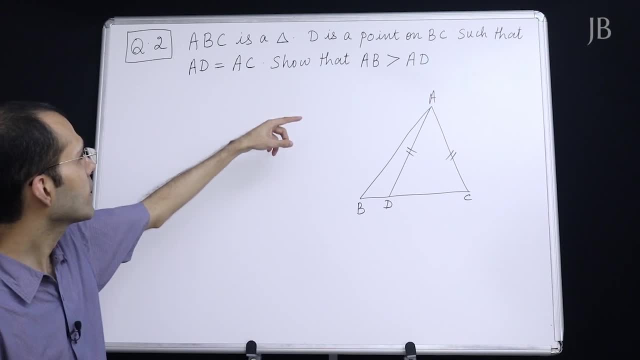 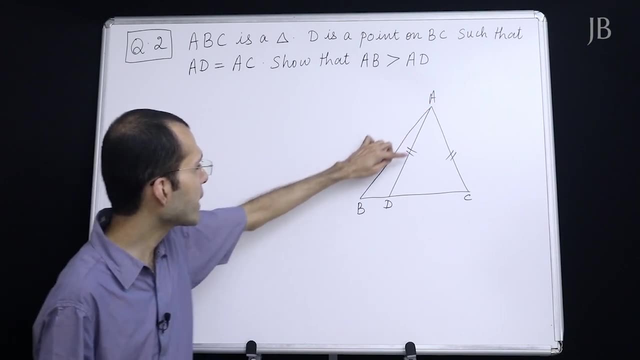 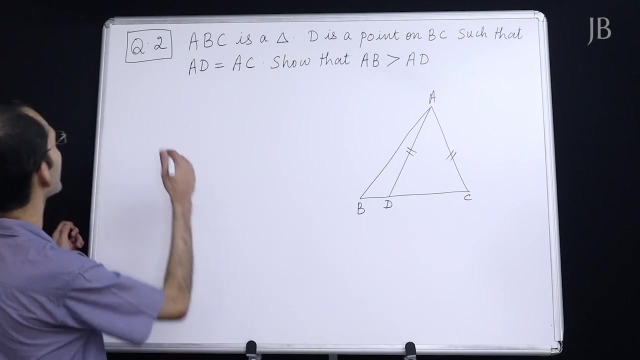 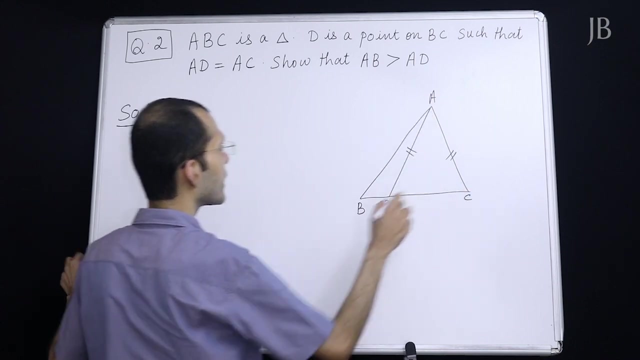 equaling a c. Okay, To show that a b greater than a d, a b greater than a d. This is what we have to prove. Fine, How do we go about Now? here? a d and a c are given to be equal, So. 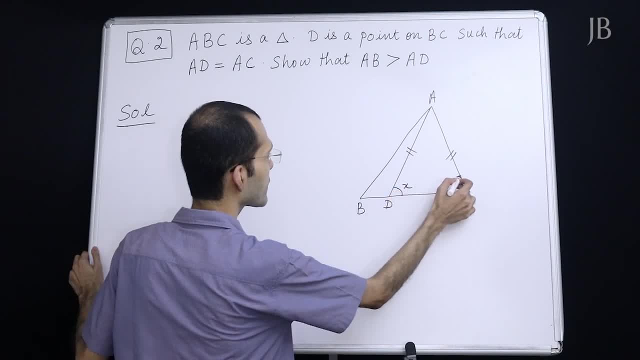 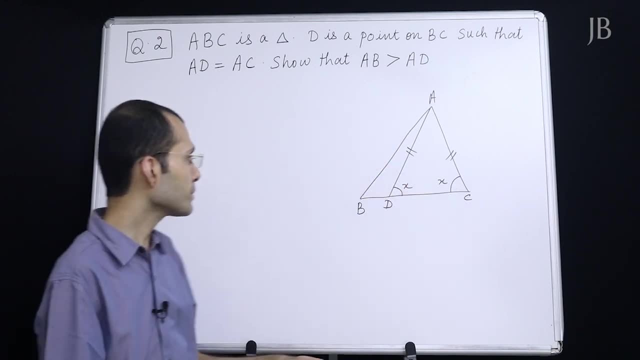 let. so angles opposite to them also will be equal. You know simple isosceles triangle concept. So let the two angles be x and x, because the two sides are equal. Now what we have to prove: a b greater than b d. So we have to prove that. 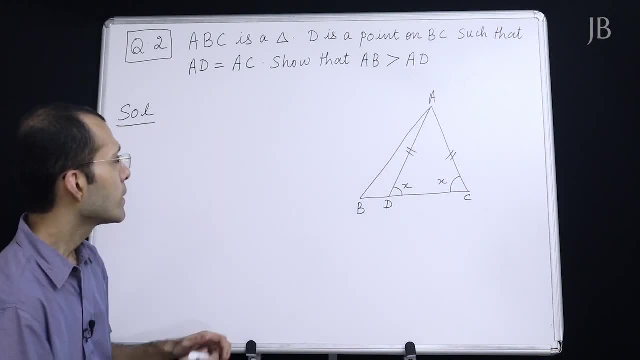 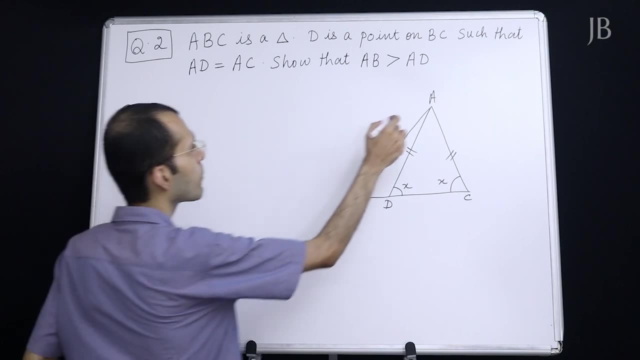 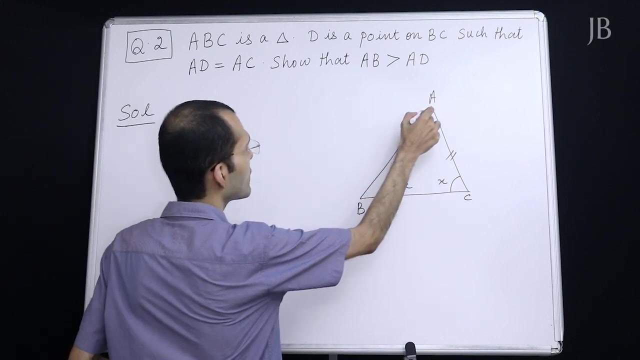 ab, c is a point on a, d. So what will we do? We try to- we proved this in directly- We try to catch hold of the angle which is opposite to ab. So, But then you have to consider one triangle at a time. Now this is a- b. So if I take triangle a, d, b, 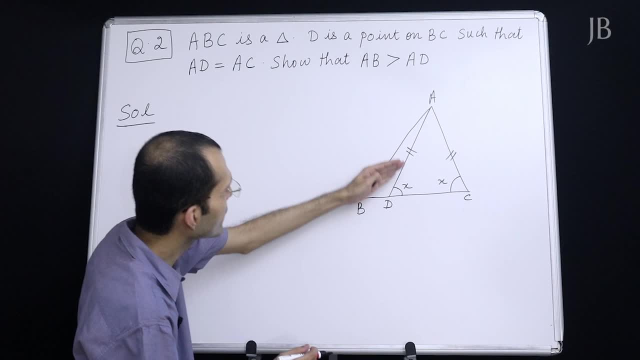 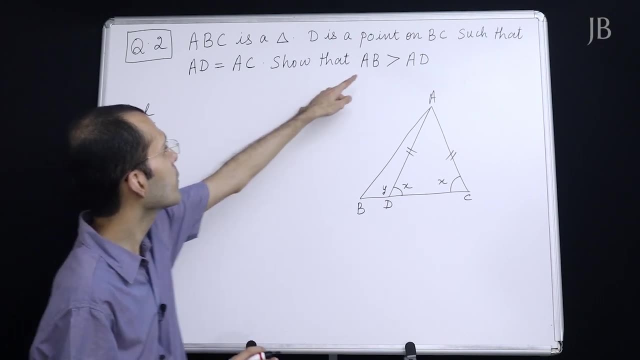 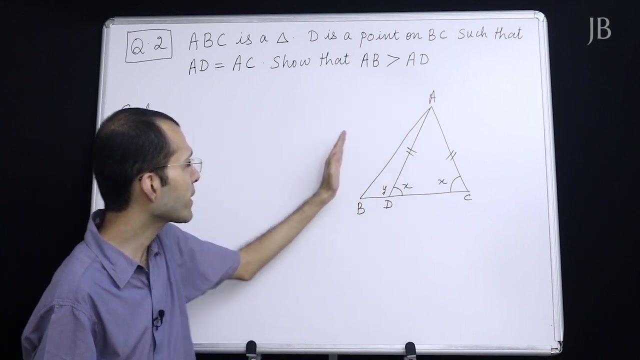 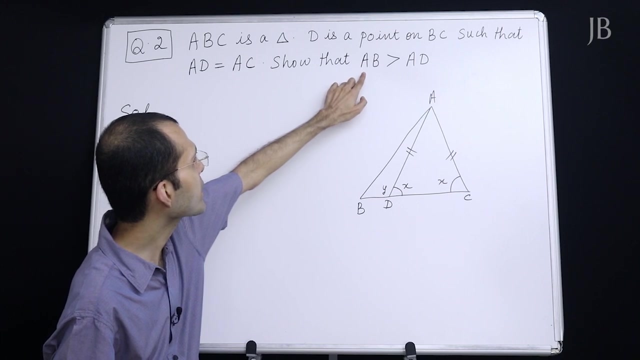 opposite a b, Opposite a, b. which angle will come? This one y Okay, And we want to prove it is greater than AD. This is AD. Abhi, AD ke opposite, kaunsa angle ata hai? Focus your eyes on triangle ADB. So I want a relation. 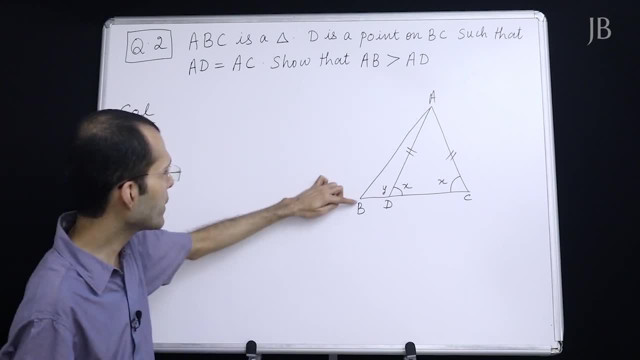 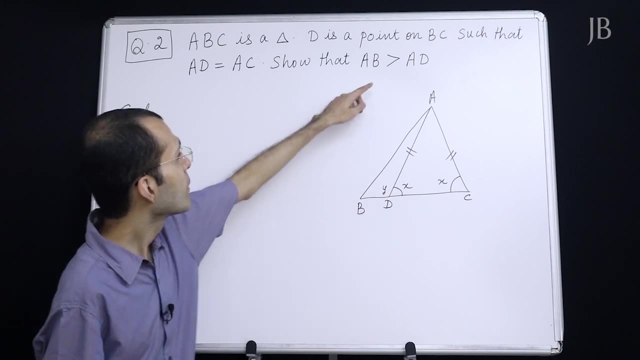 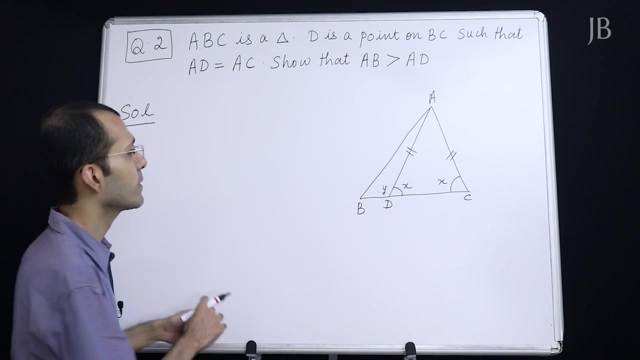 between AB and AD. So AB ke opposite kaunsa angle ata hai Y. We marked it. We can't take X because X is already used here. We want it to be proved greater than AD. This is AD. So opposite AD, kaunsa angle ata hai This one, That is Z. Now, if I want to prove, 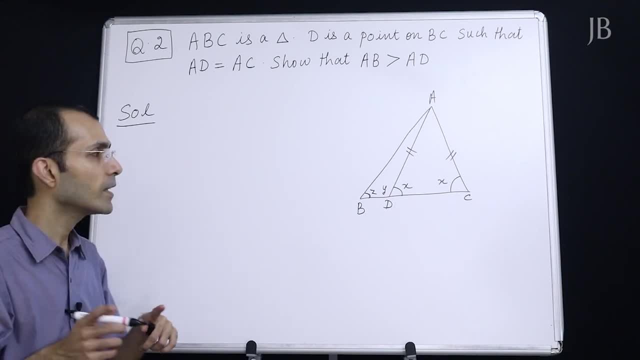 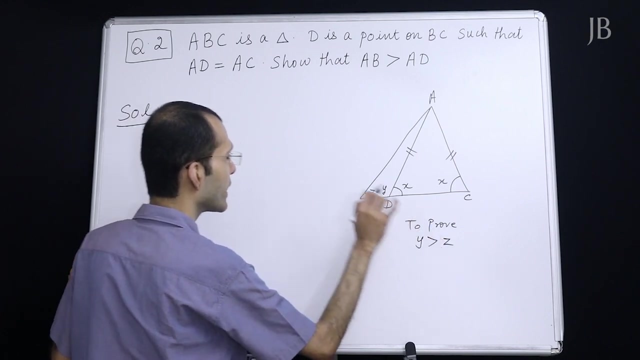 AB greater than AD segment. in other words, I will have to prove that the angle opposite to them are greater. So AB ke opposite angle, ad ang, is y and AD ke opposite angle is Z. So in other words, I have to prove y greater. 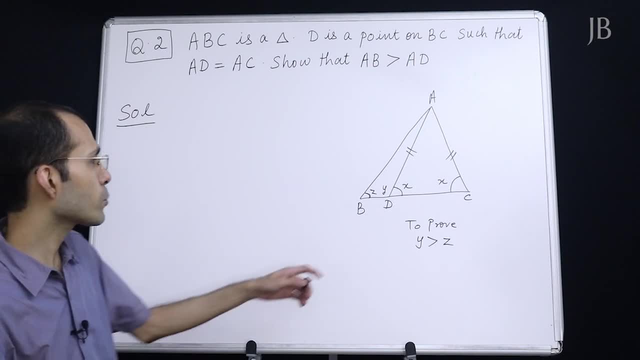 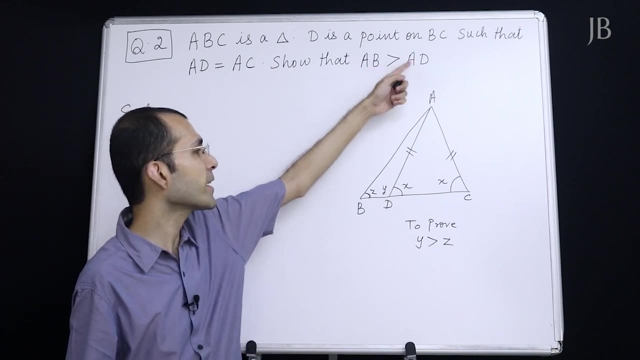 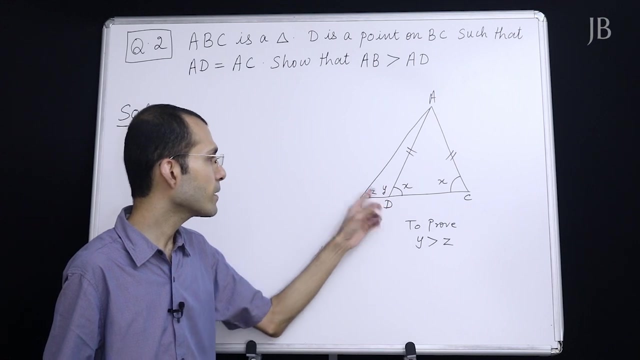 than Z. If we can manage to prove y greater than z, then we can easily say that AB will be greater than AD. Now question arises: how to we prove y greater than Z? Now see, to directly prove y greater than Z, we will have to use that boolean danger. 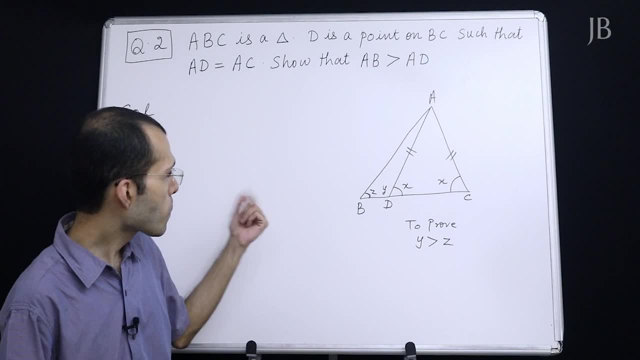 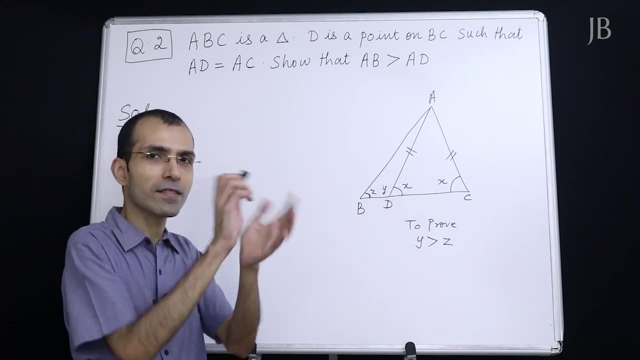 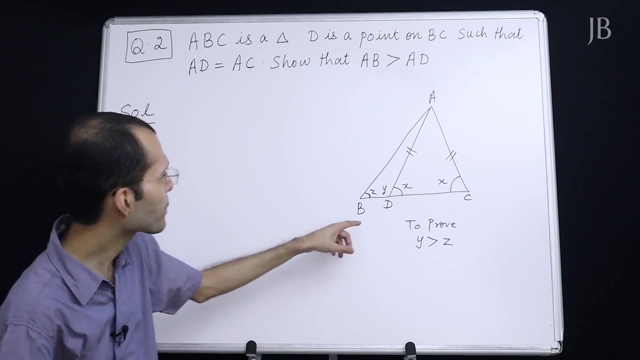 than z is becoming little tricky. So what to do Now? just observe: Whenever there are two equal sides given, we can use transition like we can prove something greater than this, and then this is equal, so we connect it. You'll get an idea. Observe triangle, ADC. Observe. 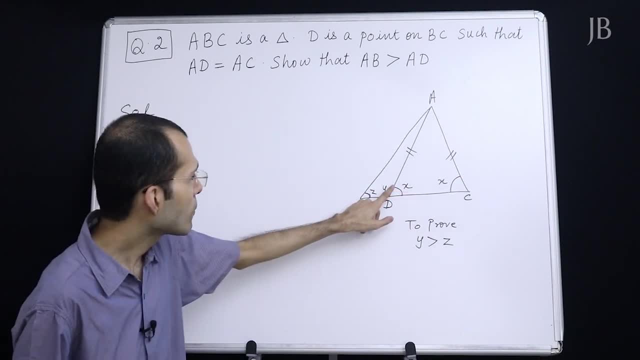 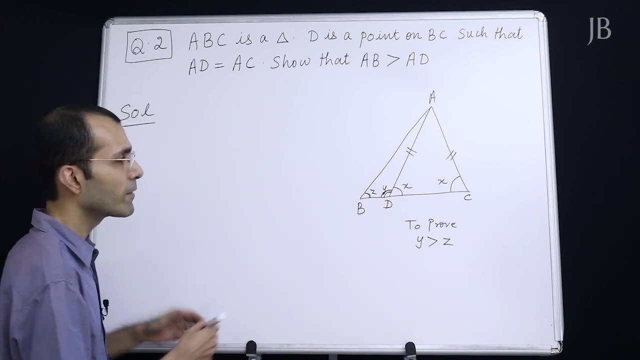 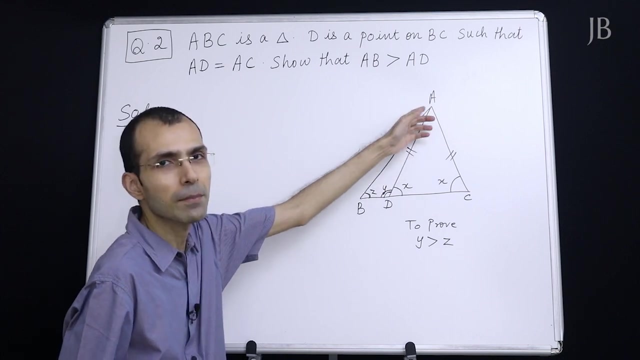 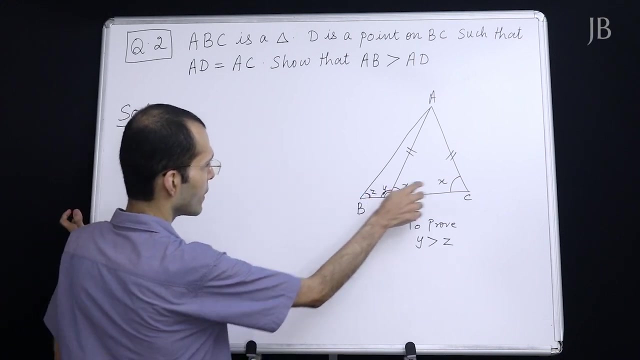 triangle ADC. This Y, don't you agree? it will be exterior angleY will be the exterior angle. So Y will be x plus this angle. Something. Exterior angle is equaling sum of opposite interior angles. So this Y will equal this x plus this angle. So let this be. 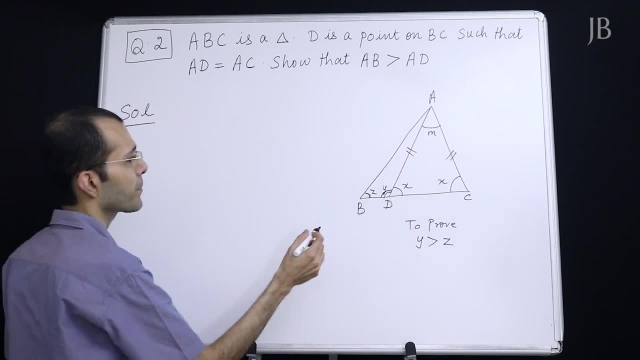 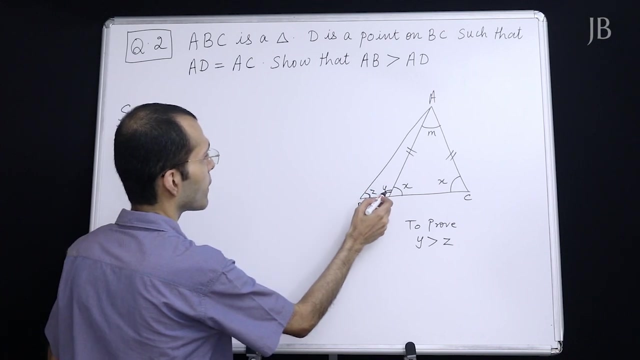 So this y will equal this x plus this angle. So let this be say m, if you want. So this y will equal x plus m. These angles, we can go on marking as in when the need arises. So y will equal x plus m. So now y is greater because y is. 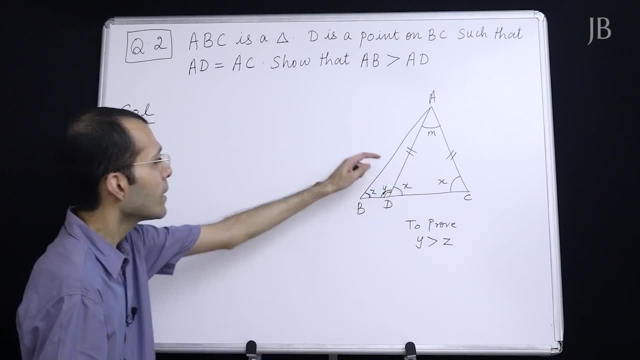 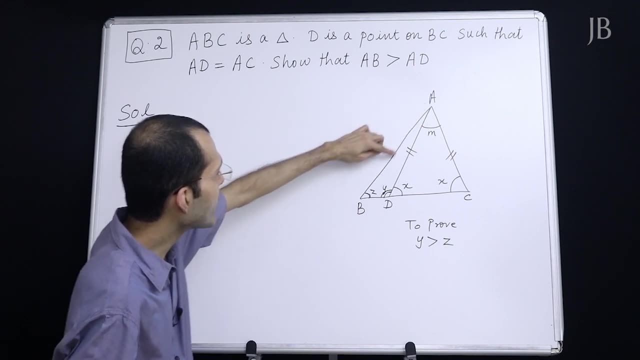 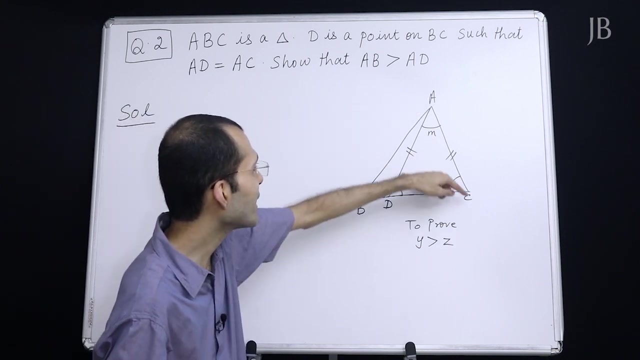 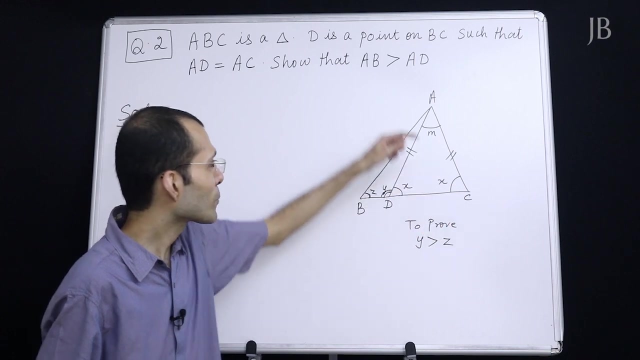 not x. y is x plus m. If y is greater than x, what will happen is side AB. side AB will be greater than side AC, because y is greater than x and opposite AC also comes. So your AB will be greater than AC. 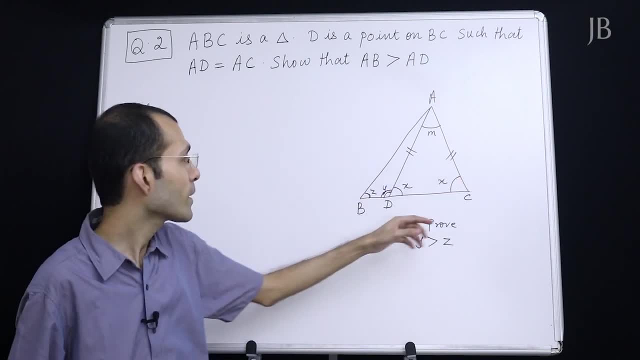 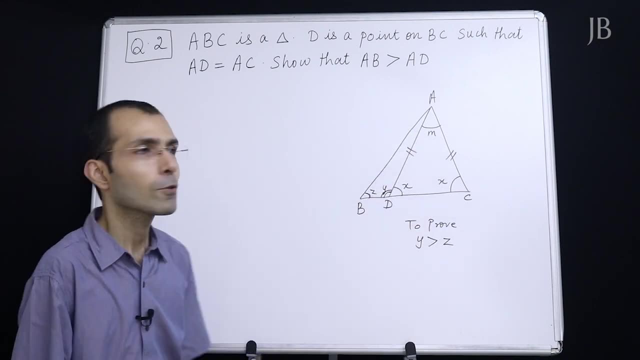 Now we are taking this triangle, Your ABC we are taking, you know. So AB will be greater than AC, but AC and AD are the same. So if AB is greater than AC, it will be greater than AD, also because both of them are of the 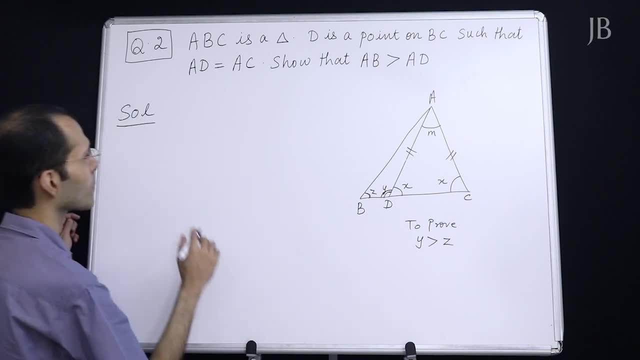 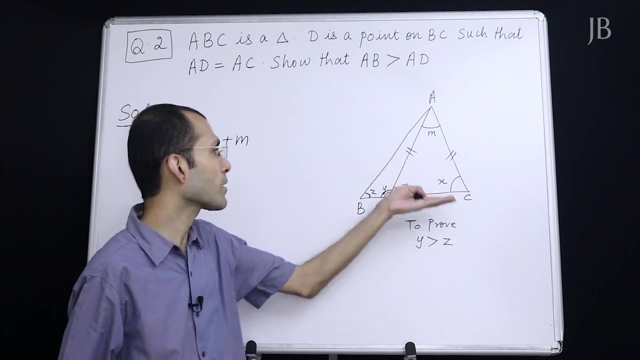 same length. So now let's see how we write the proof. So here this: we could not work it out, So now we will write like this: y is equaling x plus m. Now, now you may wonder: how do you know that we have to mark all these angles? 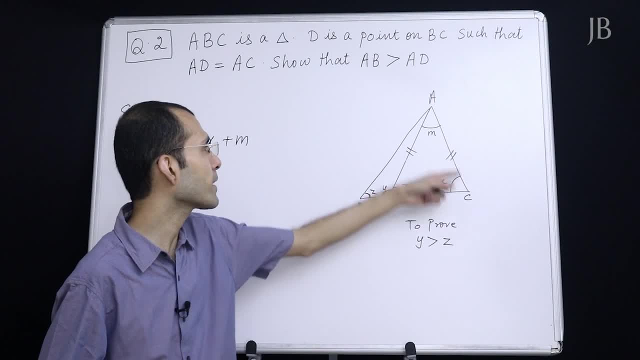 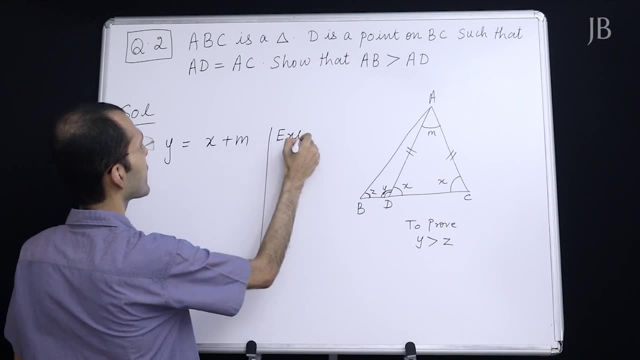 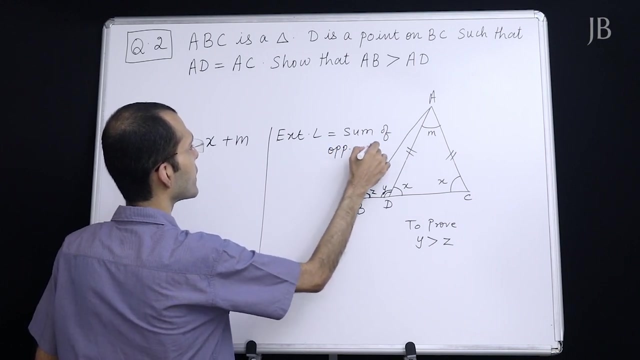 See. whenever the need arises, you mark it. Otherwise you write angle CAD Full form. No problem. y is equaling x plus m. exterior angle is equaling sum of opposite interior angles. Now if y is equaling x plus m, value will be increasing. 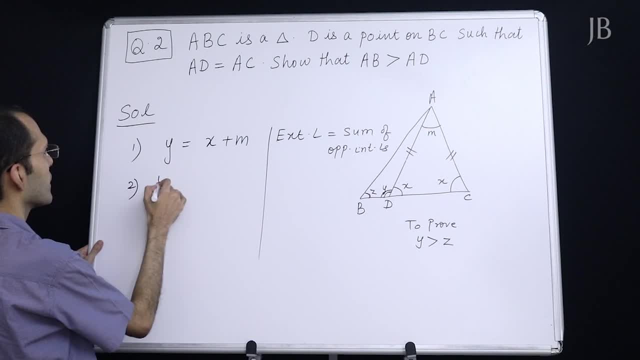 If y is equaling x plus m, exterior angle is equaling sum of opposite interior angles, x plus m. So this will imply y greater than x, naturally, Statement 1.. If y is greater than x, which is the side opposite to y, AB, So AB will be greater. 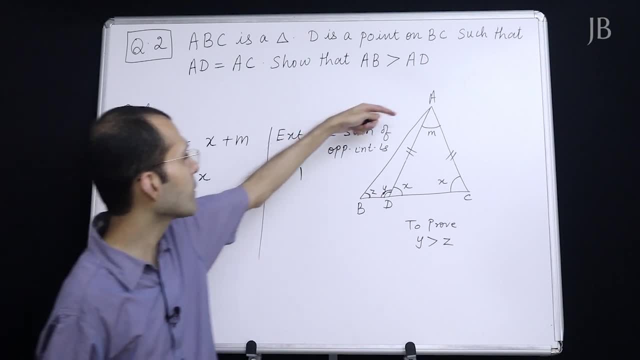 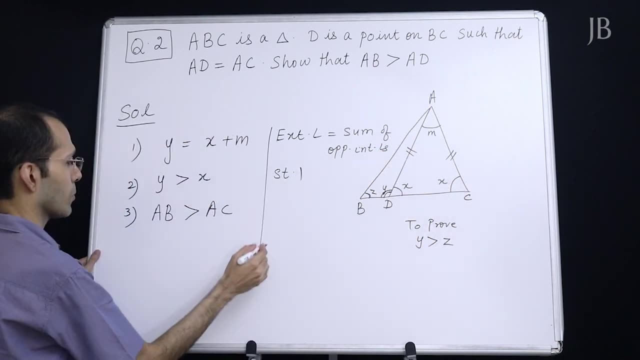 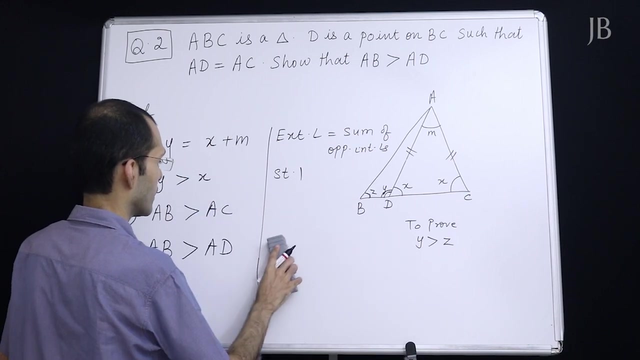 than AC. Here we are now focusing our eyes on triangle ABC, So AB will be greater than AC. Okay, but AC and AD are equal, So AB will be greater than. instead of AC, we will write AD because AC equaling AD. wait, here we will write the. 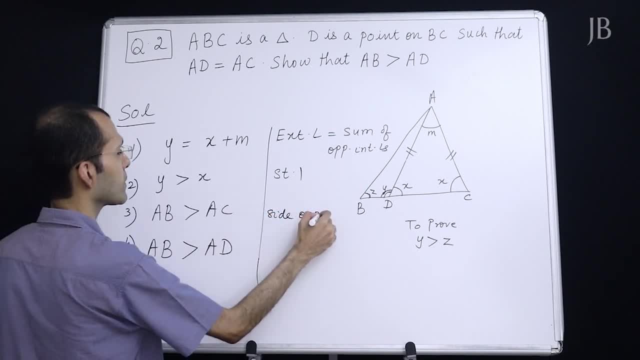 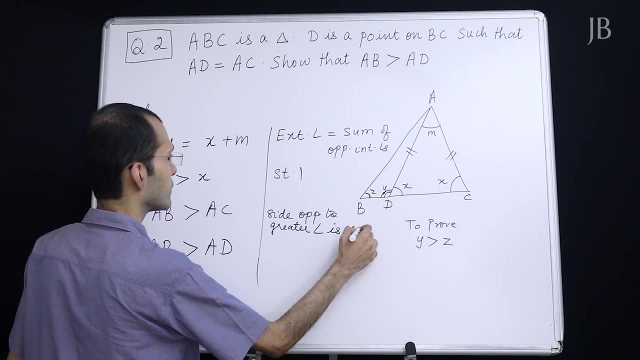 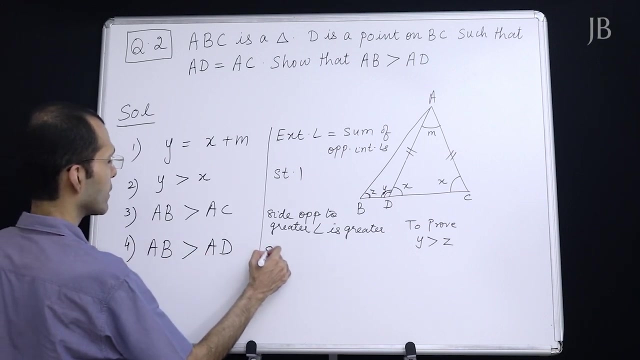 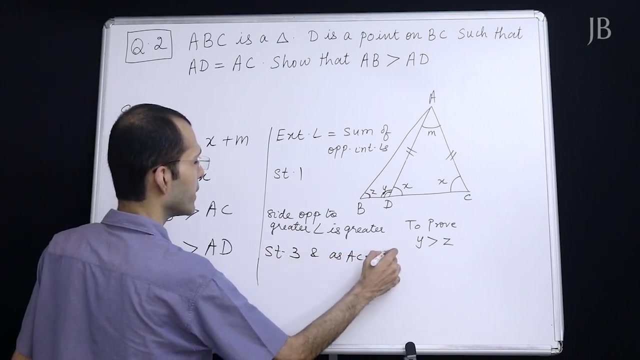 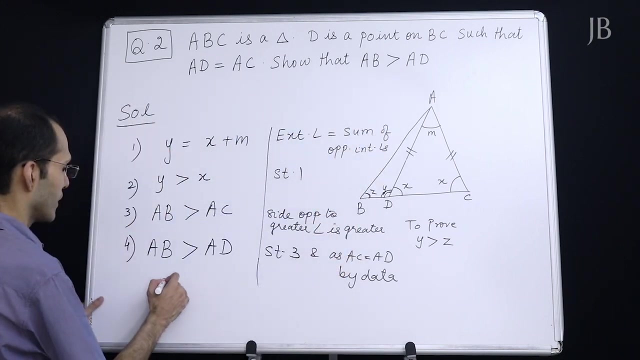 reason: side opposite to greater angle is greater And AC we have replaced with AD, So this region will be statement 3.. And as AC equaling AD by data. So we have proved, finally, AB greater than AD And that is what we had to prove, Hence proved. So these are: 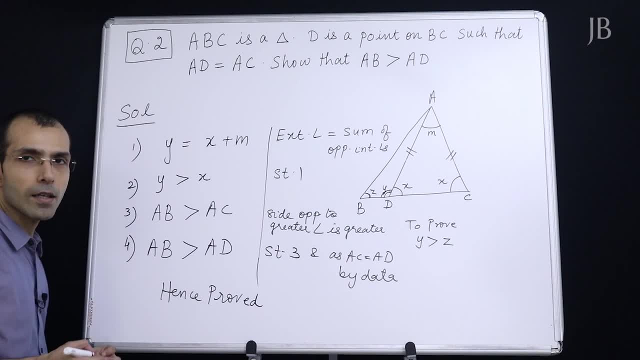 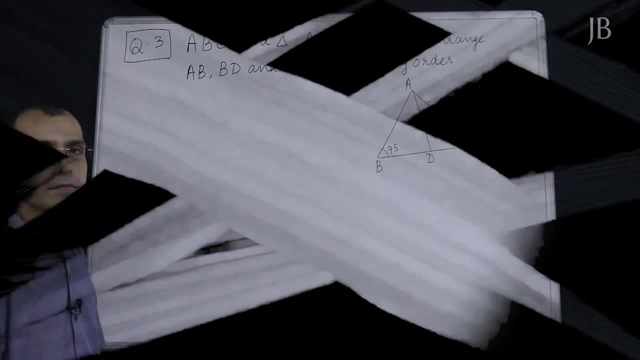 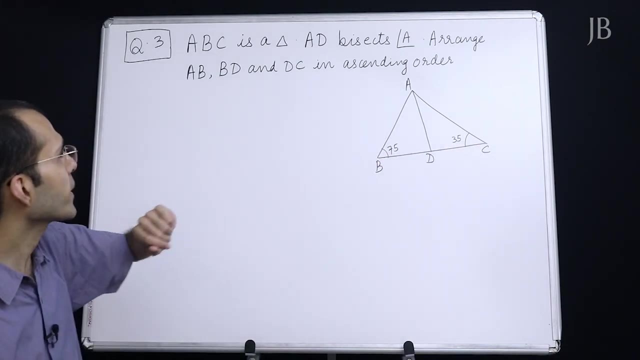 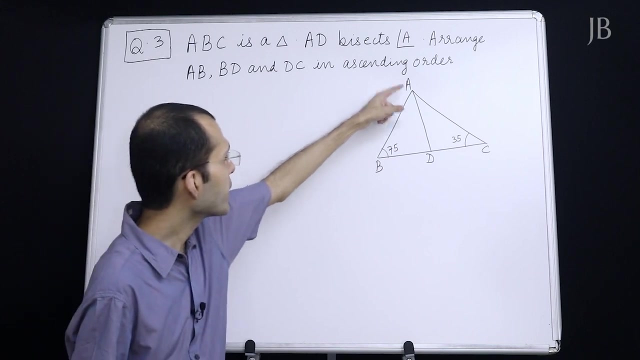 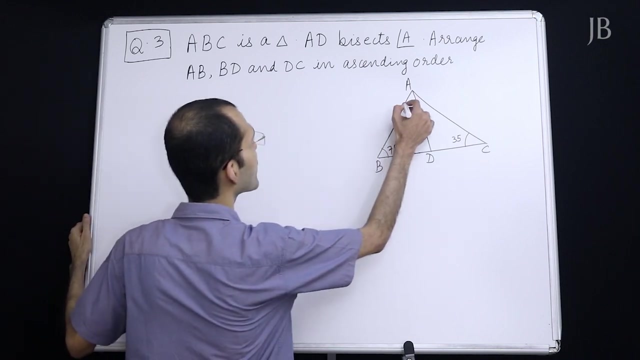 very short proofs Comfortable with this. So this is done. Question 2 now stands complete. Question 3. ABC is a triangle. Fine, The diagram has been drawn AD by bisects angle A. AD, bisects angle A, That is the entire angle A. So bisecting means let this be X. 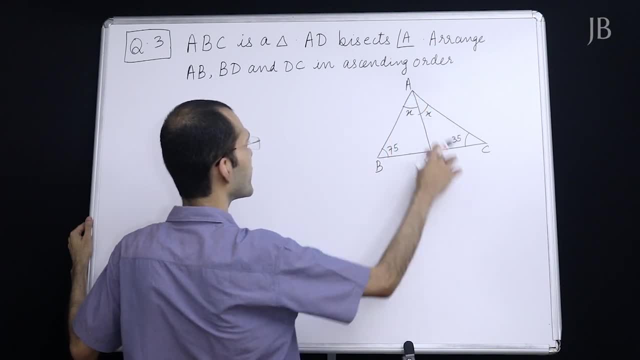 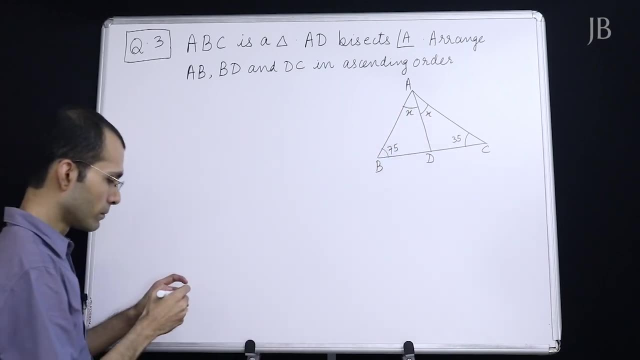 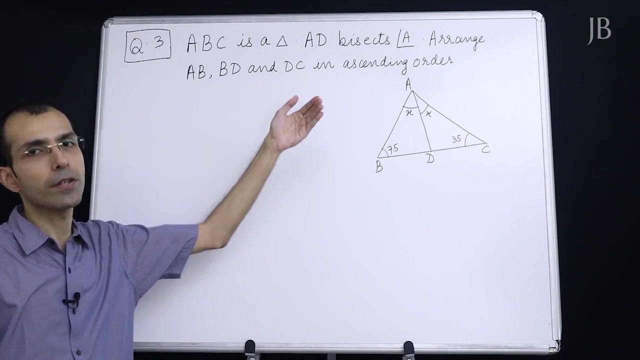 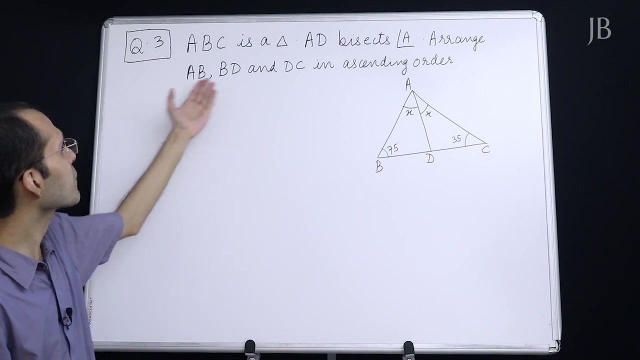 and let this be, X, AD is bisecting angle A. That means angle BAC. So you know what is the meaning of angle bisect. Arrange AB, BD and DC in an ascending order. So naturally, when they say AB, BD and DC, they stand for segments, Or rather length of their 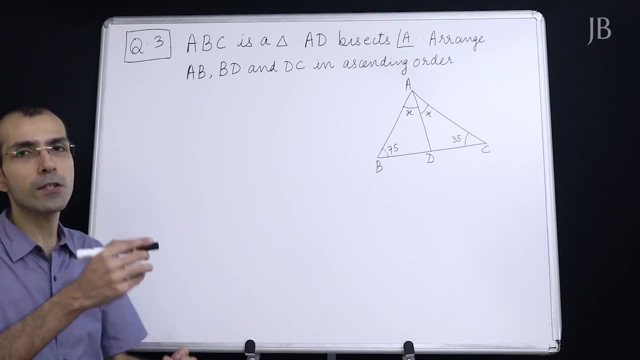 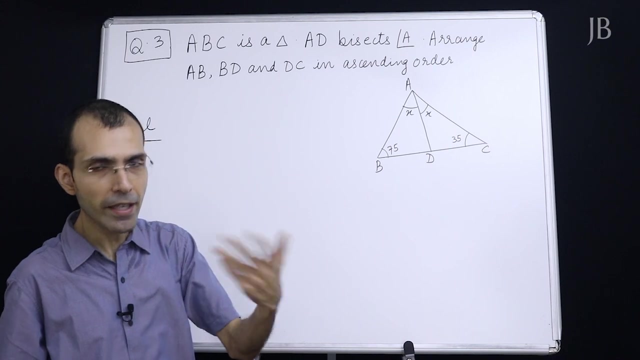 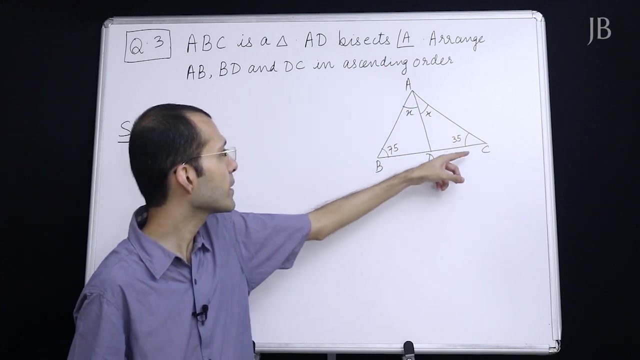 segments In ascending order. they are telling you That is from small to big. Okay, Here some values are given, So let's work out the angles. They may help us. Look at triangle ABC. This is 75. This is 35. So angle BAC will be how much Some of the angles of a triangle, Isn't it? 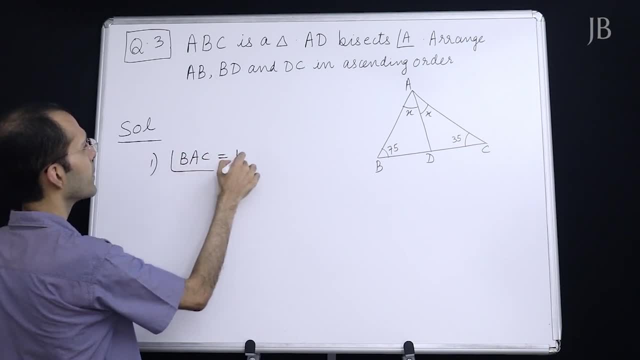 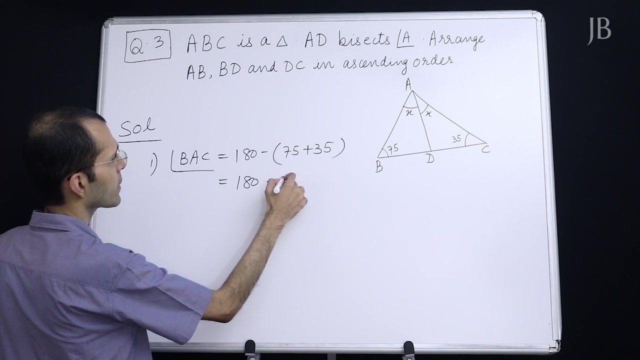 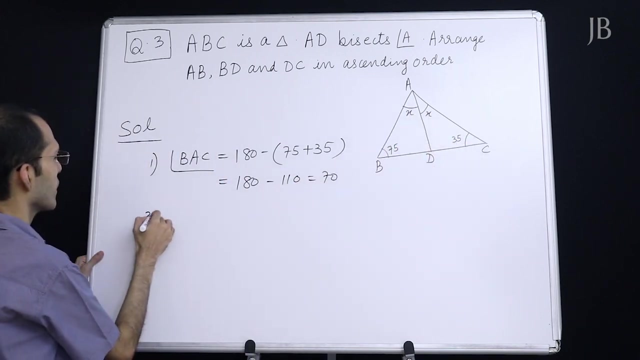 So angle BAC will be 180, minus of 75 plus 35. And this comes to how much? 110.. That comes to 70. So angle BAC will be 70.. But it is mentioned that AD is the angle bisector, So X will be how much? 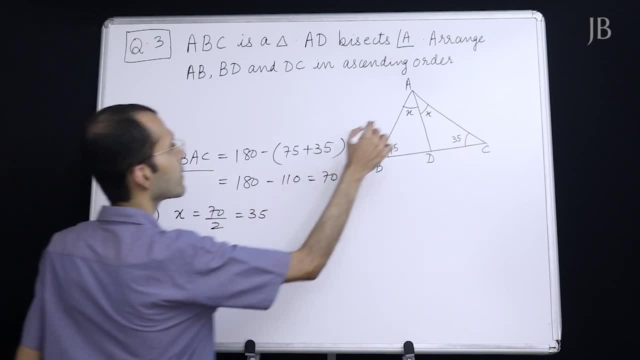 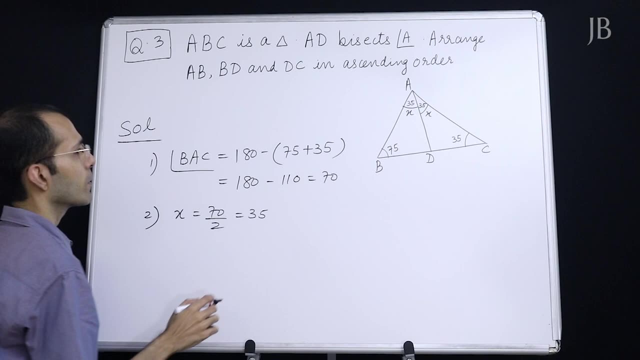 70 upon 2. That is 35. So this will write it here: 35, 35.. Okay, Here we will have to write the reason I am not writing it here. What is the reason? Some of the angles of a triangle is 180.. This is a small reason. 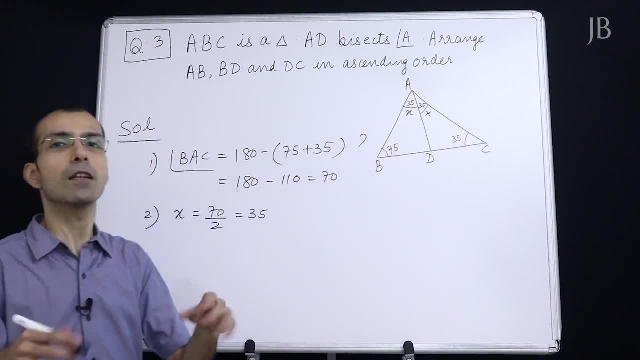 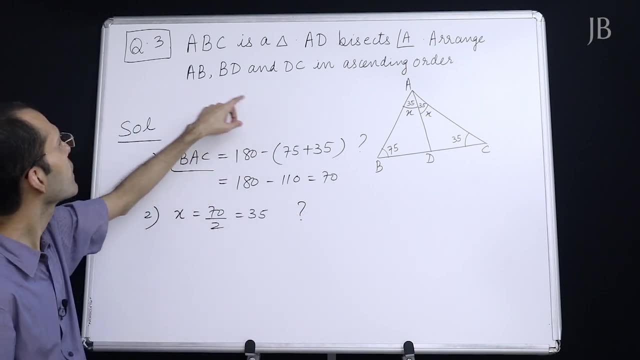 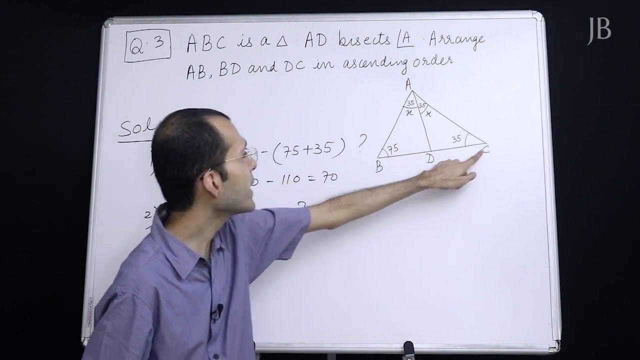 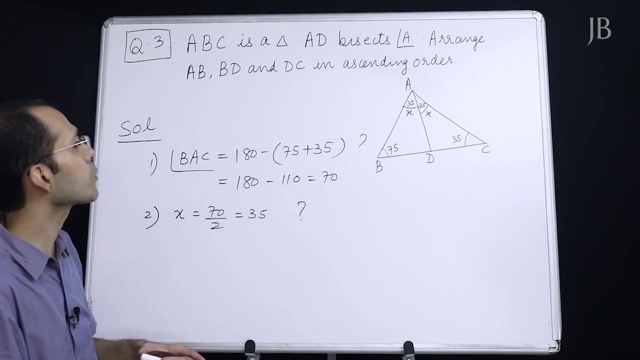 Okay, Okay, Okay, Okay, Okay, You can write it. AD is the angle bisector. Okay, Fine, Now what do we want to do? We have found the angles. You have to write AB, BD and DC in an ascending order, So from small to big: AB, BD and DC. 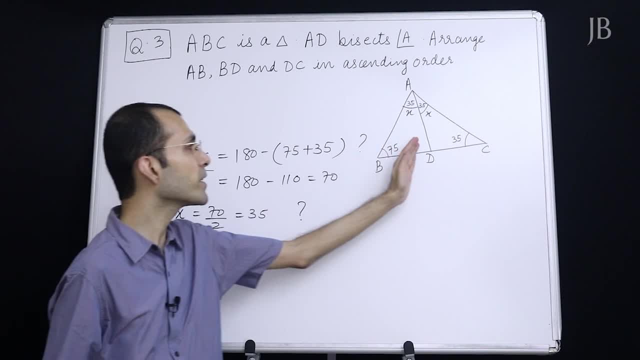 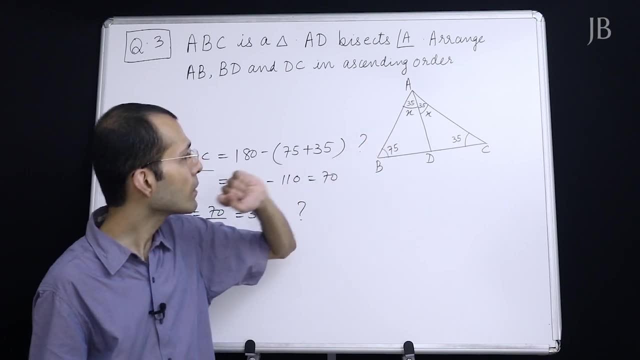 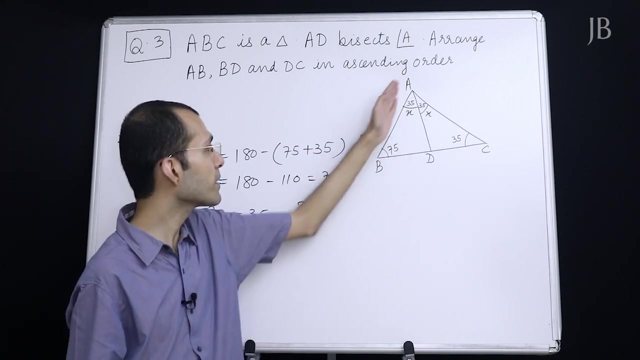 Now be careful. DC is going in the other triangle, So whenever we apply the properties, they are restricted to a particular triangle, So we may need a crossover Like: see, AD is a side which is coming in this triangle and AD is a side which is coming in triangle ADC as well as ADB. 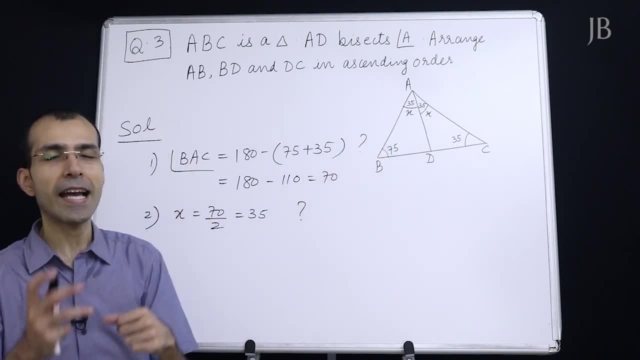 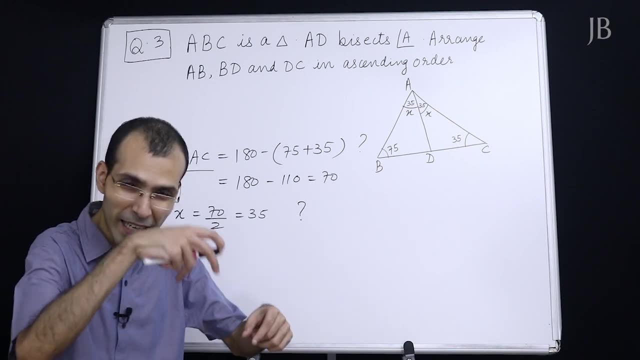 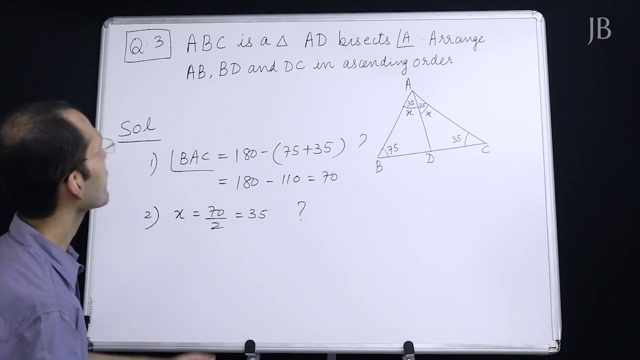 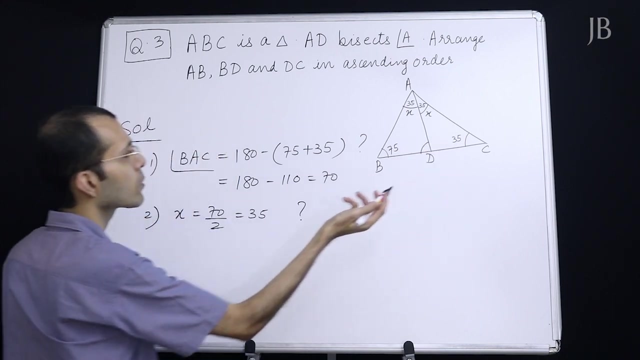 Because you cannot use the property angle opposite to Side, opposite to greater. angle is greater. We can, but it should be used in that one single triangle at a time. You can't compare two different triangles like that. So, anyway, now here they are talking about AB and BD, Right? So let's first compare AB and BD. which is greater? AB is opposite to this angle. This angle we do not know, Let's find it out. We call this as 1.. 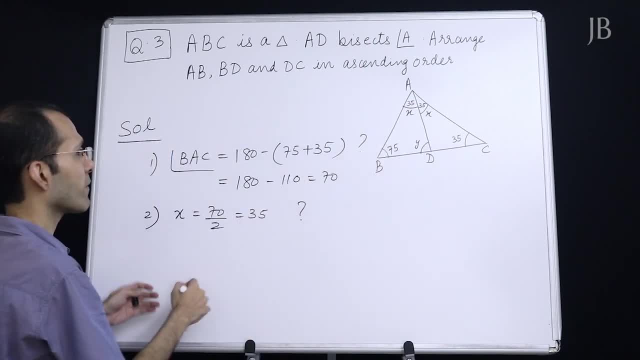 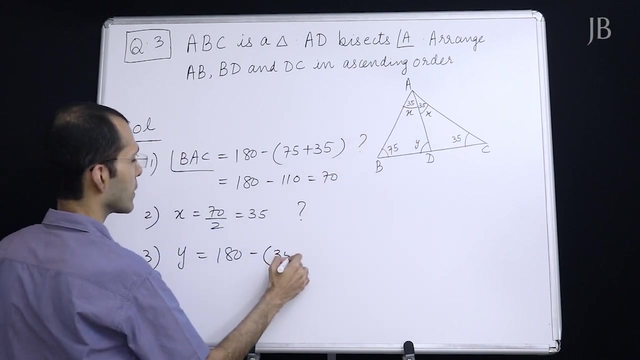 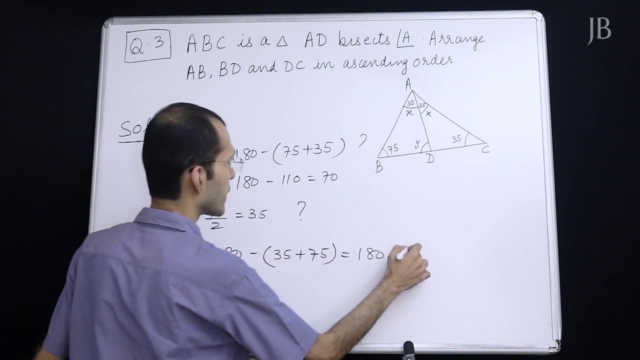 Y, Mark it in the diagram. If you write only Y here and you have kept it in mind but not shown it in diagram, that's a serious offense. So Y will be 180 minus 35 plus 75.. That is 180 minus 110.. That comes to 70. 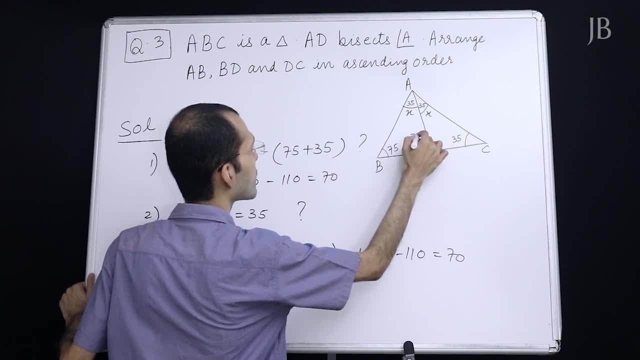 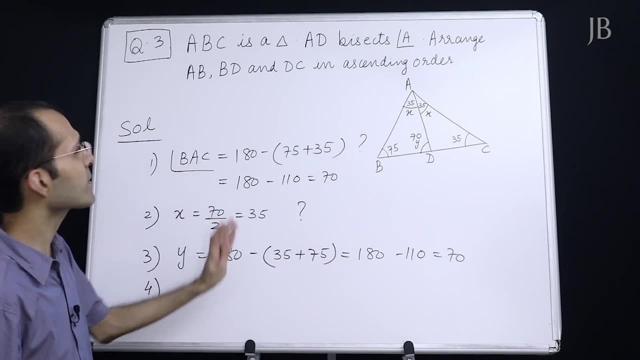 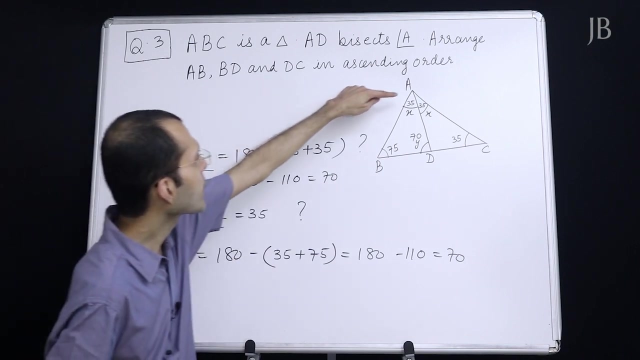 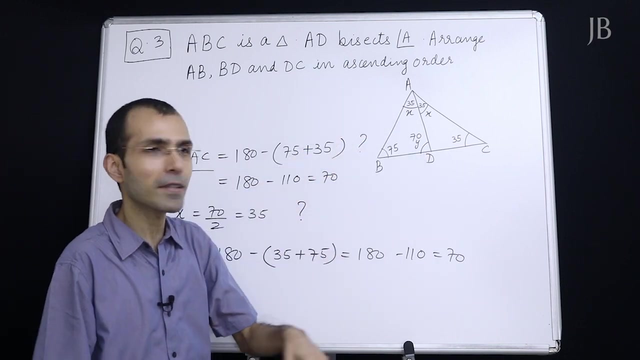 So Y is 70. No need to write units and all Only in the final answer. you write the units wherever required, Not in the intermediate steps. Okay, Sorry, Now see we are comparing AB and BD. Not a problem, because AB and BD both come in the same triangle, That is ABD. 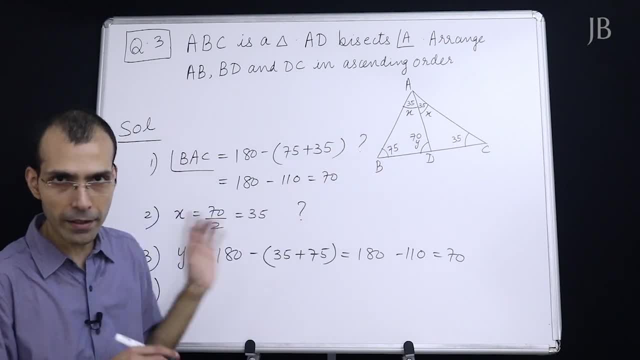 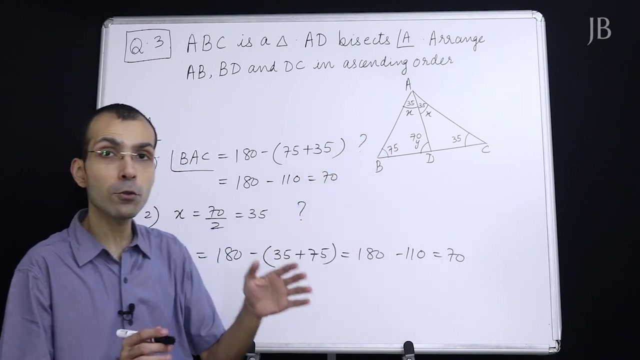 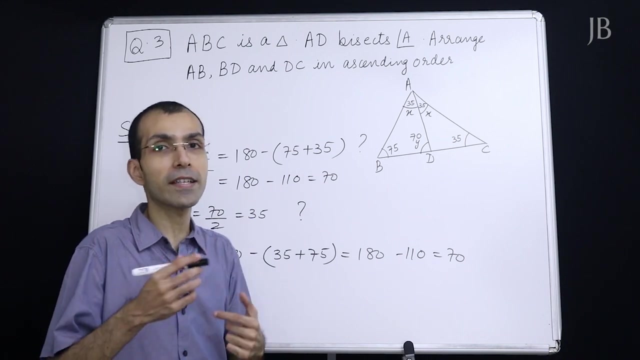 So opposite to 70 degrees. Very clear: BD is opposite to 35 degrees. So who will be greater? Naturally, AB will be greater than BD, because AB is opposite to 70 degrees and BD is opposite to only 35 degrees. So side opposite to greater angle is greater. So now we will write AB. 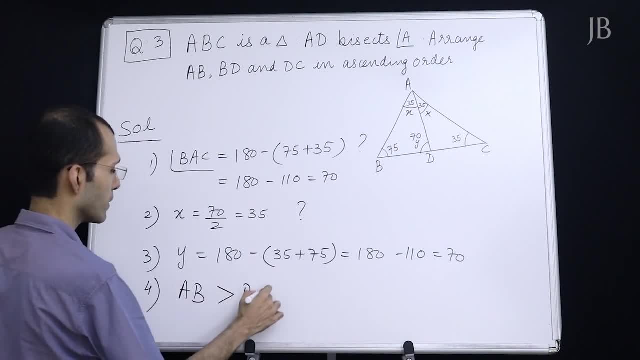 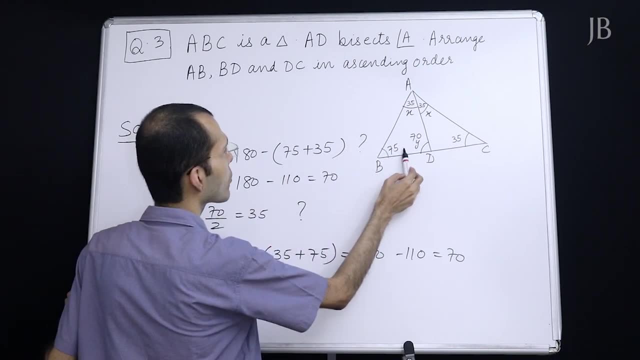 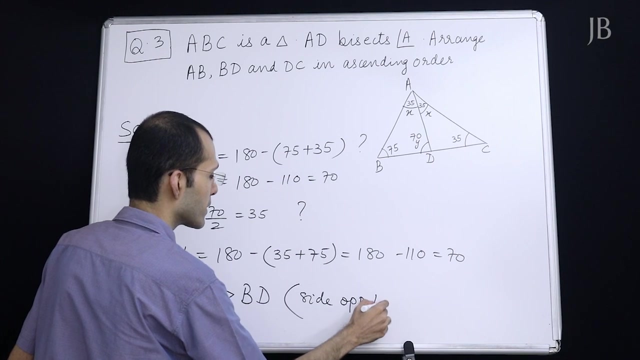 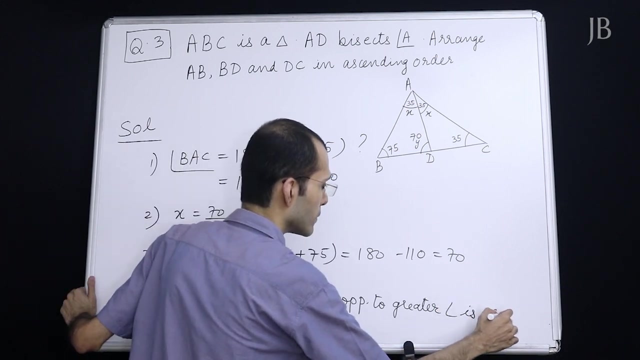 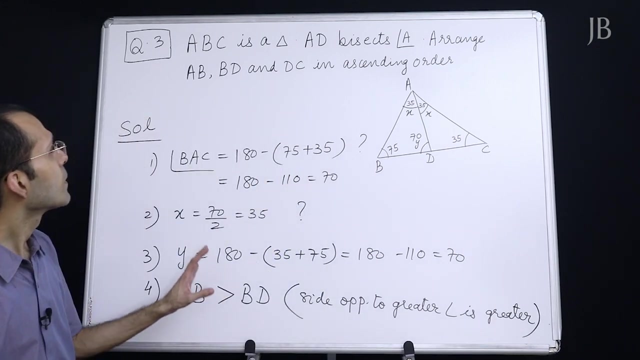 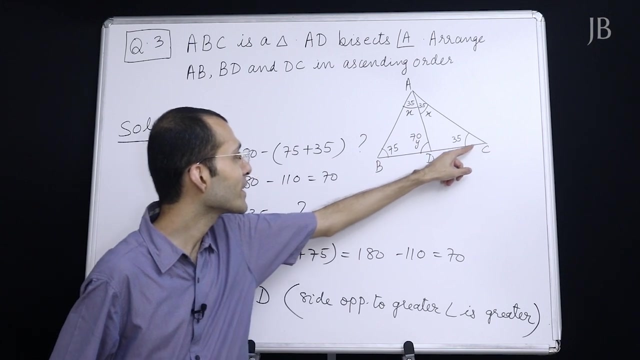 Greater than BD, Because AB is opposite to 70 degrees and BD is opposite to 35 degrees. So side opposite to greater angle is greater. So side opposite to greater angle is greater, So side opposite to greater angle is greater. This is done. So now AB and BD has been done. But wait, There is one more remaining: DC. 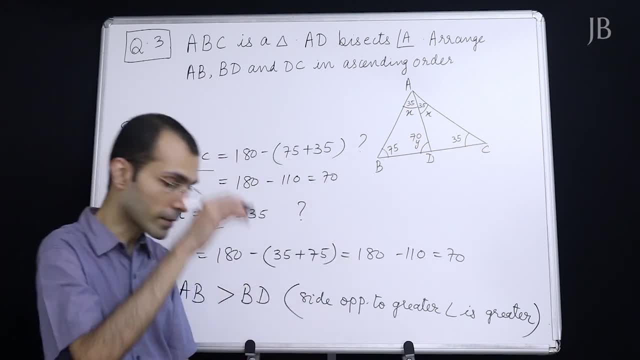 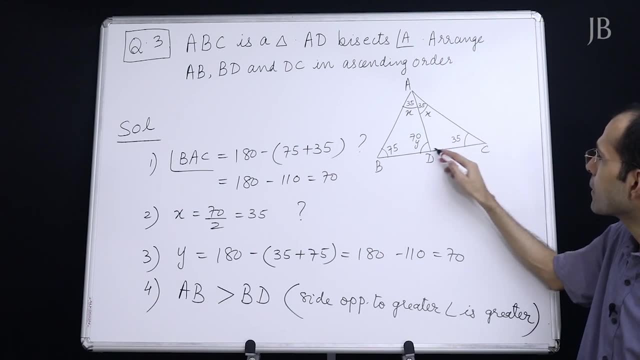 But DC is coming in the other triangle. Now DC is opposite to 35. Right, This DC is opposite to 35 degrees. Now this DC, we will compare with AD. Why we will do that? Because AD comes in this triangle and AD comes in this triangle also. 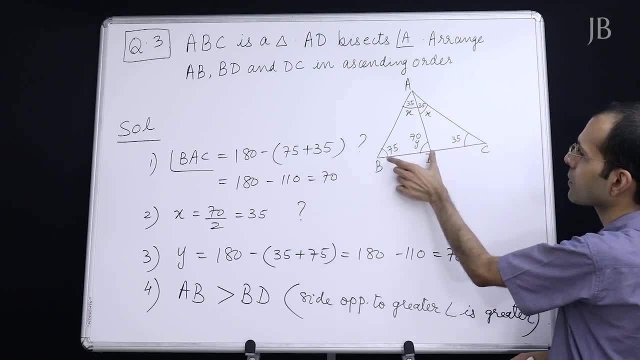 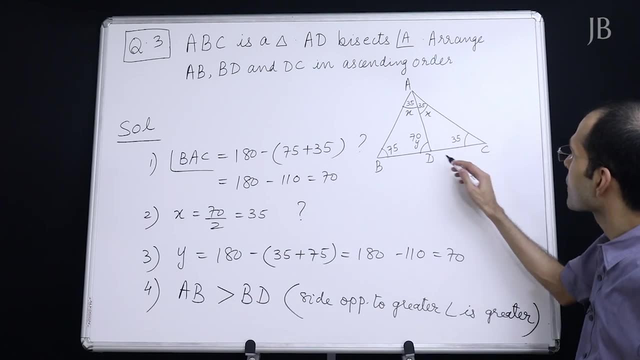 So it will help us to cross over, Otherwise you cannot take the angles of this triangle and comment on the length of the sides of this triangle. Now, DC is opposite to 35 degrees. I will just write for your understanding here: DC is opposite to 35 degrees. 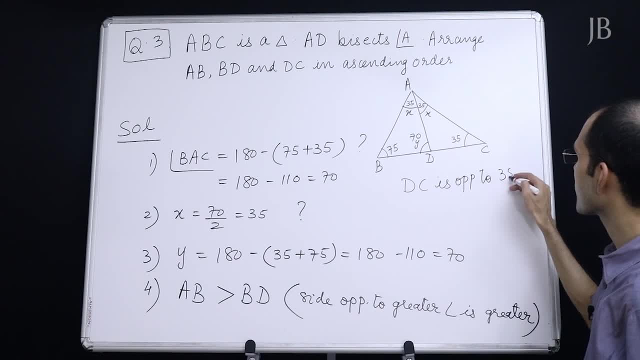 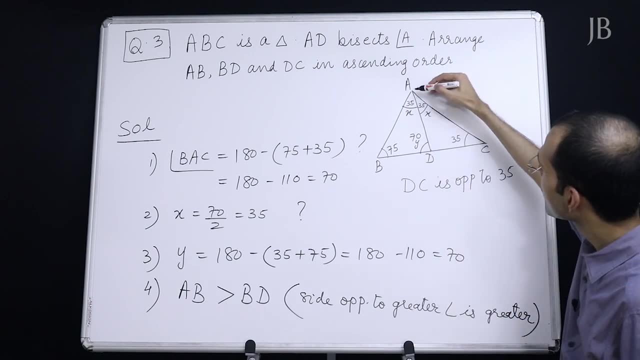 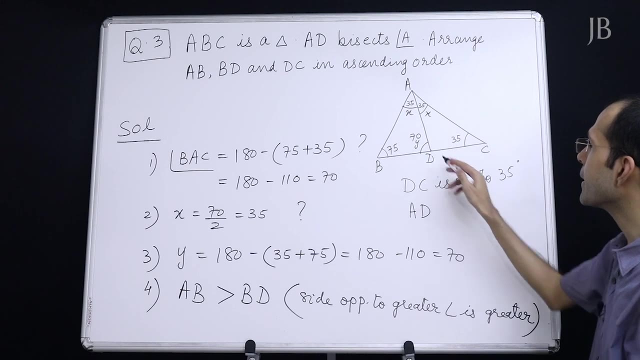 opposite to 35 degrees In the exam. also, if you want, you can write like this, no problem. DC is opposite to 35.. Look at AD now Look at AD. AD is also opposite to 35 degrees. Now we are looking at this. 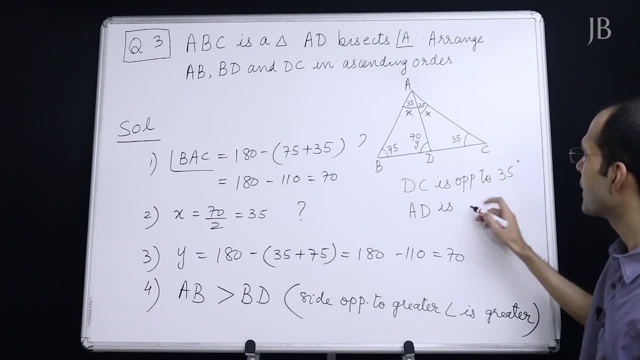 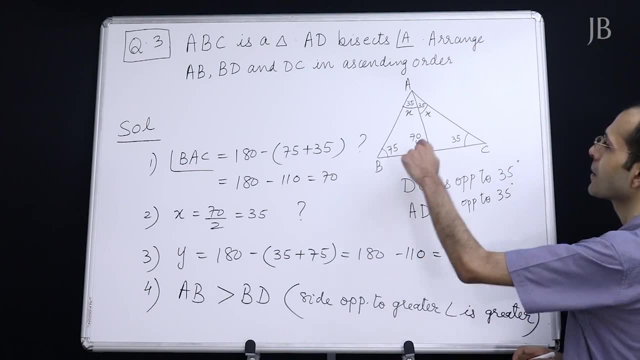 triangle. okay, We are looking at this triangle. ADC, AD is opposite to 35. Is something striking your mind? DC opposite to 35. AD also opposite to 35. So what will be the relation between AD and DC? What would be the relation between AD? 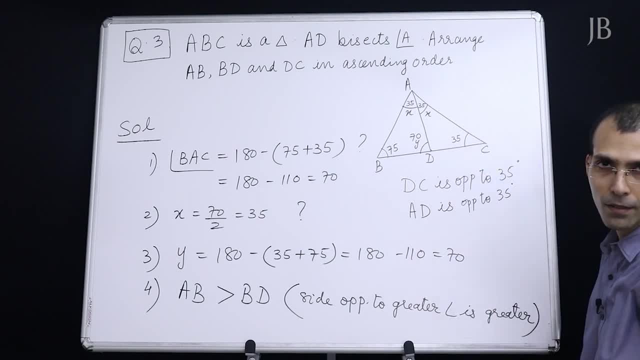 and DC. They will be greater. Who will be greater? Nobody, Both will be same, because AD is opposite 35 degrees and DC is also opposite 35 degrees. You have to look in one triangle at a time. So now this implies that AD is equaling DC. 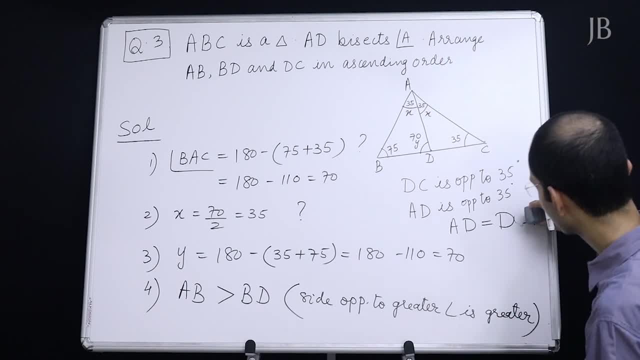 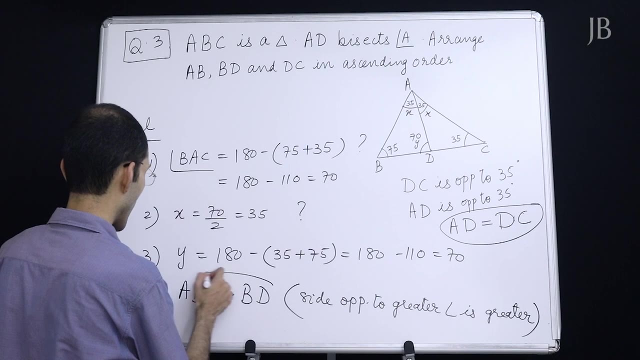 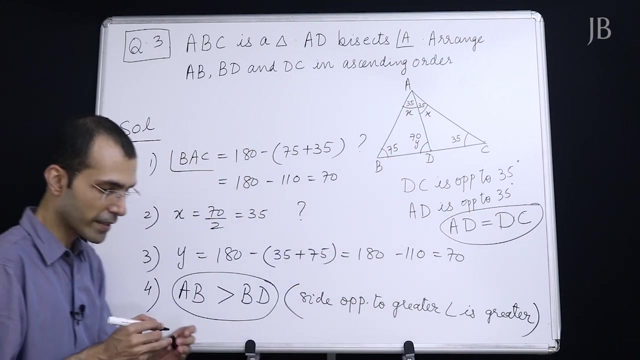 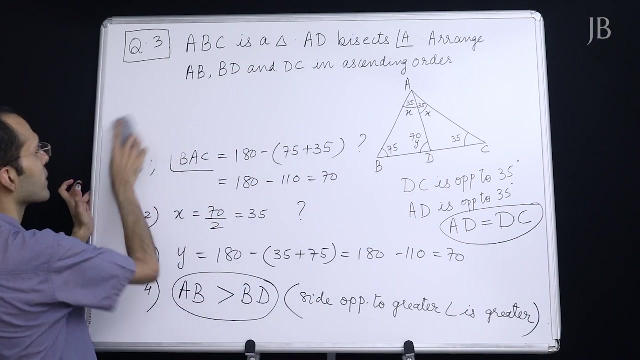 So AD and DC are equals. So this one logic we have now found out, and somewhere else we found out this AB greater than BD, and now we came to a conclusion that AD is equaling DC. Now connect both of them and see whether we can get whatever is asked in the 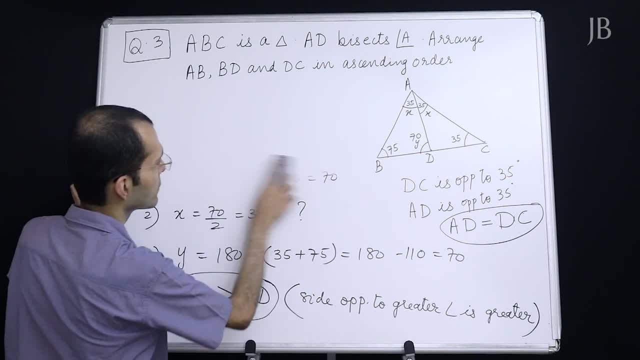 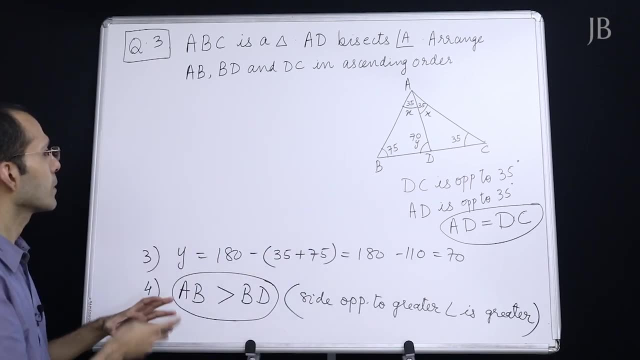 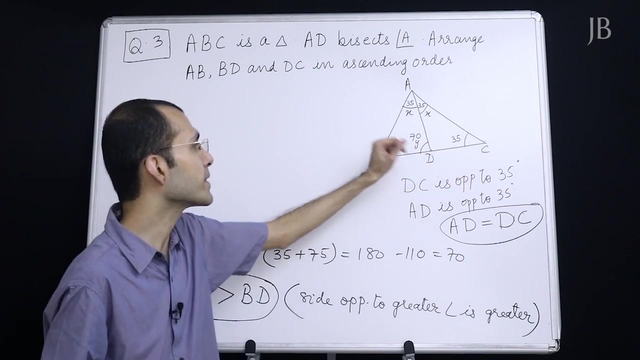 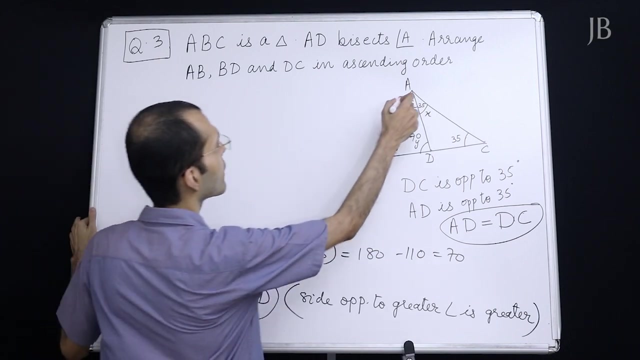 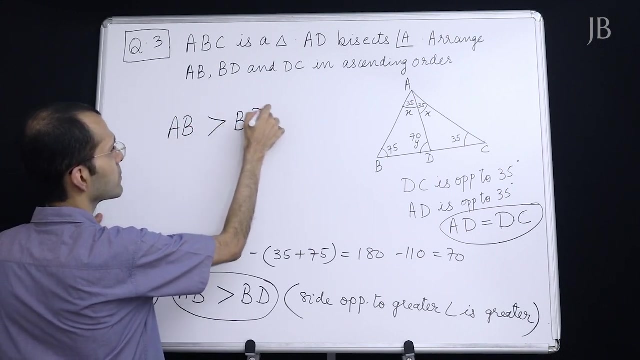 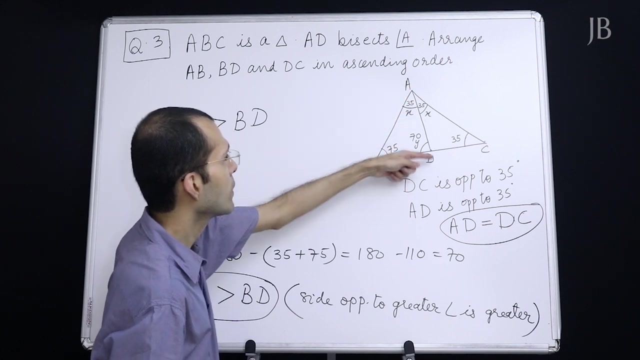 question This will erase now. OK, Coming to this, we want AB, BD and DC. This we want now to be arranged in ascending order. So what will happen? AB is greater than BD. That too, we proved it clearly. What about AD now? Now, AD and DC are same. 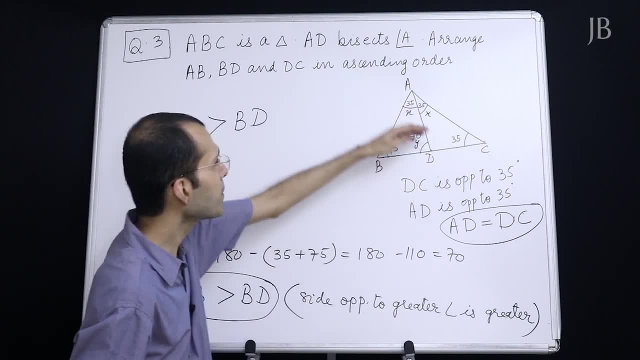 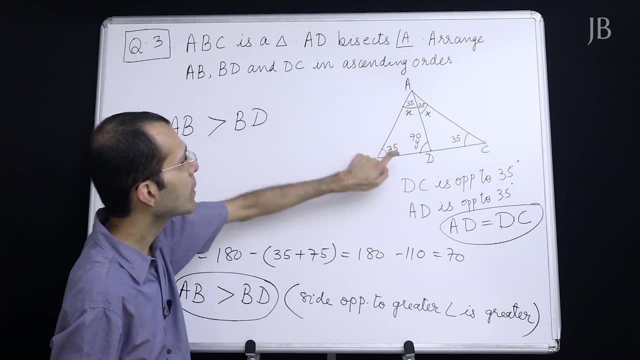 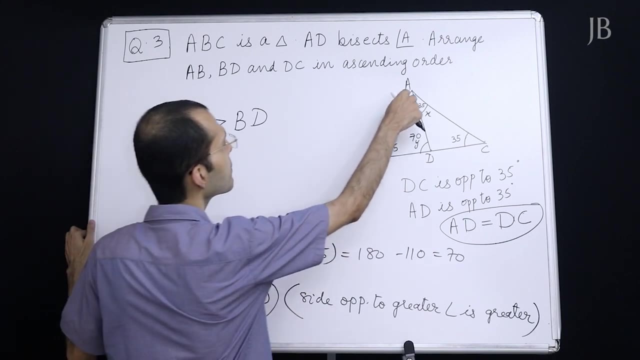 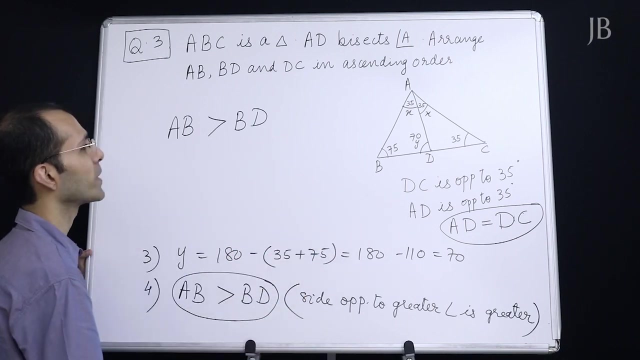 So what you do forget DC for some time. you concentrate on triangle ABD, You try to arrange AB, BD and AD in ascending order and then, in the end, simply replace AD with DC, because AD and DC are the same. We just now proved it. 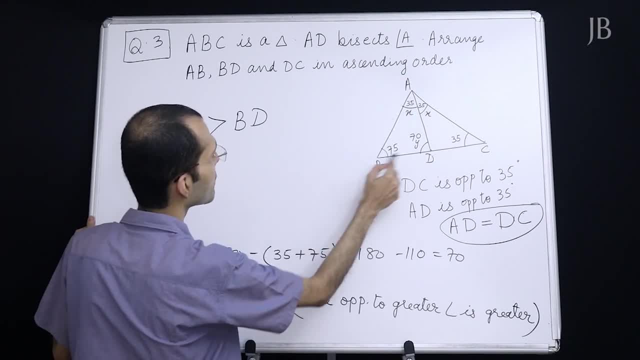 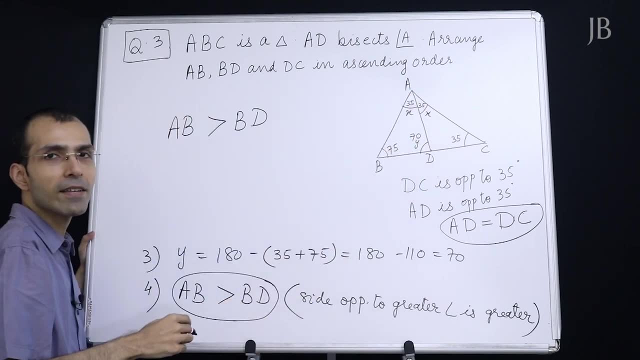 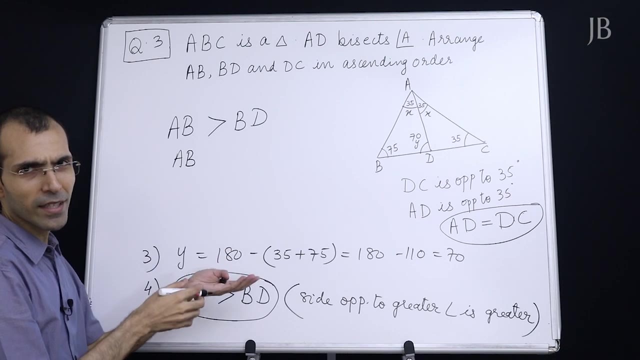 Okay, now see, AB is greater than BD. Okay, what about AD? AD is opposite to 75 degrees. So here we'll write again for understanding This. you can either do it in the mind and just write down the answer. No need to write so many steps in. 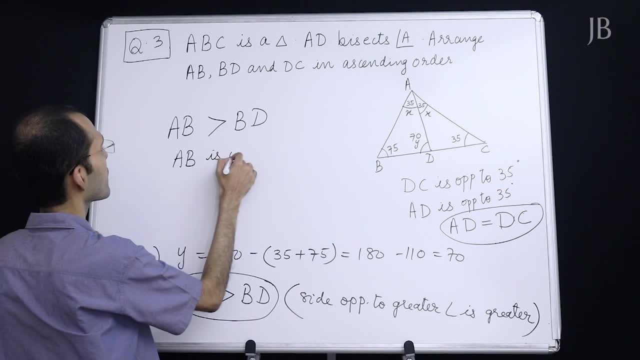 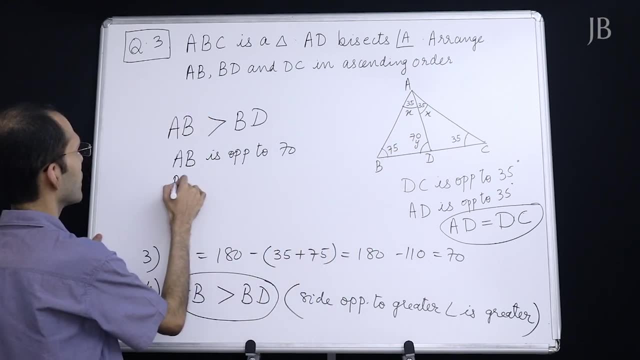 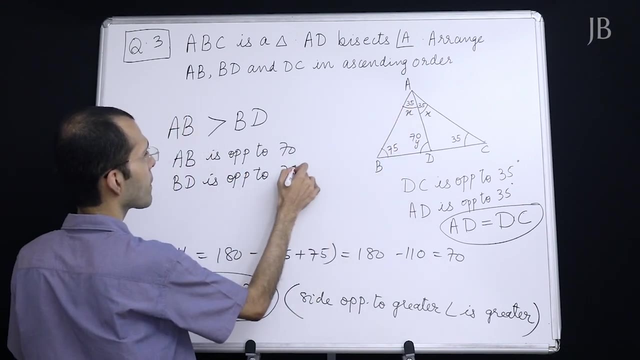 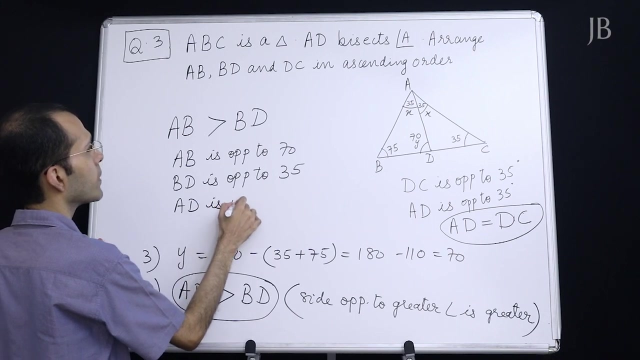 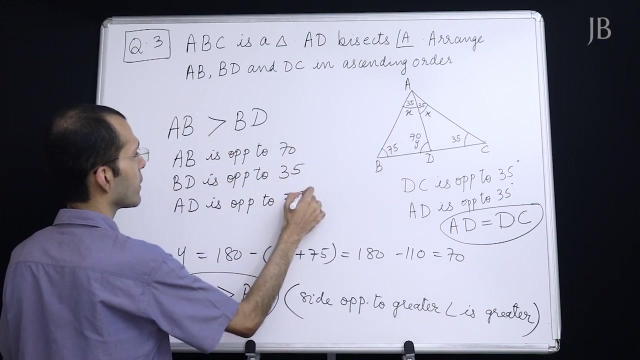 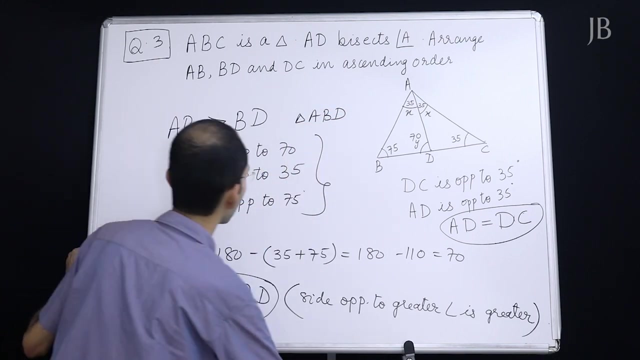 the exam. AB is opposite to 70.. AB is opposite to 70.. BD is opposite to 35 and your AD is opposite. AD is opposite to what? 75.. Which triangle have we considered here? Triangle ABD. Why we had to do all this. 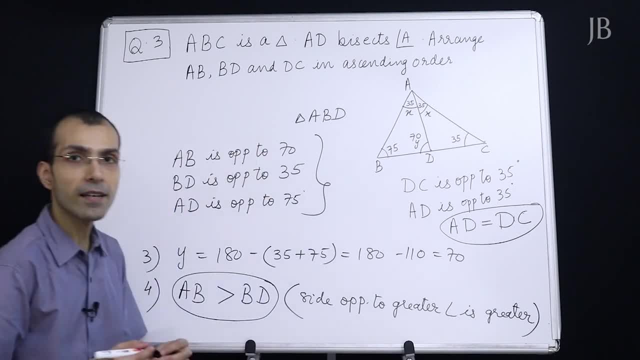 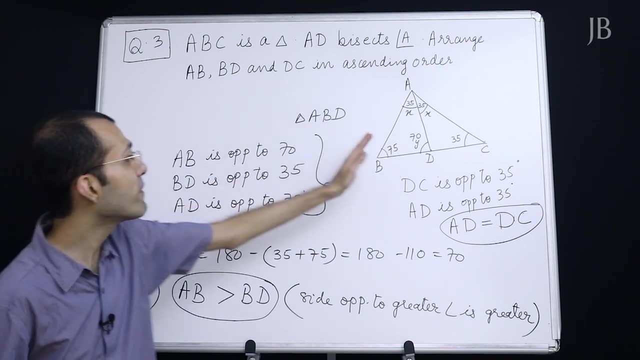 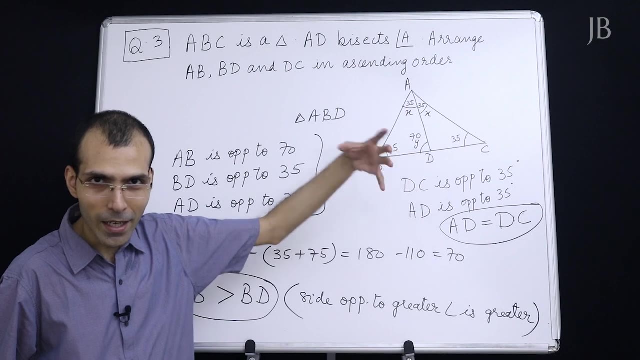 so much effort? Because they asked us to compare three sides, of which two sides were in this triangle and one side went in the other triangle, So we could not compare directly. So whenever they tell you compare three sides and of which two sides are in one triangle and the other, 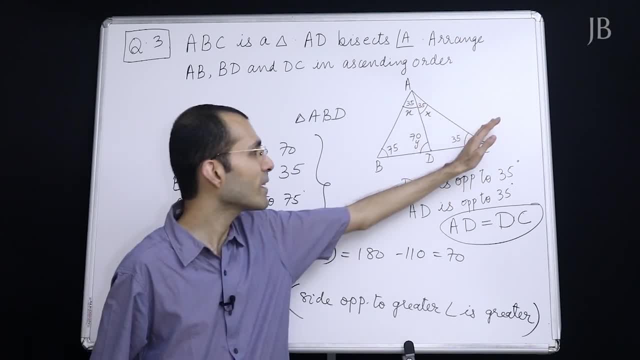 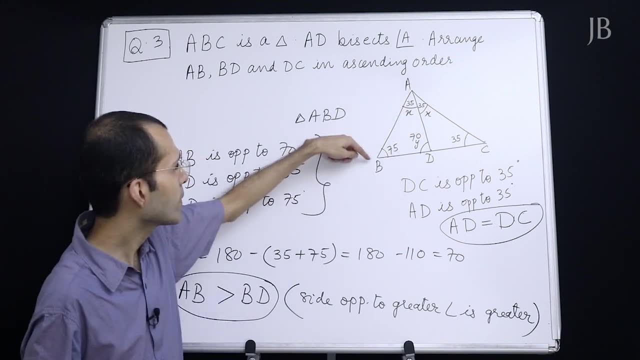 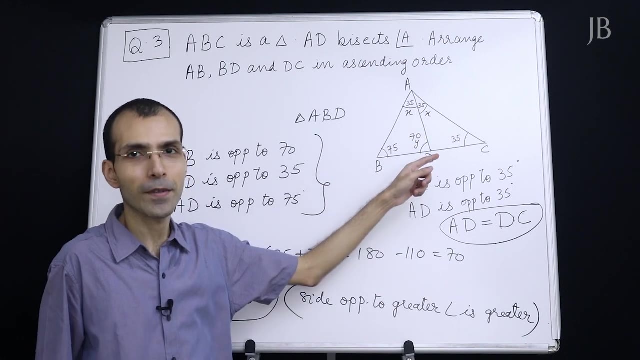 side is in the other triangle. what you do is you keep that other side aside for some time. You try to first get that one original triangle ka all the three sides in ascending order, and then normally in such sums there will be a common side right Which will be shared. 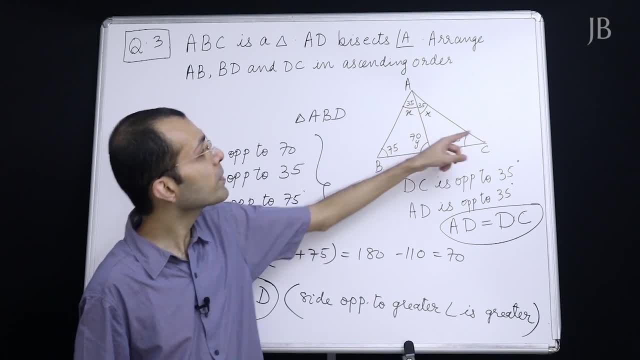 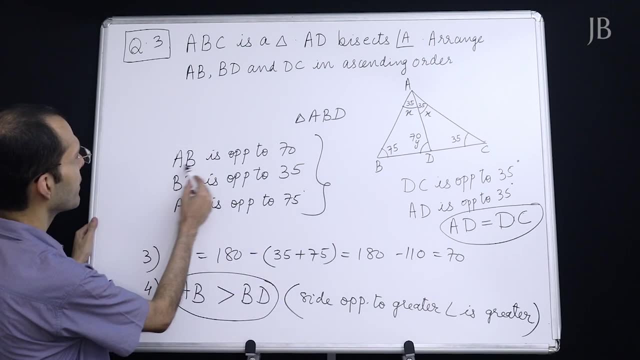 by both the triangles, That common side will turn out to be equal to the side which you have to compare. So we can replace them like that. Okay, so now A, B is opposite to 70,, BD is opposite to 35,, AD is opposite to 75. So now we are. 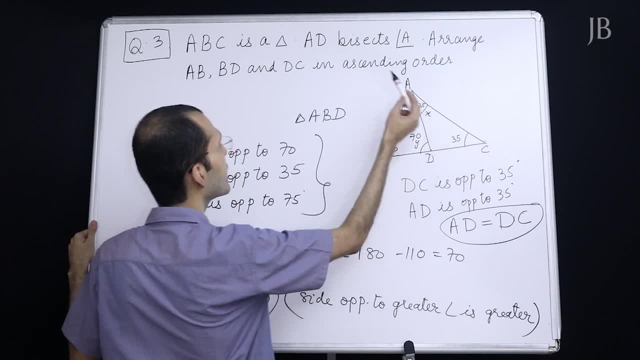 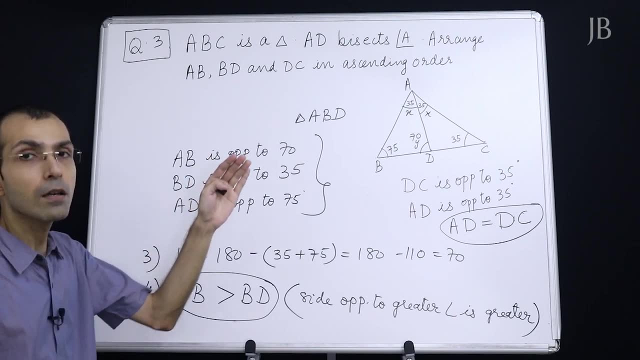 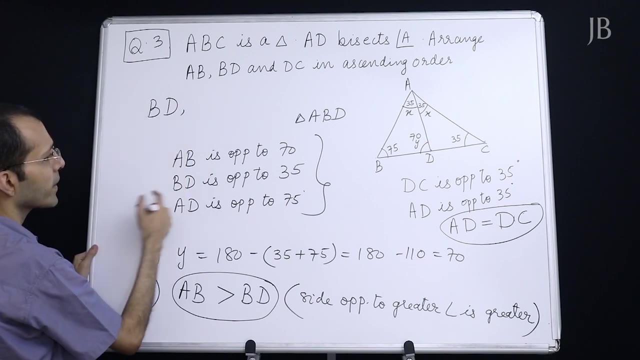 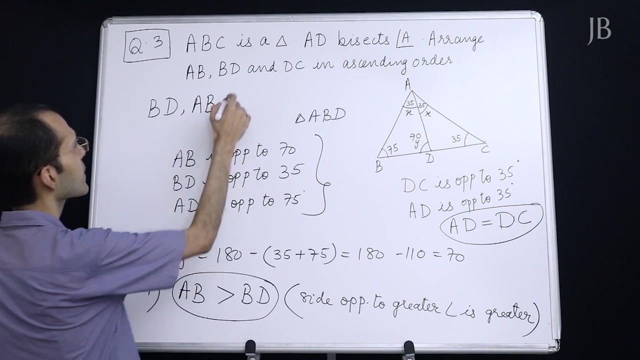 focusing our eyes only on triangle, ABD. So which one? Now ascending order means what Small, big, bigger like that? So which is the smallest here, BD, Then little more big, AB, And which one will be the greatest, AD. So this is your ascending. 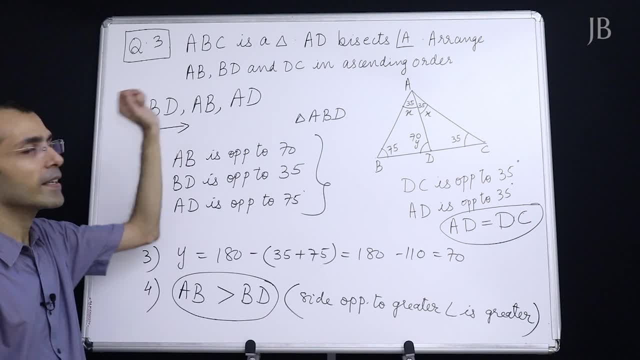 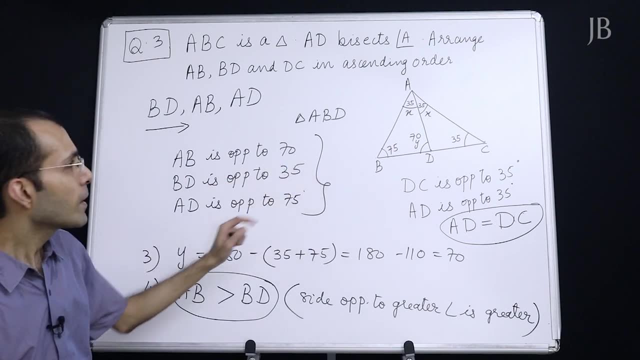 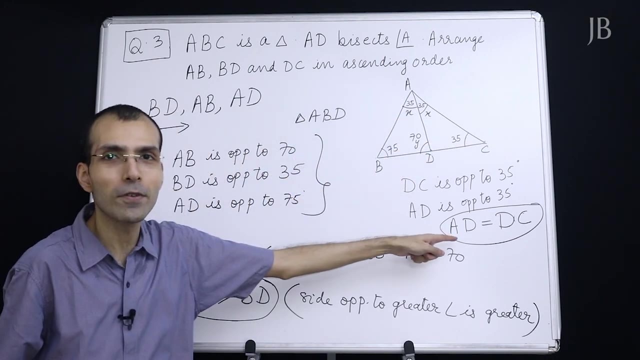 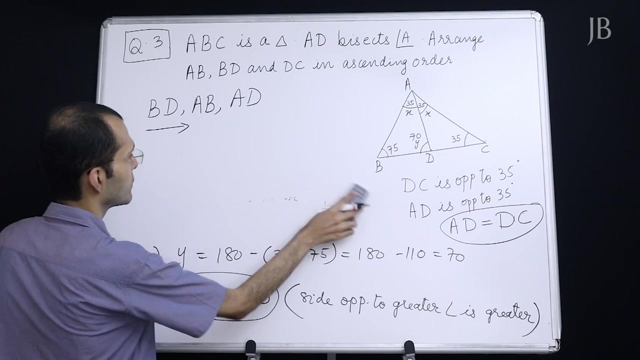 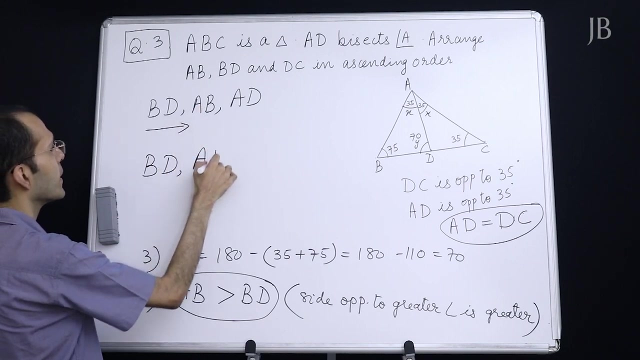 order: BD, AB and AD. But the problem is: AD is not required. They are. they want you to get DC. So AD and DC are equal. We just now proved it: AD and DC are equal. So So now final answer will be: BD, AB And AD is not required. They want DC to. 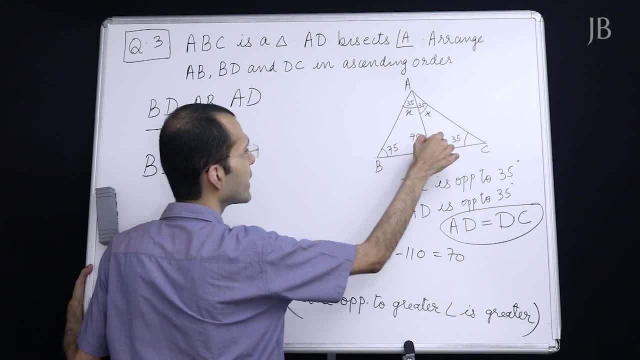 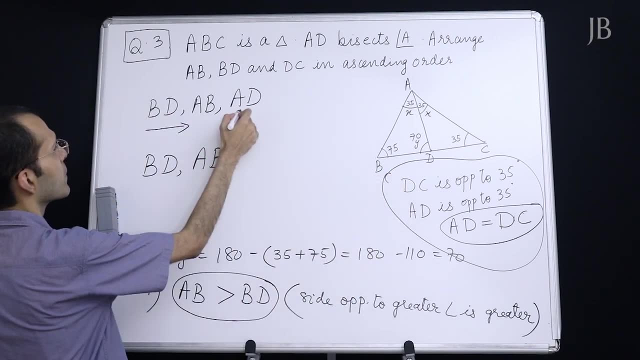 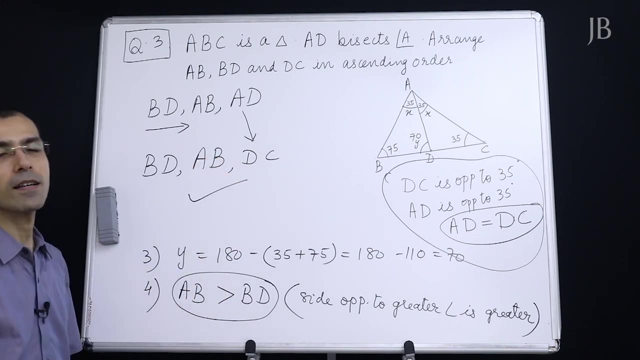 come in the picture, And just now we proved that AD and DC are same because of this argument. So this AD can be changed with uncrwen, который refuse our answer with DC, and this will be our ascending order. Comfortable with this, sir, Had they. 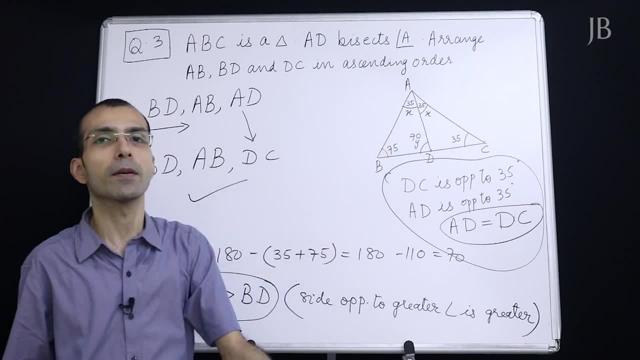 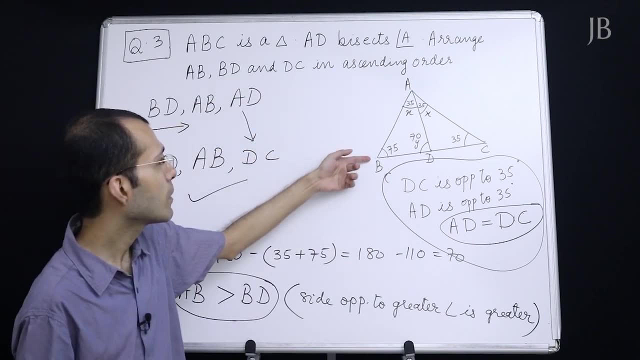 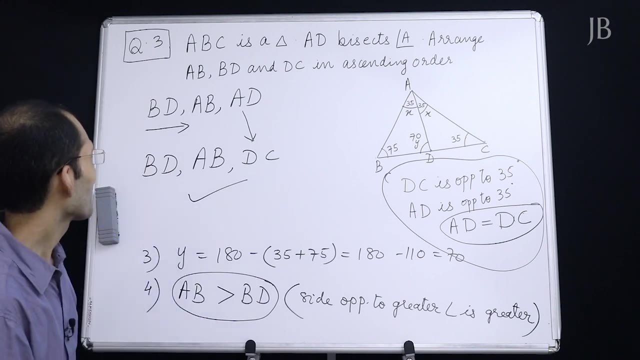 asked you compare AB, BD, DA. no problem, because they all belong to the same triangle Here. what smartly they did? they gave you: compare AB, BD and the third segment. what they gave you was of the second triangle. So this is your final. 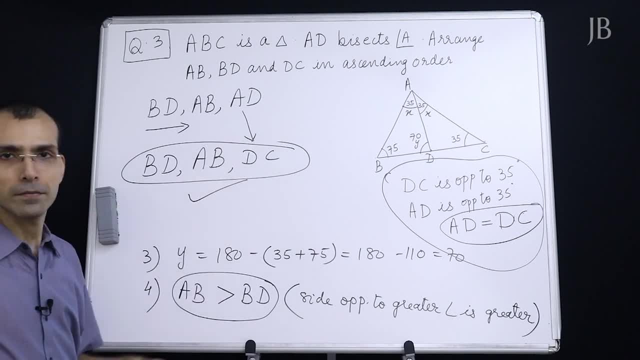 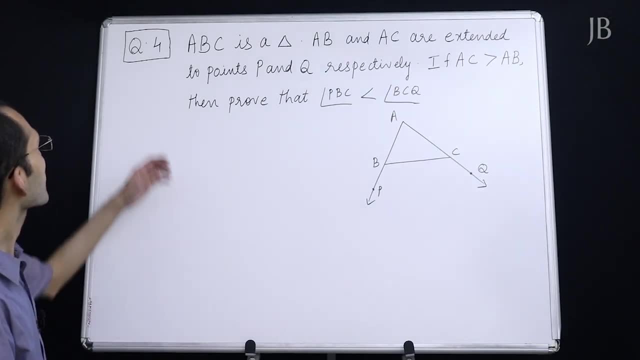 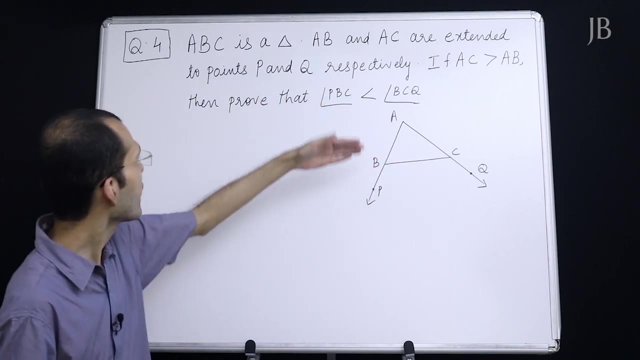 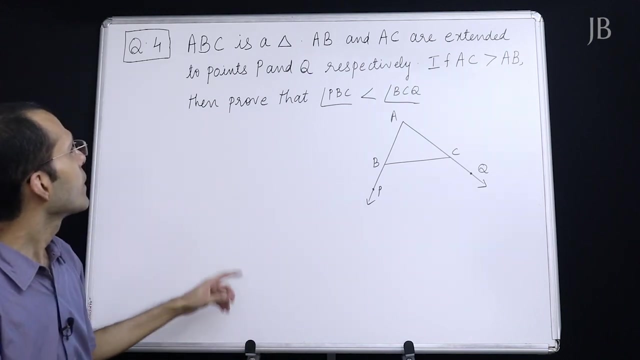 answer now, Ascending order, Comfortable with this. This completes with your question 3.. Question 4.. ABC is a triangle. AB and AC are extended to points P and Q respectively. Extended means pulled straight. Ok, if AC is greater than AB, then 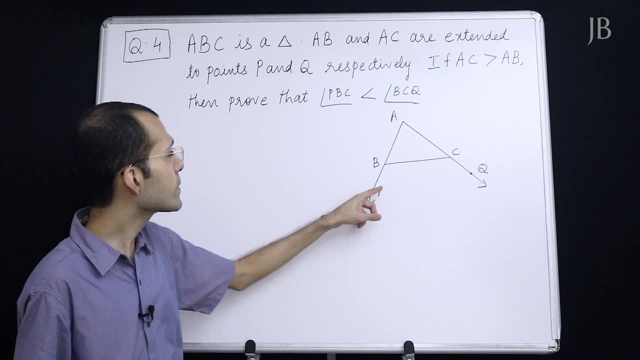 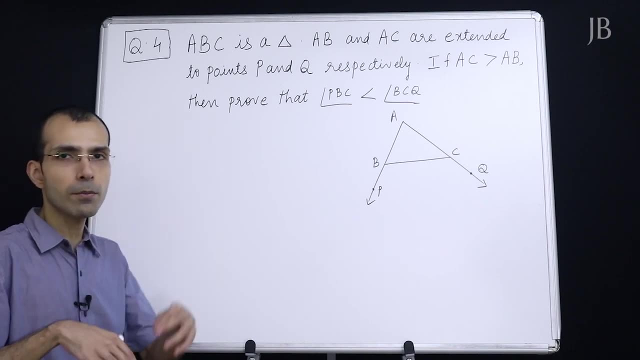 prove that angle PBC is smaller than angle BCQ? A different question. So far what was happening is we were proving this side greater than the other side or this side is smaller than the other side. Here, information about the sides is given to you. You have to prove some. 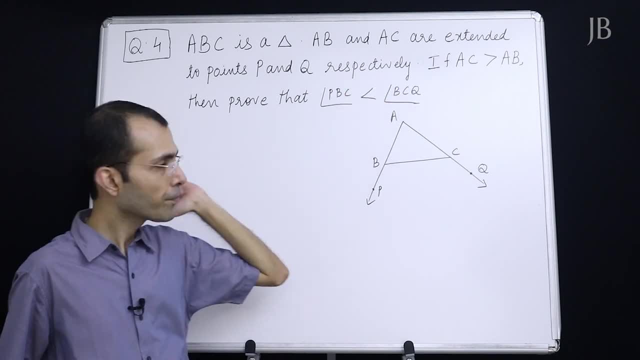 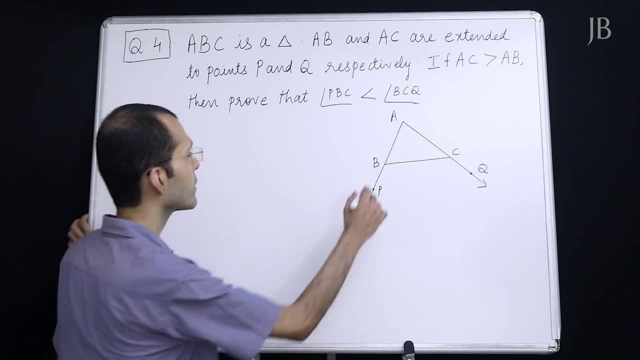 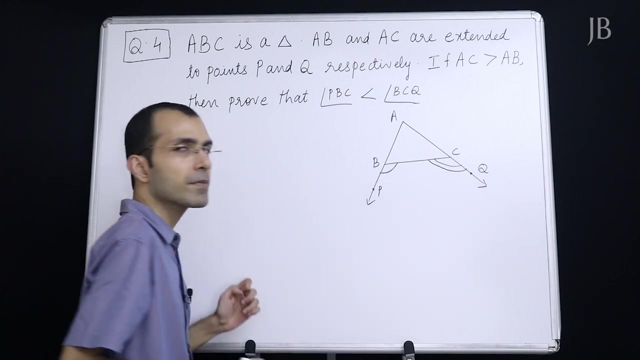 angle smaller than another angle. Ok, now if you look at angle PBC, it is going outside like: this is your angle PBC and this is your angle BCQ. So the problem is it becomes difficult to apply the property directly, Like see, if I want to prove some angle smaller. 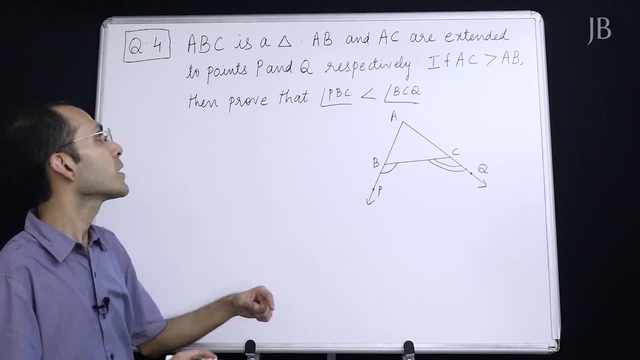 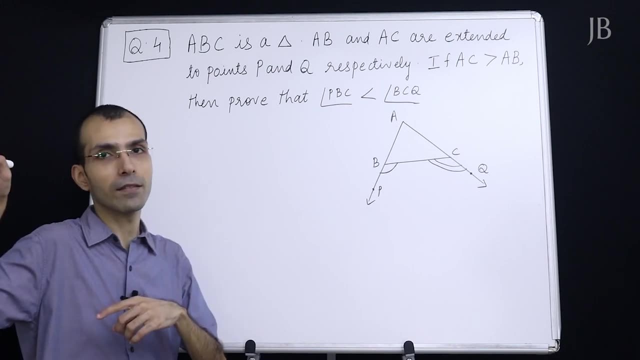 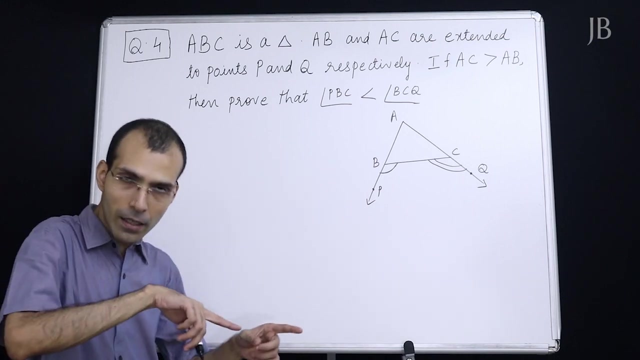 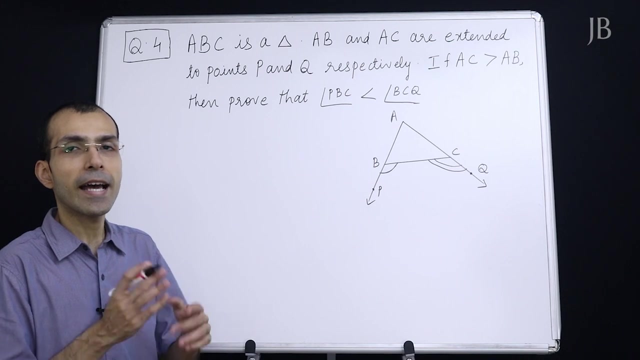 than the other, then I will have to prove the side opposite to that angle smaller than the side opposite to other angle. If we can prove one side smaller than the the other side, then the angle also will be smaller. It's like that concept, which is that concept: angle opposite to greater side is greater, or angle. 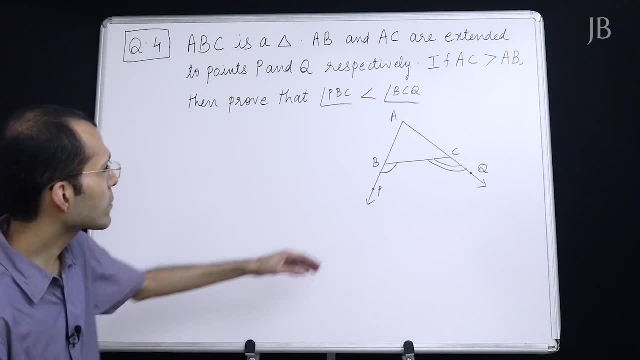 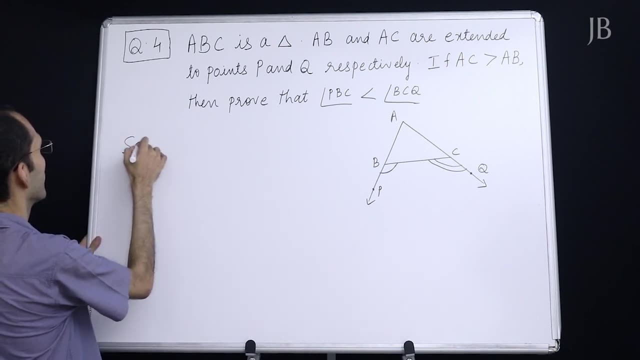 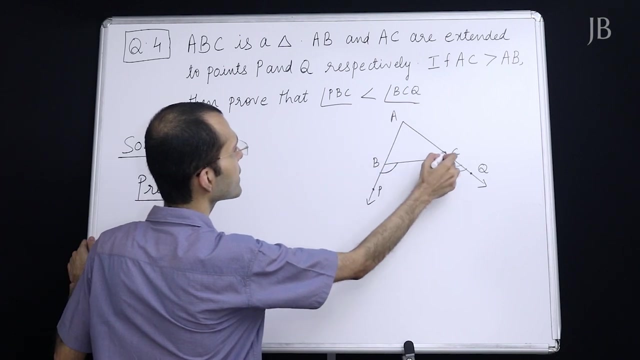 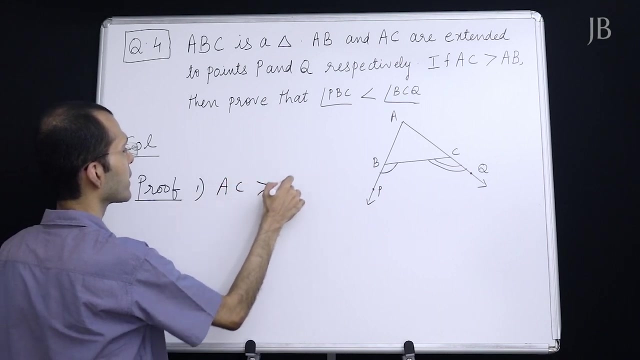 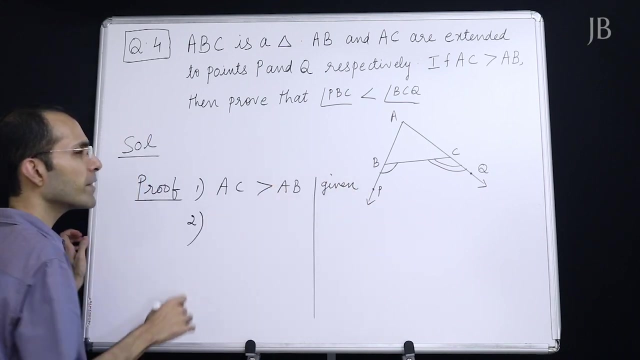 opposite to smaller side is smaller. But this is going outside. How do we do So? we'll have to go in an indirect way. Proof: Okay, they have given you AC greater than AB. This is given, AC greater than AB Given. So what can we conclude about the angle? 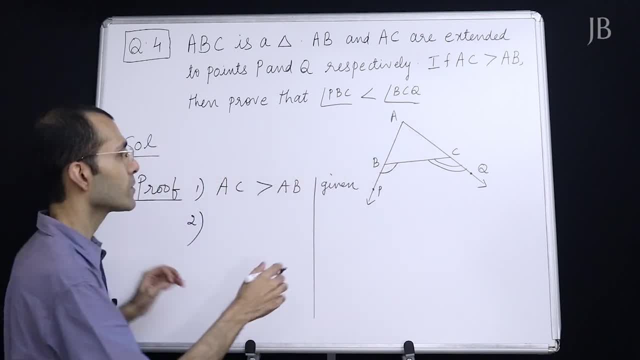 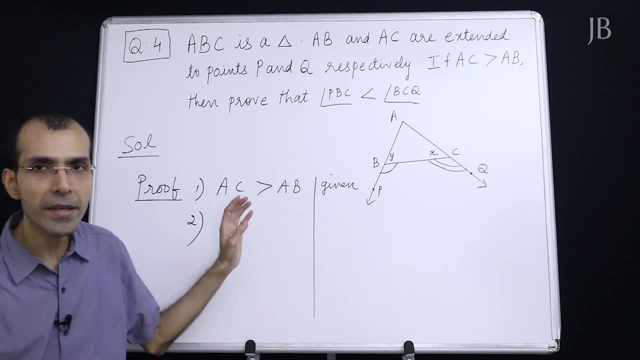 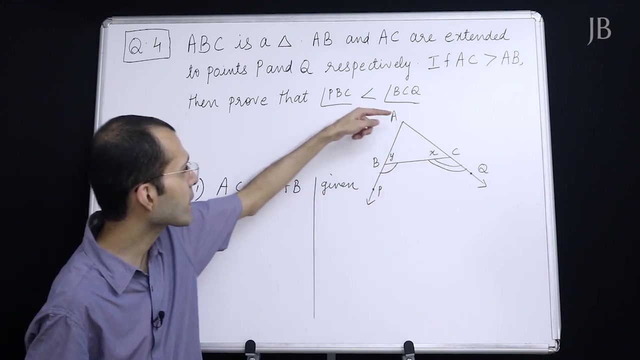 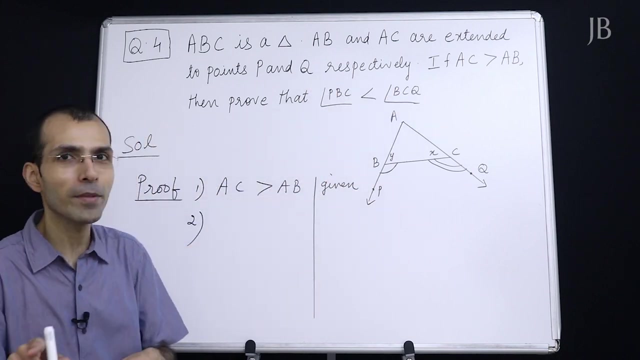 which is inside the triangle ABC. So let this angle be, say, X and this angle be y. It is very clearly mentioned that AC is greater than AB. If AC is greater than AB, then the angle opposite to AC also will be greater, then the angle opposite to AB. So AC is greater. 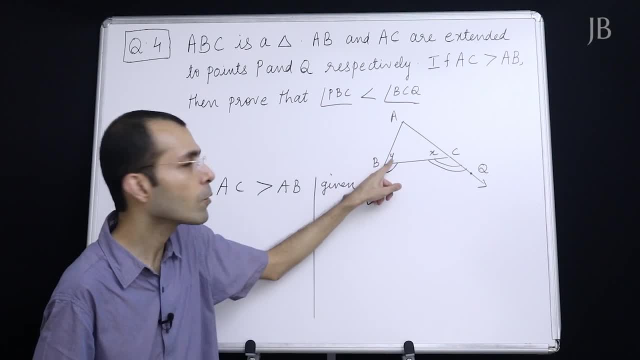 than AB. So which is the angle opposite to AC Y And which is the angle opposite to ABZ, Right Between these, and this angle is greater than AC. for Z, The opposite angle be x. And what has been told to you, AC is. 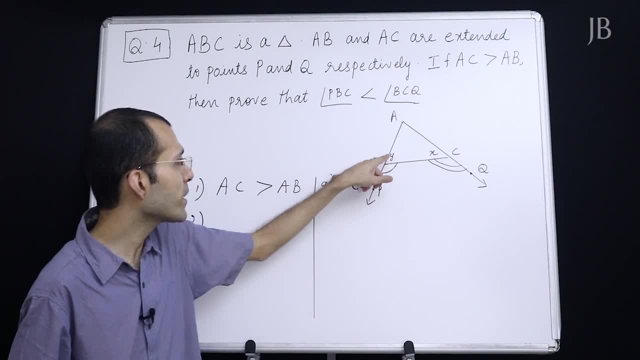 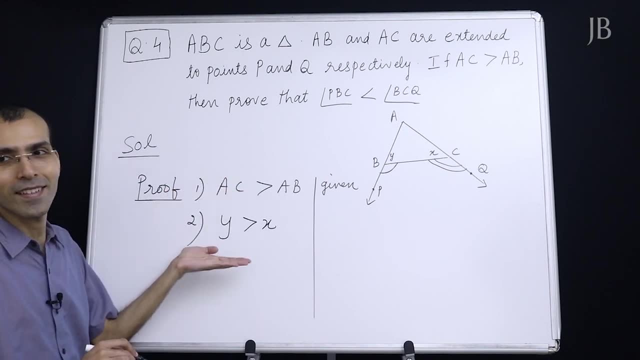 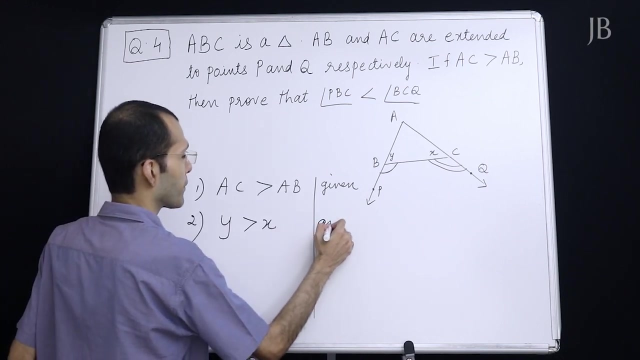 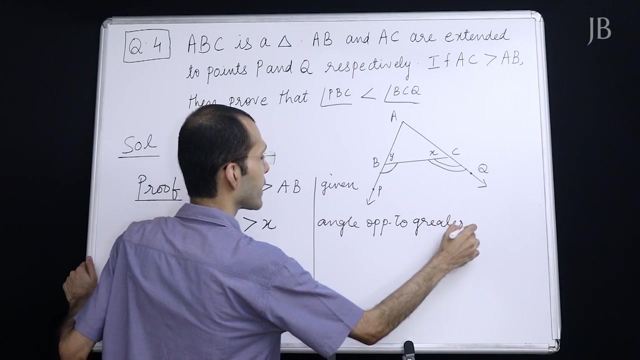 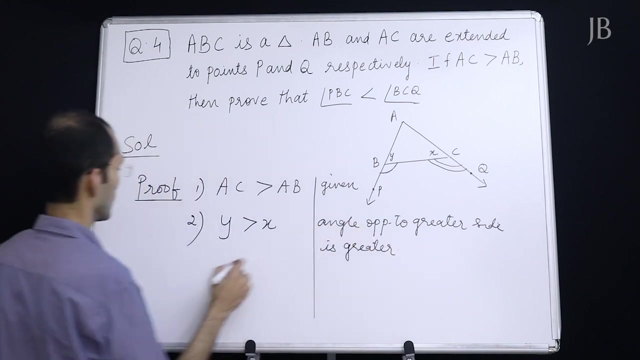 greater than AB. So, which is the angle opposite to AC, Y. So Y will be greater than x. As a consequence of this, what is the reason? Angle opposite to greater side is greater. Angle opposite to greater side is greater. Ok, so now Y is greater than x. 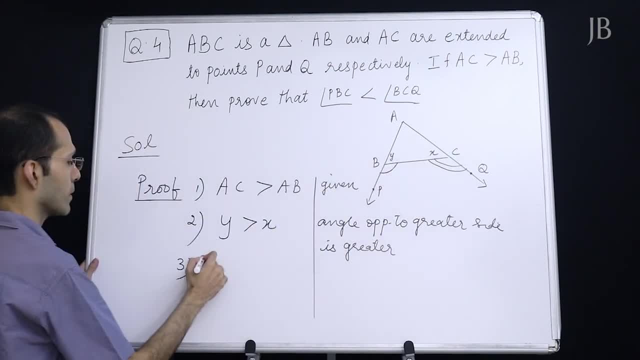 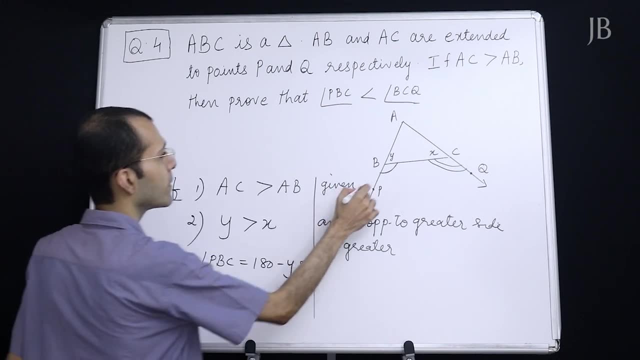 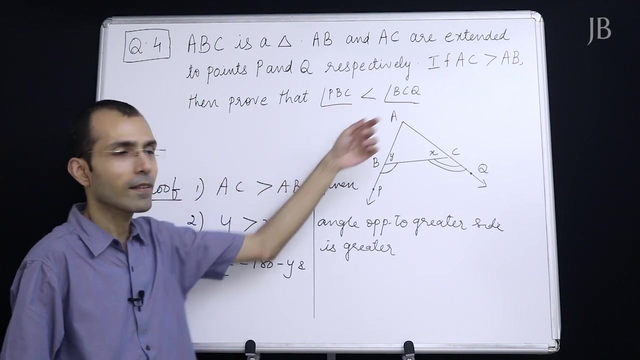 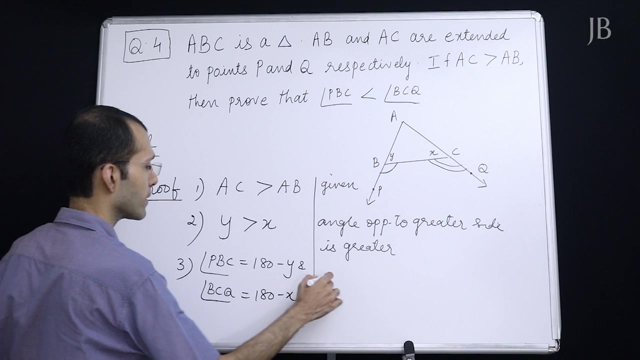 Now look at angle PBC. Angle PBC will be how much 180 minus Y Linear pair, And what will be angle BCQY? We are finding all these angles because they are required. in question, An angle BCQ will be 180 minus x, The. 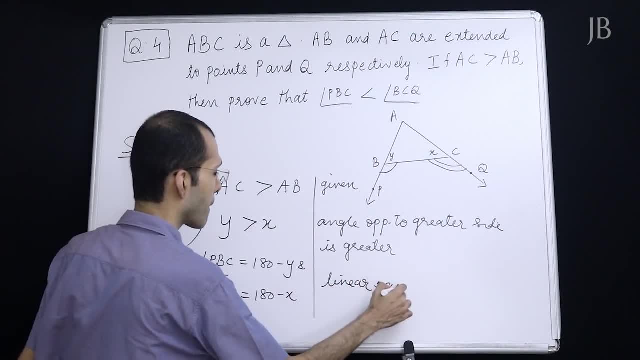 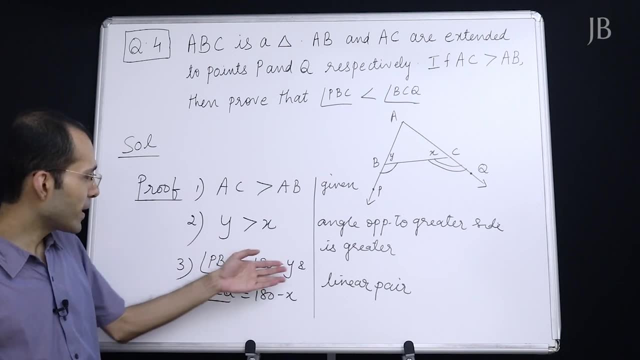 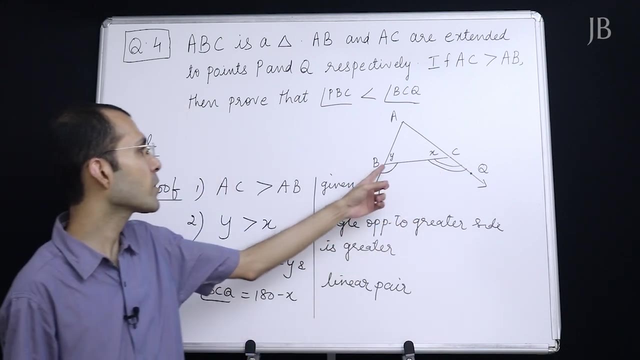 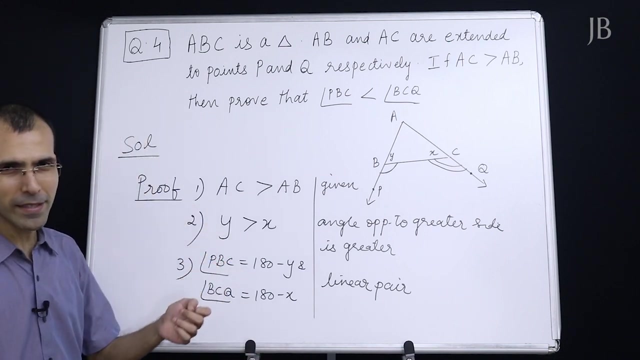 reason is linear pair. We are almost done now. See, PBC is 180 minus Y and BCQ is 180 minus x. We just have to compare these two angles Now. who will be greater? Ok, think like this. Let's take an. 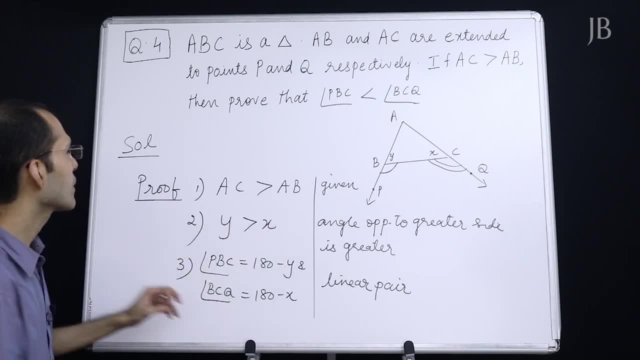 example Y greater than x. So let's take something like 30 greater than 20.. Agreed, Nothing wrong in this: Y greater than x. So let Y be, say 30 and x be 20.. So 30 is greater than 20.. Now we do 180. 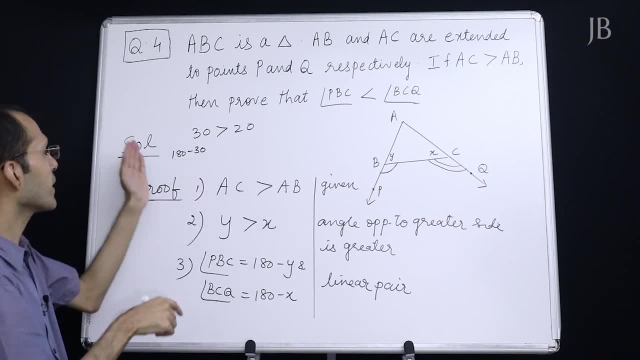 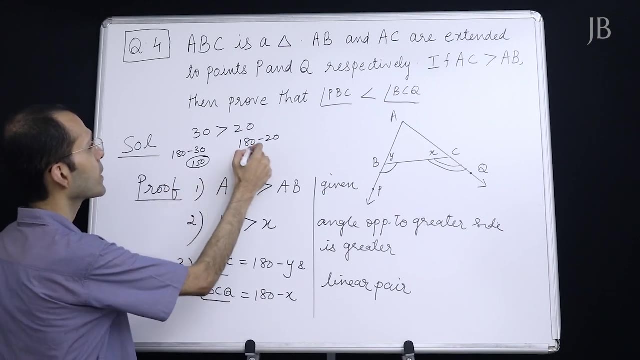 minus 30.. Not 30 minus 180.. 180 minus 30.. And this side we do 180-30.. And this side we do 180-30.. And this side we do 180-30.. So what happens? 180 minus 30 gives you 150 and 180 minus 20 gives you 160. 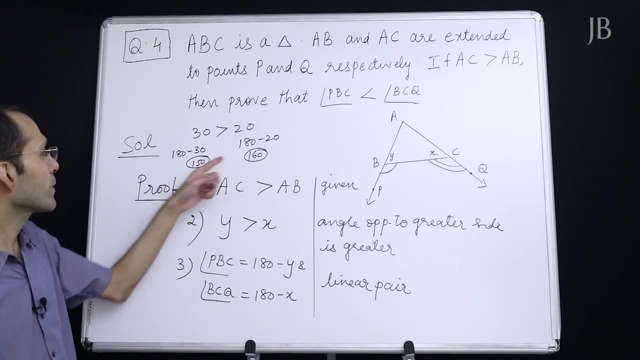 Now, who is greater, 150 or 160?? 160 is greater, So inequality will go like this: The open mouth will go towards 160. Automatically, inequality has reversed. We have not done any manipulation. 30 greater than 20? Agreed. Now I do 180 minus 30 and here I do same. 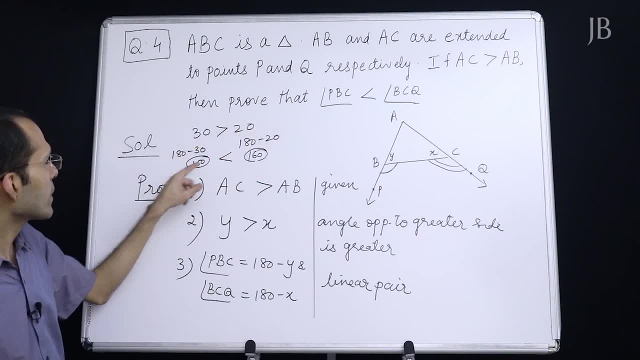 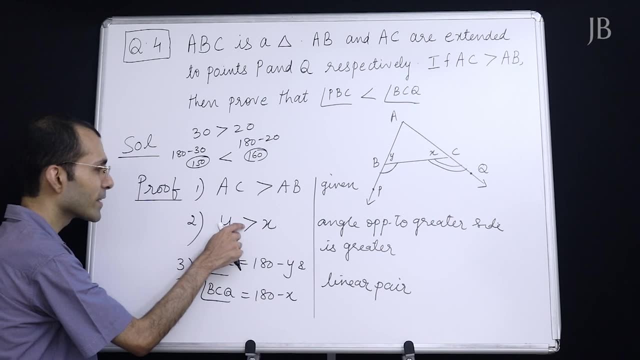 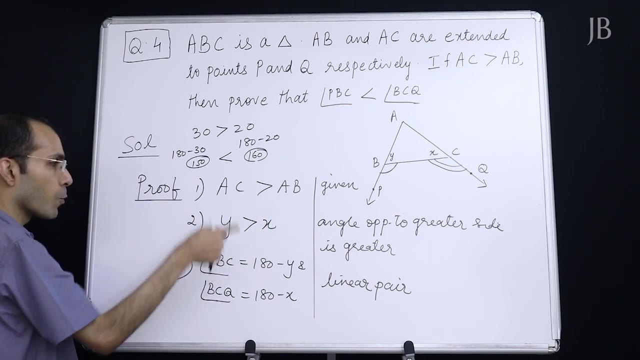 180 minus 20.. So this becomes 150 and this becomes 160.. So inequality reverses. So now here, y is greater than Now. connect this funda to this general thing: y is greater than x. So 180 minus y on this side and 180 minus x on this side. 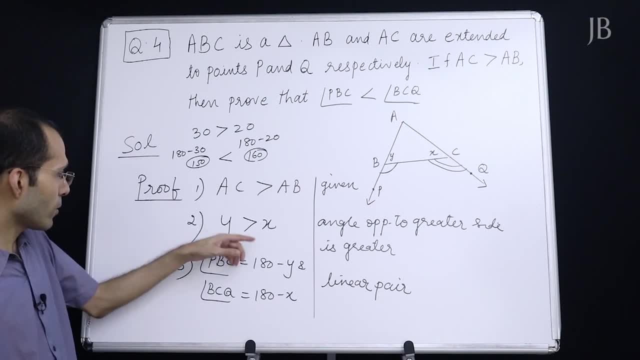 So who will be greater now, 180 minus y or 180 minus x? Ulta, 180 minus x will be greater, So here it will be 180 minus y lesser than right, because inequality reverses. So 180 minus y. If y is greater than x, then 180 minus y will be less than 180. 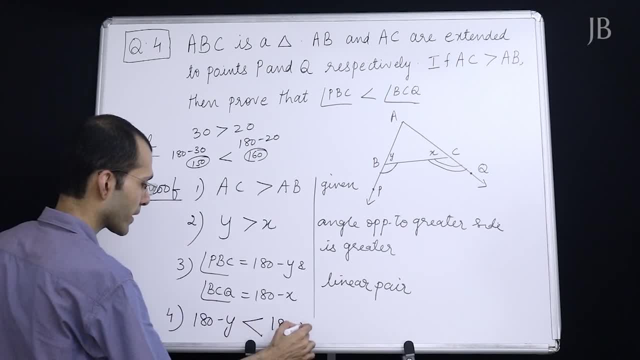 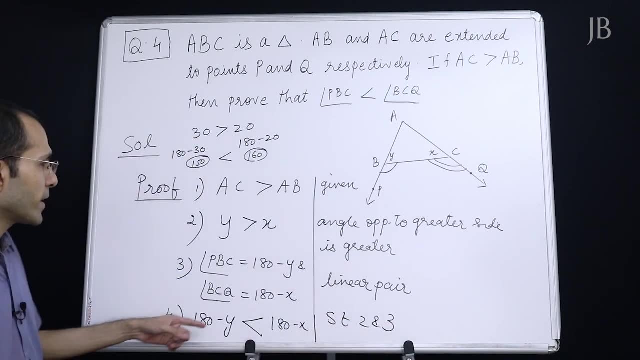 180 minus y will be less than 180.. Then 180 minus x. Here we will write statement 2 and 3.. But what is 180 minus y- Angle PBC and what is 180 minus x- Angle BCQ? 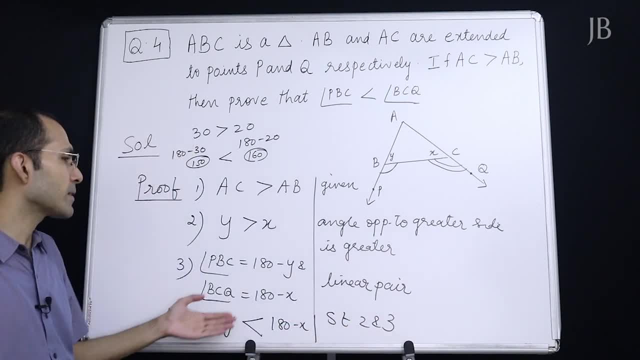 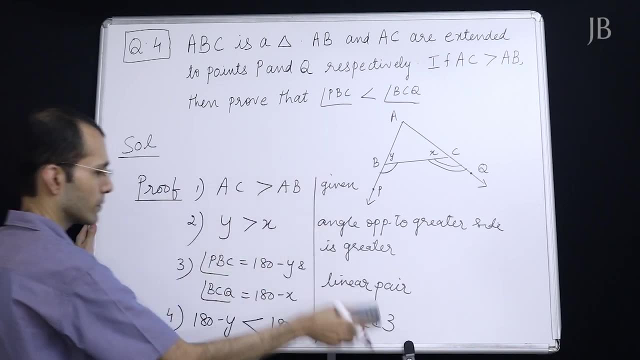 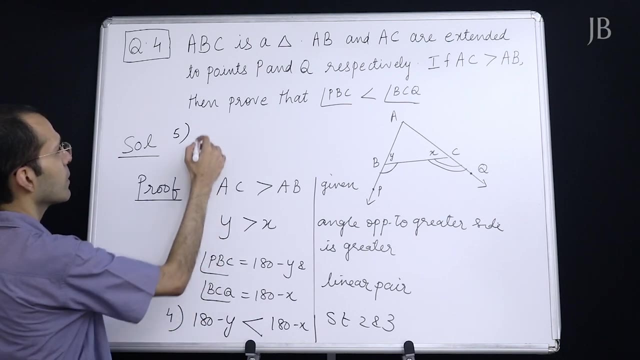 So we have successfully proved that angle PBC is lesser than angle PCQ. So let's put it here formally: So 180 minus y will result in angle PBC And the inequality will automatically reverse because of the reason which I have just now showed you. 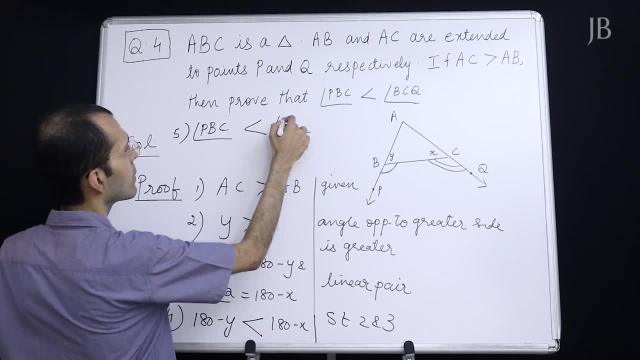 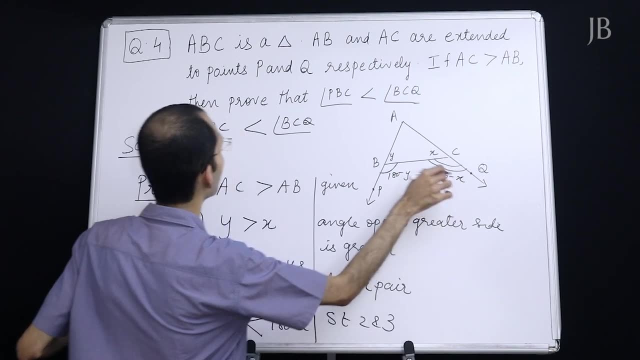 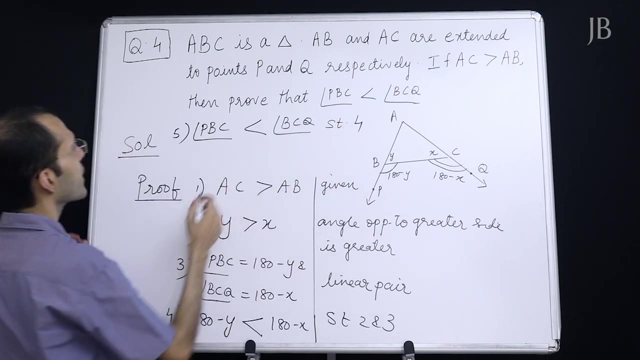 And 180 minus x represents angle BCQ. Here the reason will be statement 4.. And that is what we wanted to prove. We wanted to prove angle PBC lesser than angle BCQ, Hence proved. This completes with your question 4.. 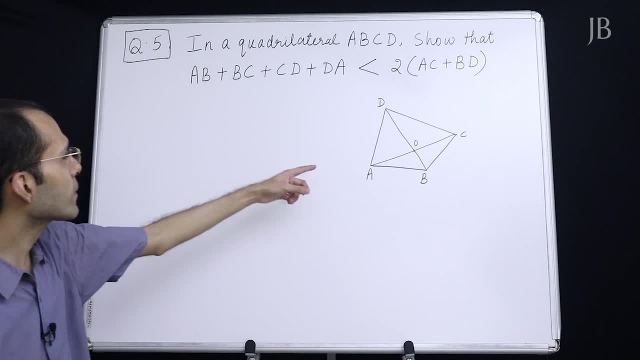 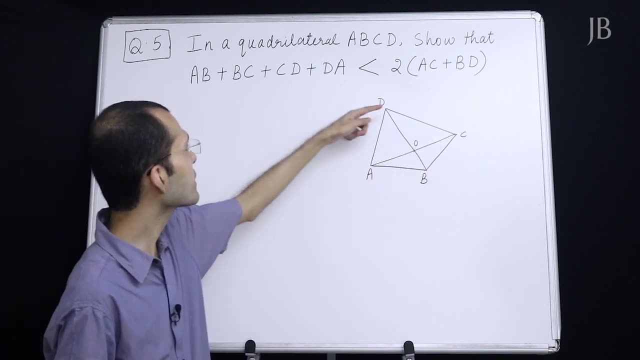 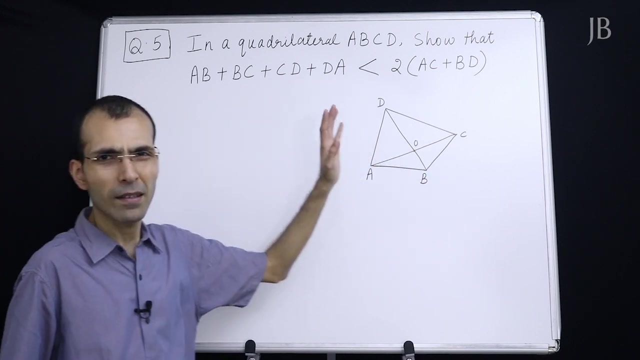 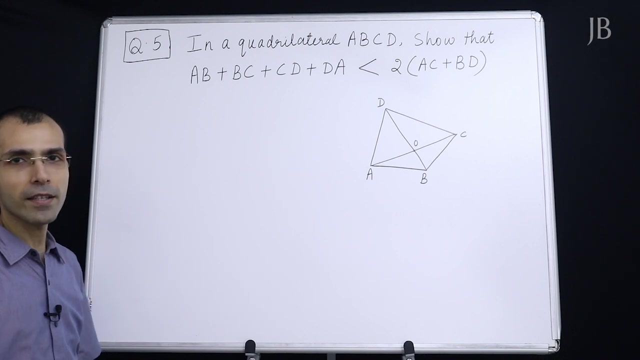 Question 5. In quadrilateral ABCD show that AB plus BC plus CD plus DA is lesser than twice of AC plus BD Appears bewildering. but nothing of that sort. We have studied the triangle inequality So that only somehow we have to apply. 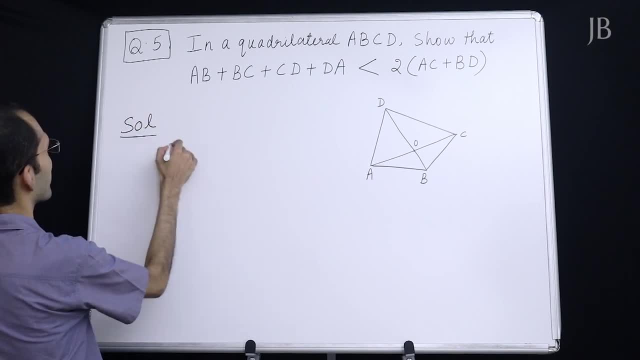 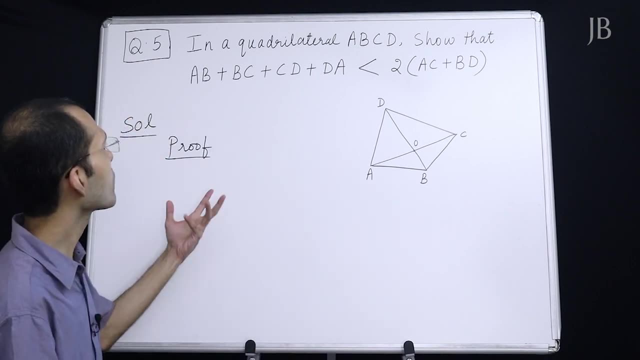 Okay, Now here no information is known about the angles and all That means, most probably the triangle inequality will come in the picture That is sum of two sides. Sum of any two sides of triangle is always greater than the third side. Fine, 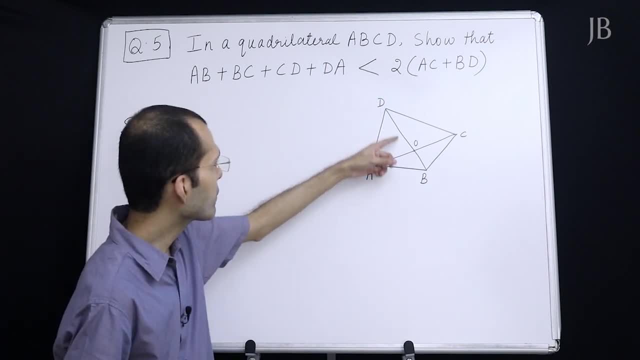 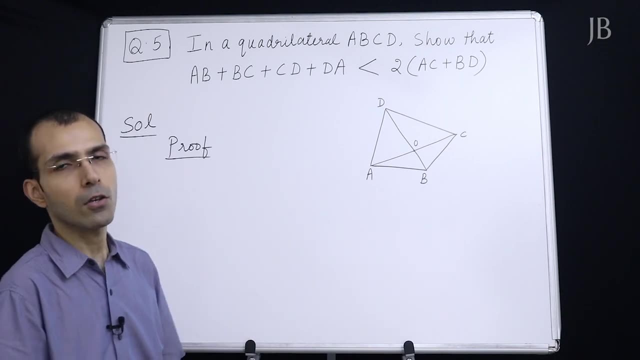 So let us see how to start with now. We can have, we can see so many triangles: DOC, COB, AOB, DOA. That is good. So we can apply some concept which we have been taught. They want AB, BC. 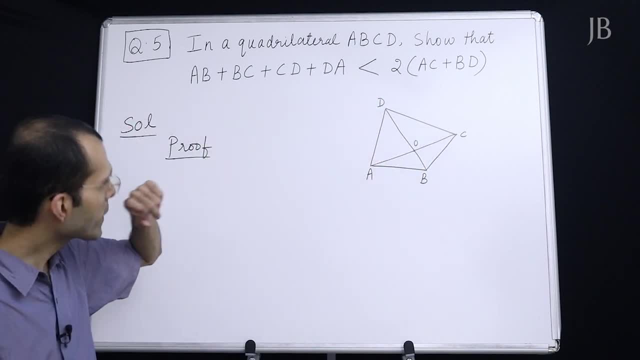 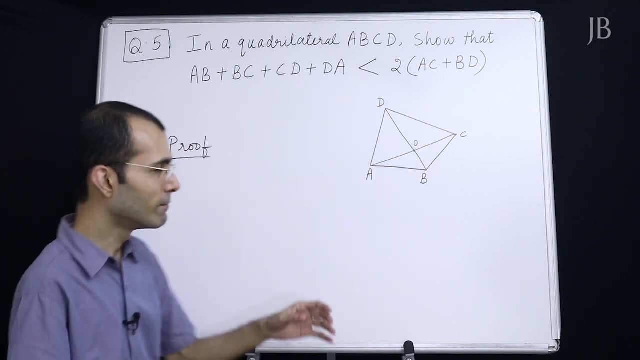 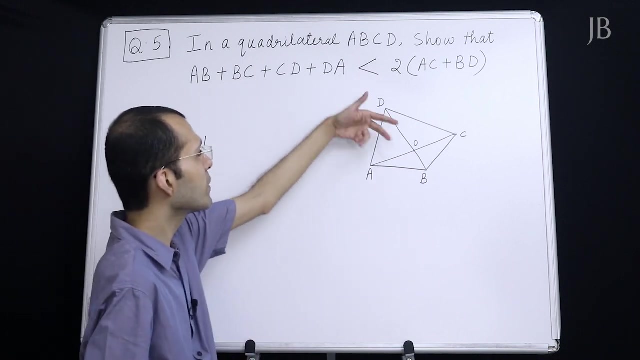 AB BC CD DA Outer side. Okay, So what we will do, We will try to keep AB BC CD DA on one side And then simply add them, Because the question says add Okay. And how this two comes, we will see. 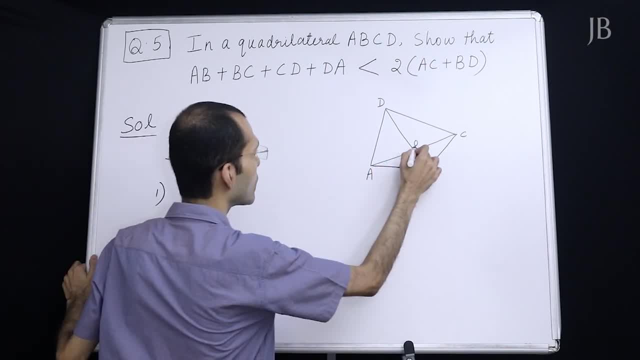 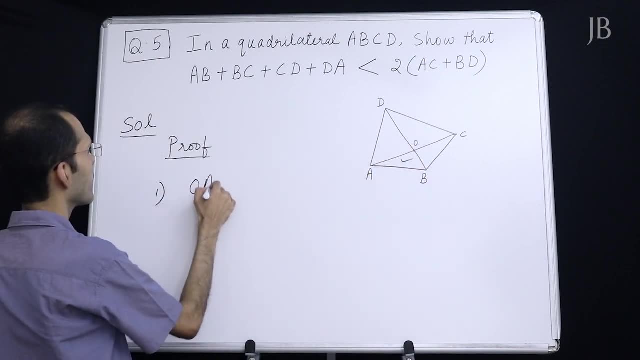 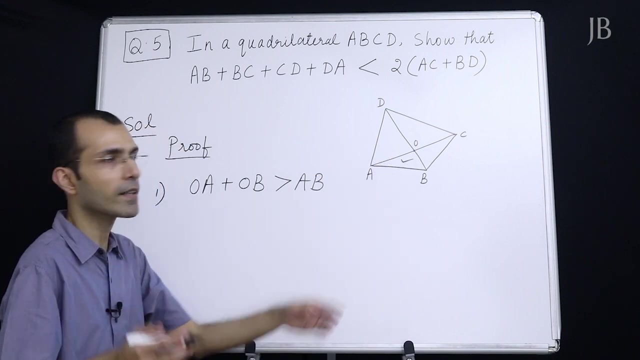 First step. Consider triangle OAB. Consider triangle OAB. So OA plus OB will be greater than AB. Do you agree? OA plus OB will be greater than AB. Sum of any two sides of a triangle is always greater than the third side. 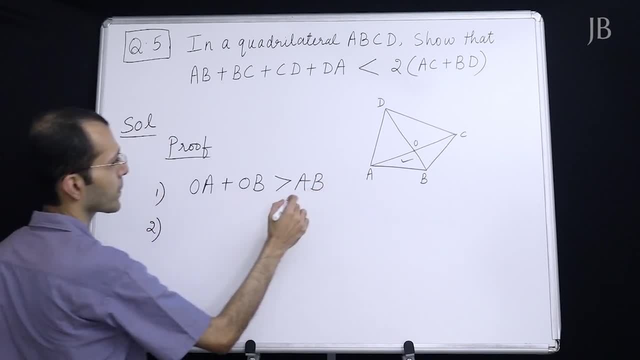 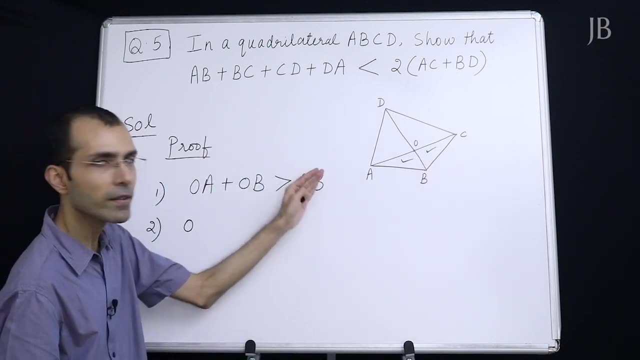 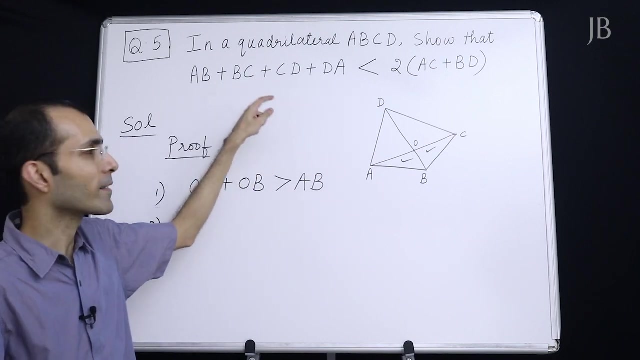 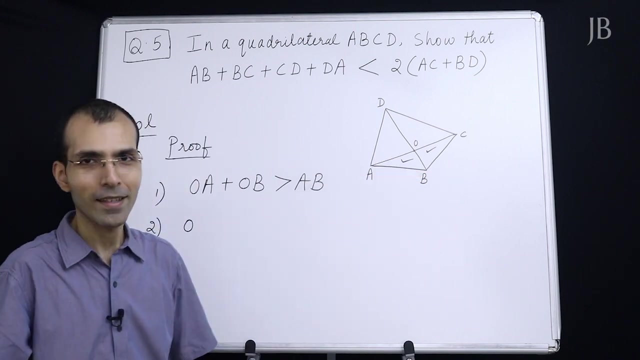 So that reason you will have to write it Now. consider this triangle: OB, keep AB on this side And even BC on this side, CD on this side, Because we want to add all of them. So it is easier. That way, if you see, AO plus AB will also be greater than OB. 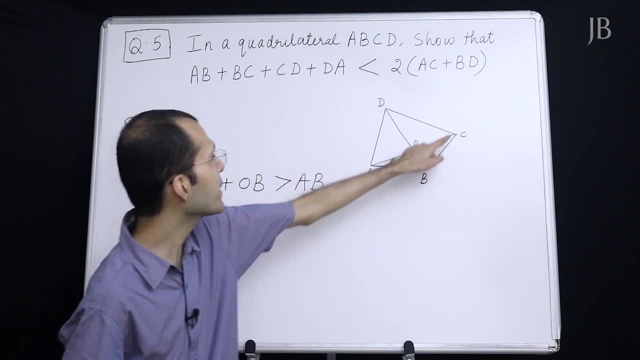 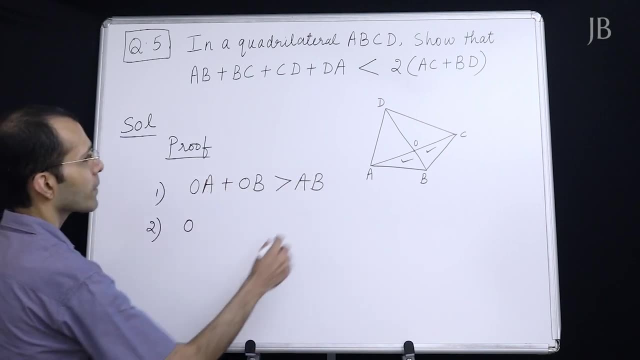 But don't do that. You try it, Because look at the question: AB, BC, CD, DA, And we want to add everything. So keep everything on one side. only Now, here in this triangle: OCB, OC plus OB. 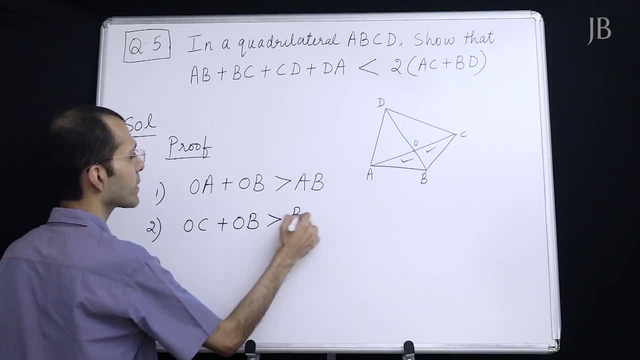 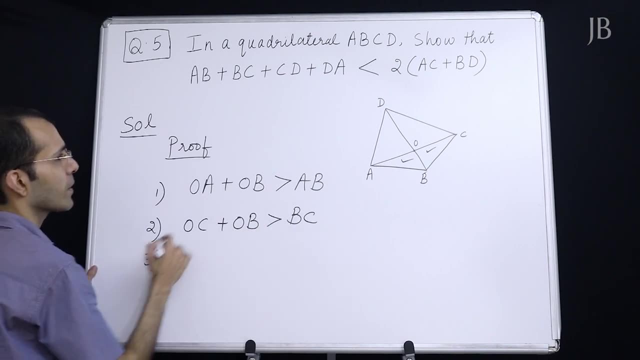 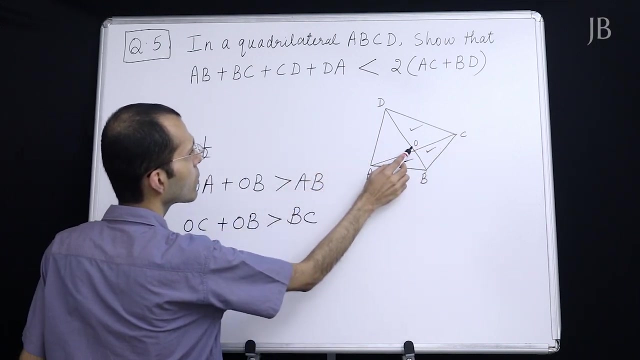 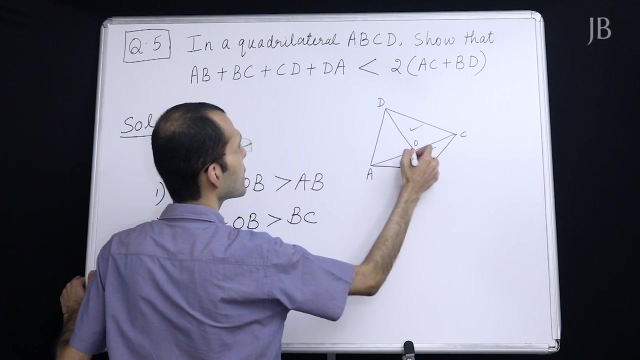 OC plus OB will be greater than BC. So we have kept BC on this side. only You know what is required in the question. Now we consider this triangle OC, We take triangle DOC, So it will be OC plus OD, OC plus OD. 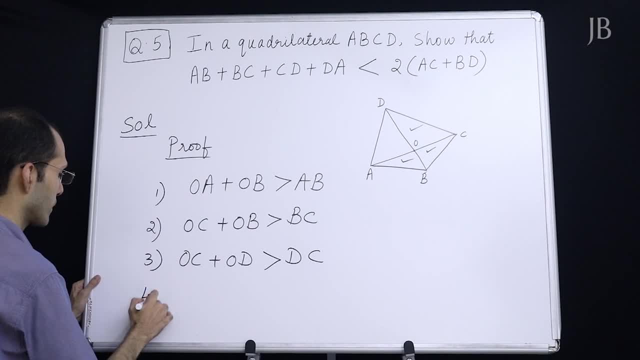 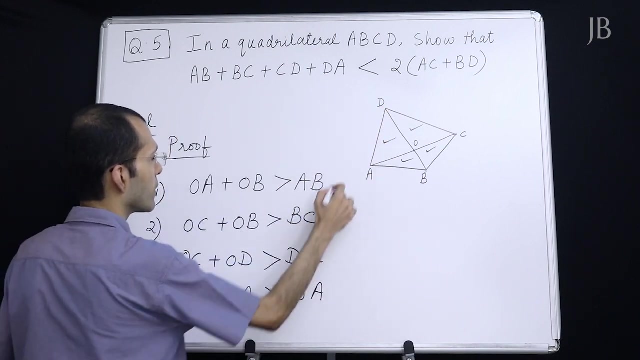 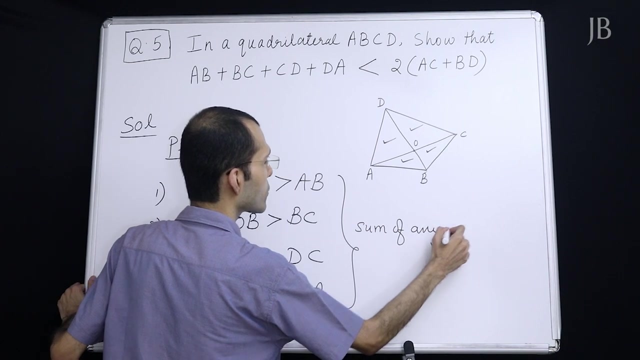 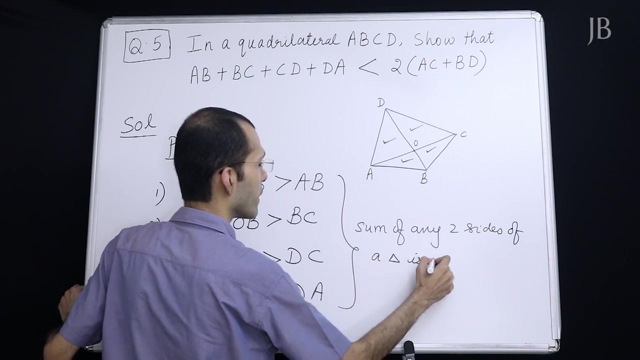 Will be greater than DC. Now take this triangle. It will be OD plus OA. OD plus OA is greater than DA. The common reason for all this will be what Sum of any two sides, Sum of any two sides Of a triangle, is greater than the third side? 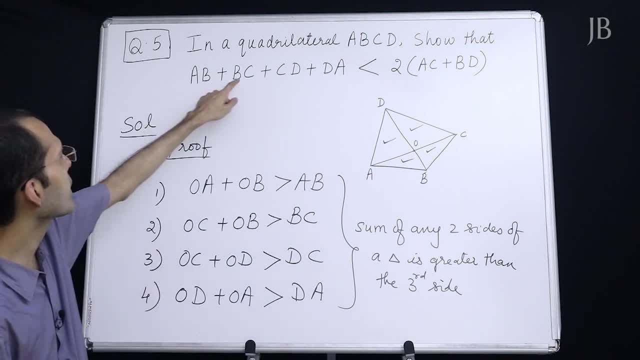 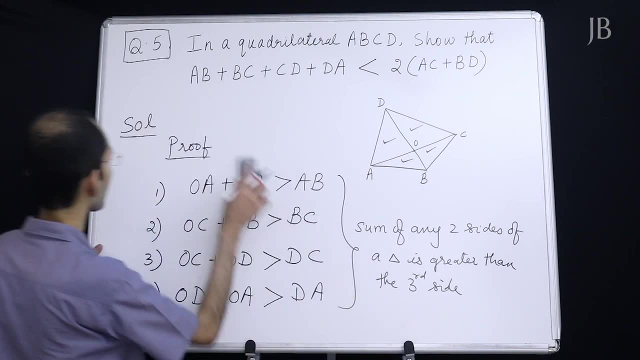 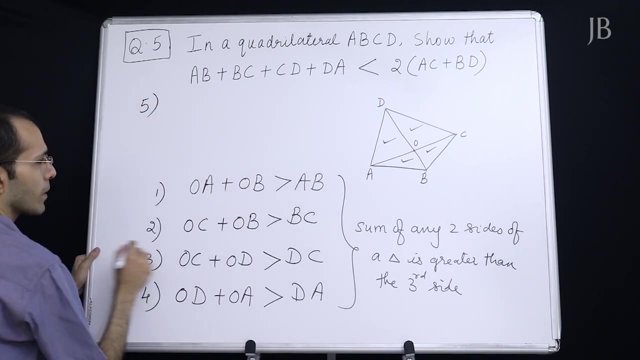 This is okay, Direct application. Now, what they want: AB plus BC plus CD plus DA. Since they want the addition, We will simply add all of them. Add all of them. So now what will happen is So, if we add this side, 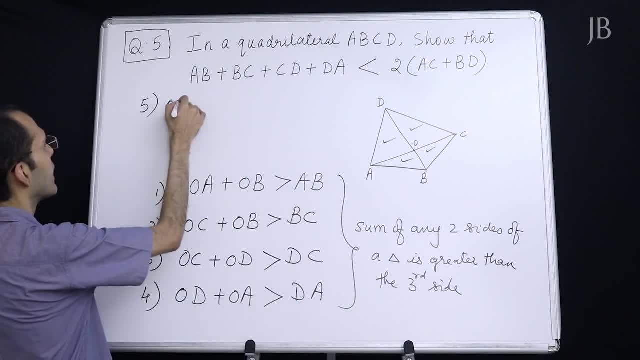 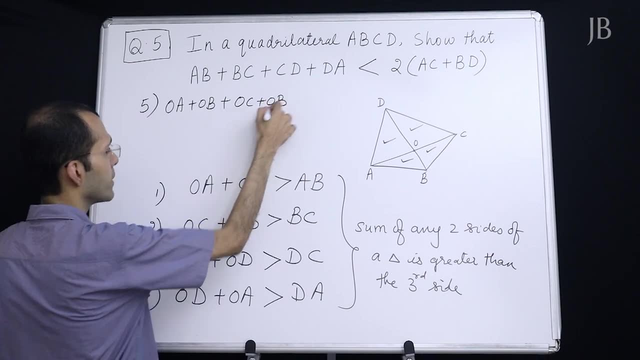 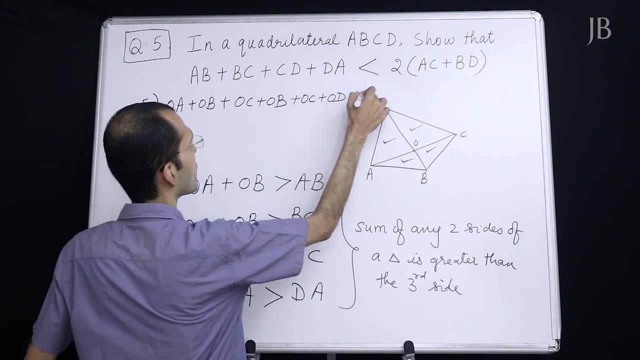 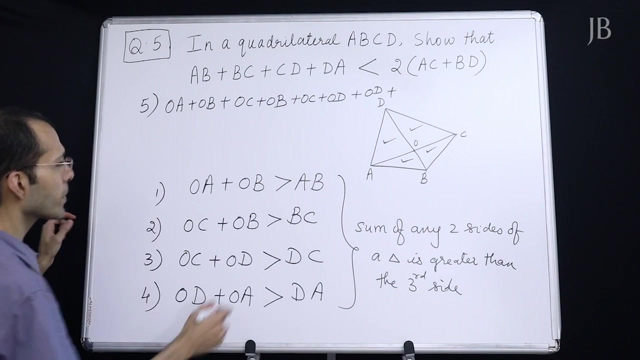 Even this side will get added. So we will have OA plus OB Plus OC plus OB Plus OC plus OD Plus OD plus Where it is there, 2,, 4,, 6. OD plus OA Will be greater than. 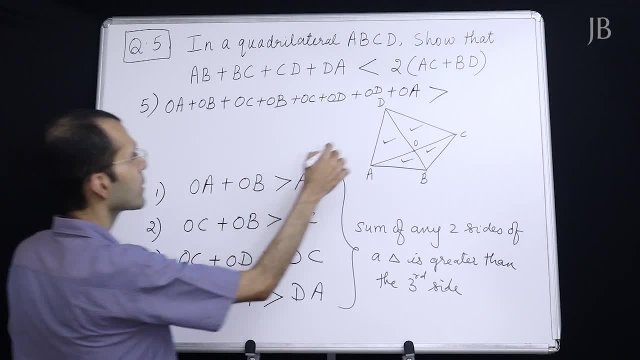 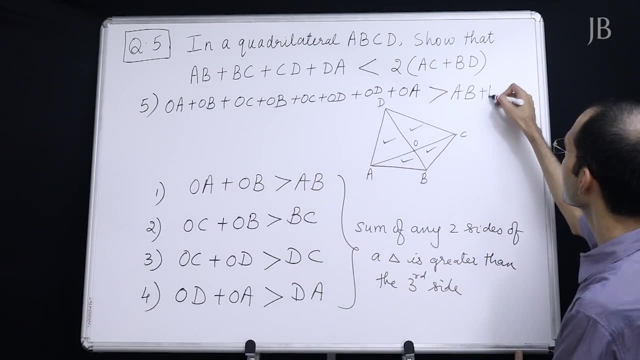 We add up everything. Here also, we add up everything. So here we will have greater than AB plus BC plus DC plus DA. Here the reason will be statement 1,, 2,, 3 and 4.. We have simply added everything. 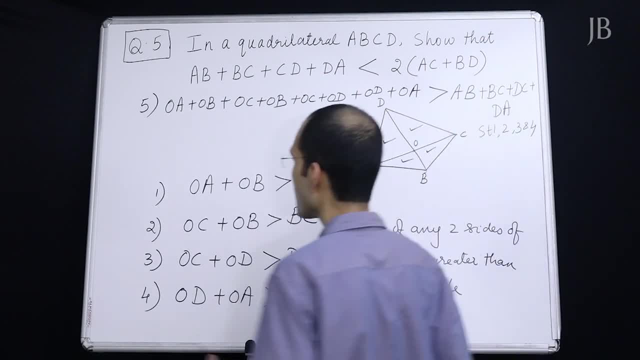 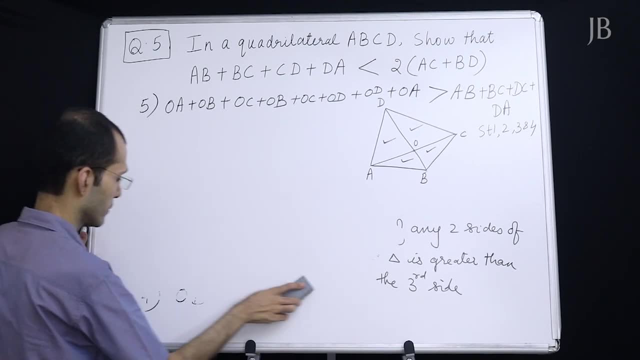 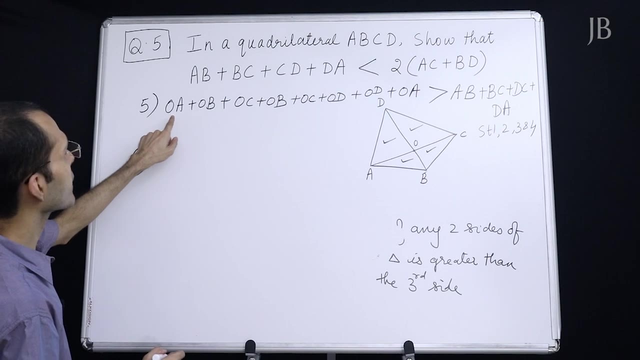 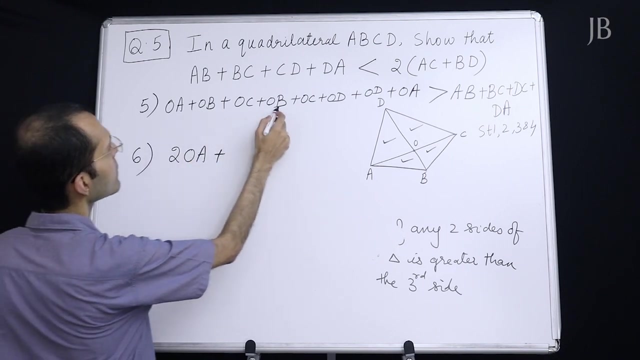 Because the question demands. so Let's see, This is OA plus OA. We will get 2 OA, Then OB plus OB. So this we have considered, Then OB plus OB gives 2 OB OC. So this is taken care of. 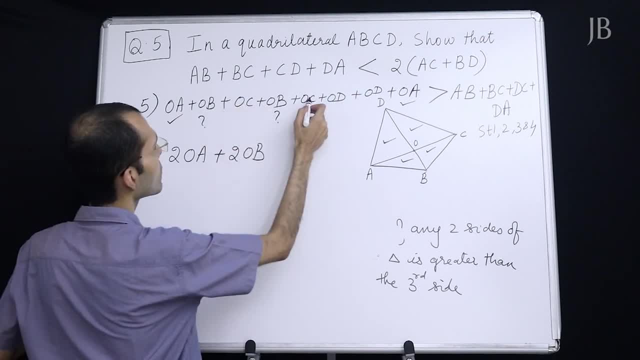 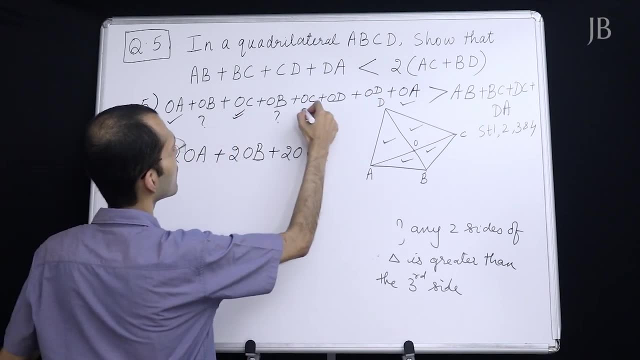 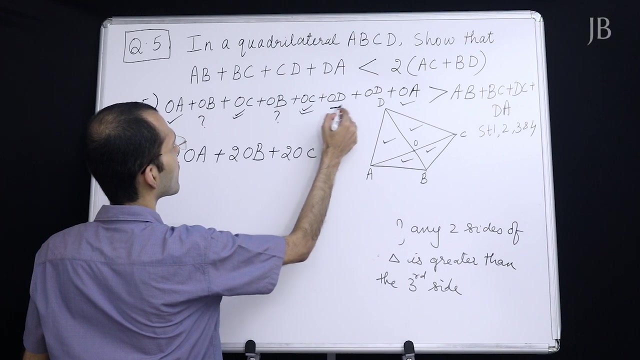 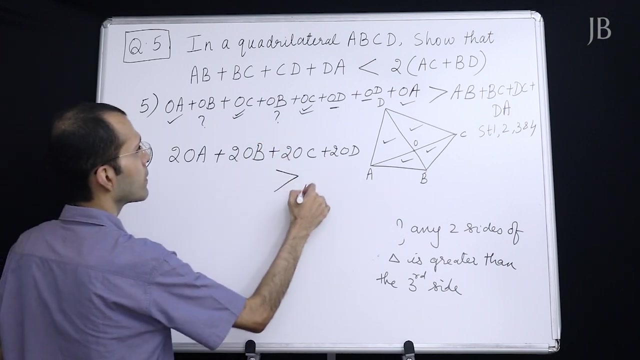 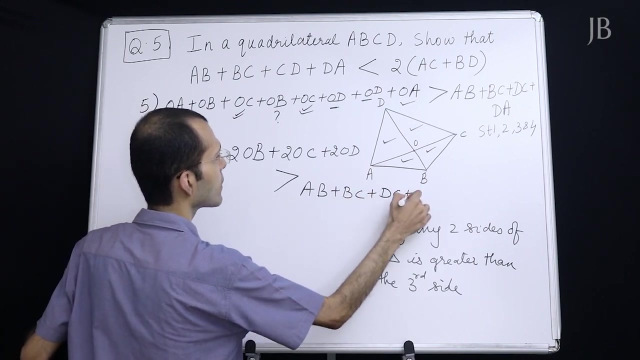 OB and OB. OC plus OC gives 2 OC. This is again taken care of. And what is remaining now? OD plus OD. Yeah, OD and OD That gives you 2 OD Is greater than Same AB plus BC plus DC plus DA. 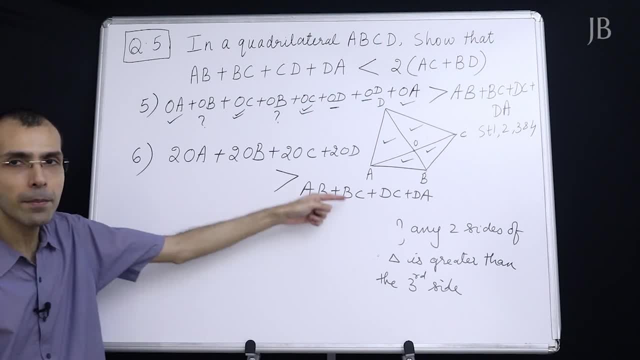 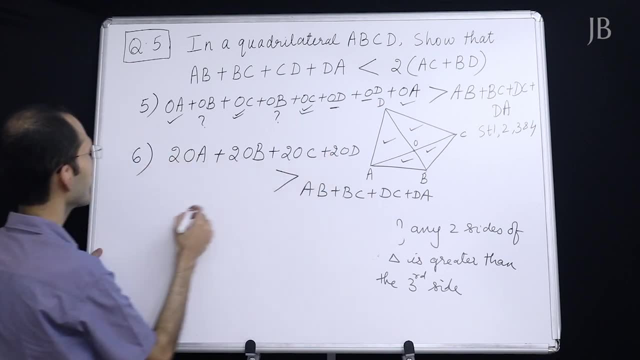 Okay, Now we need little more refinement, Because we have got AB plus BC plus DC plus DA. This much too has come Here. we have to work out something Here. if you see, We can take 2 common, We can take 2 common. 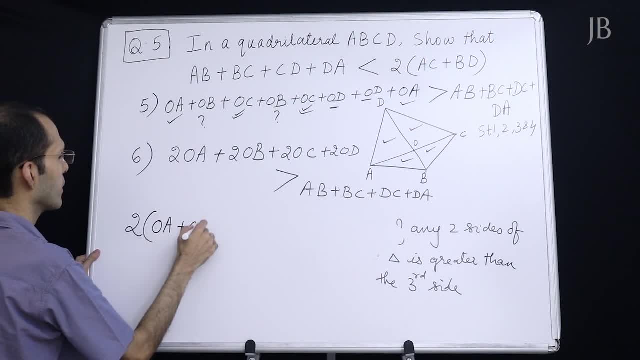 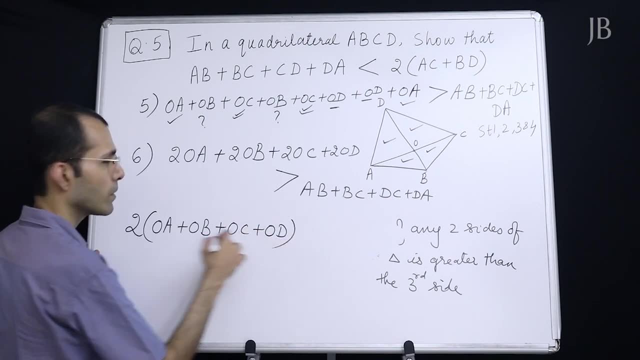 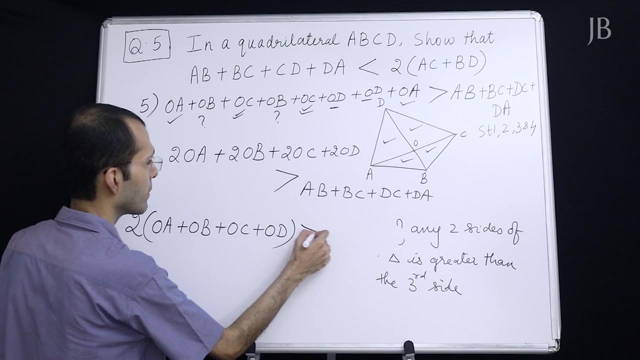 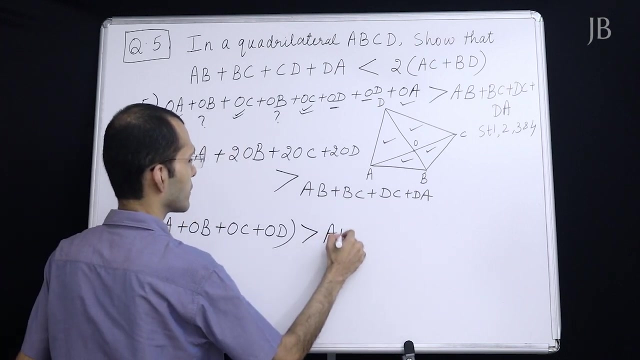 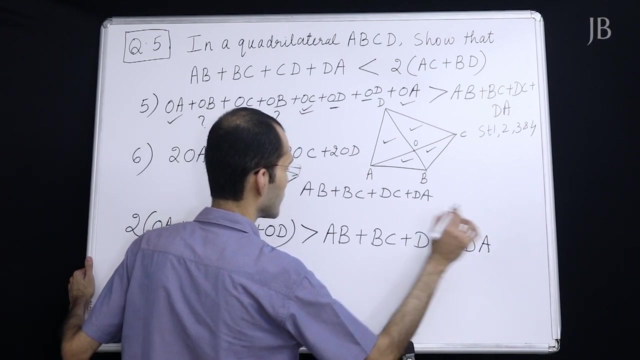 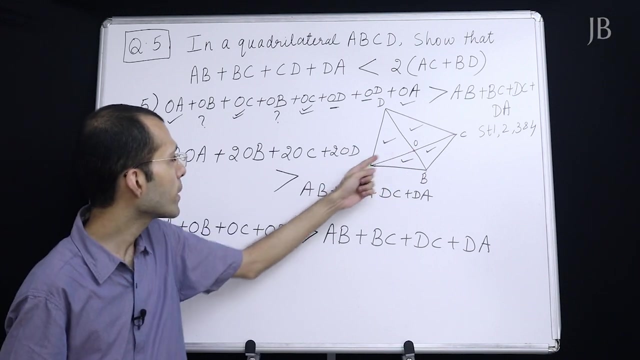 So this will be OA plus OB plus OC plus OD. We can take 2 common OA plus OB plus OC plus OD Will be greater than So. this will be AB plus BC plus DC plus DA. Okay, Now observe OA plus OB. 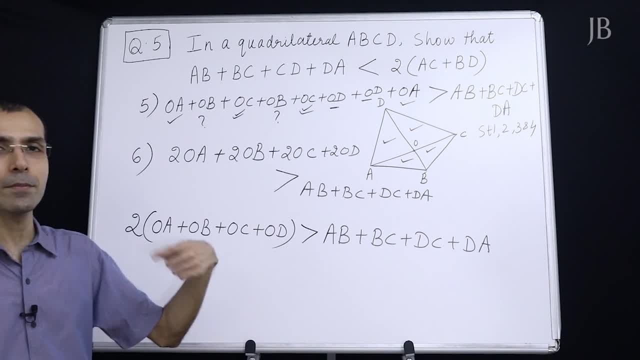 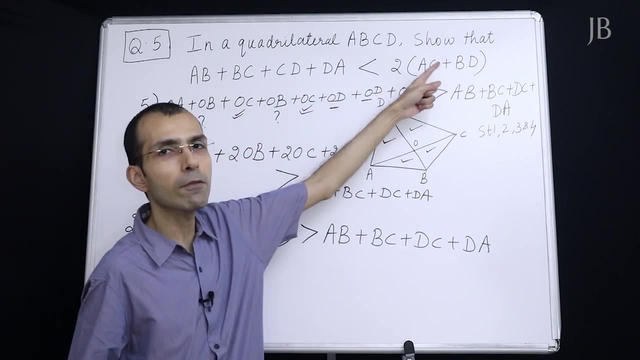 OA plus OB- Okay, No problem. Plus OC, plus OD- Is something striking your mind? We have got this Already. So here We want a small thing. We want AC plus BD 2 we have already got That means, certain segment should get added. 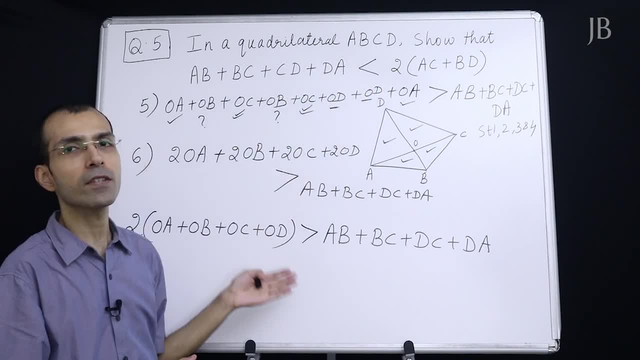 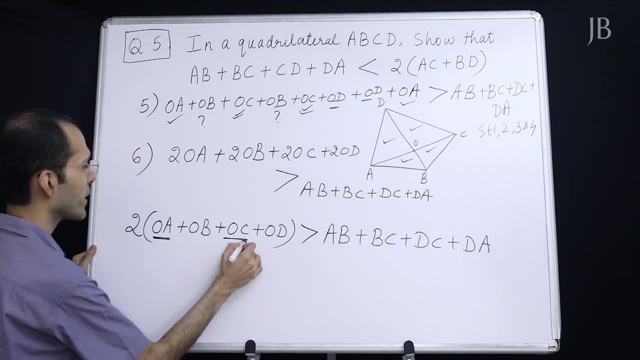 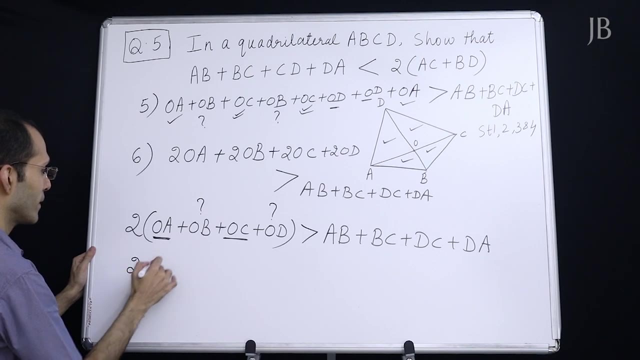 So by looking at the question We get an idea what is to be done. Now see, We want AC Right. So If you take OA And if you take OC, You take OA and OC And you take OB with OD. 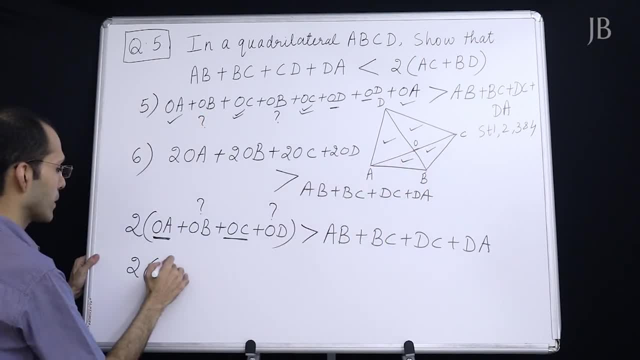 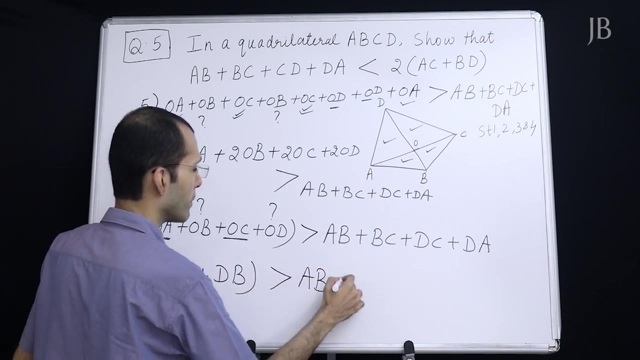 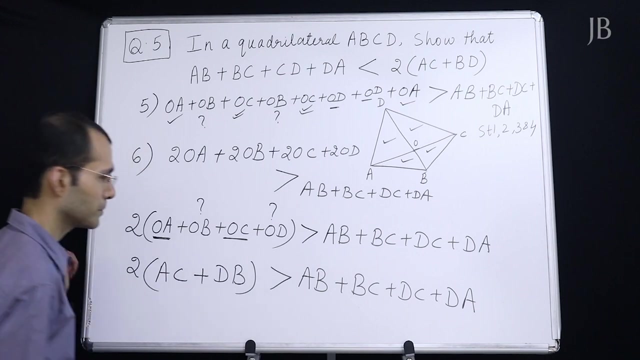 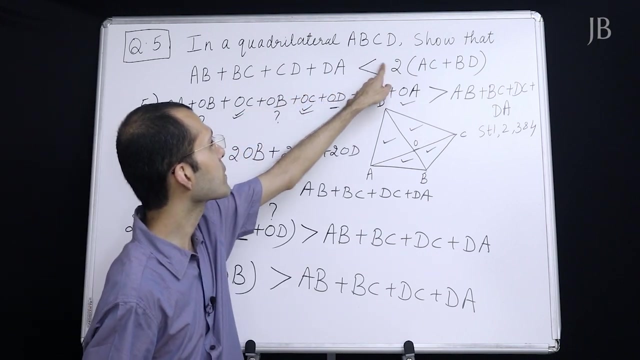 So OA plus OC Gives you AC And OB plus OD, OB plus OD Gives you DB. This is greater than AB plus BC, Plus DC Plus DA. And same thing we had to prove. See, Open mouth is towards. 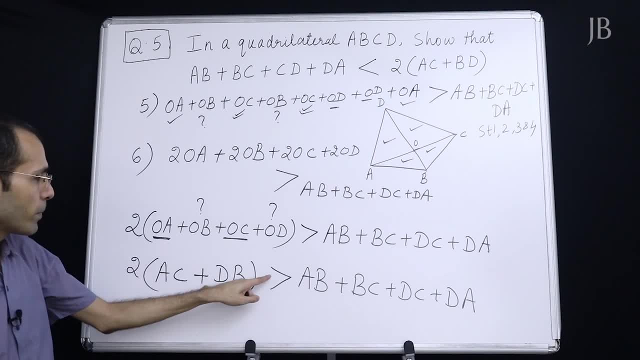 Twice AC plus BD. Here also the open mouth is towards twice AC plus DB, Just that It is in a different form, Like X greater than Y Or Y less than X. One and the same thing. Here the open mouth is towards this. 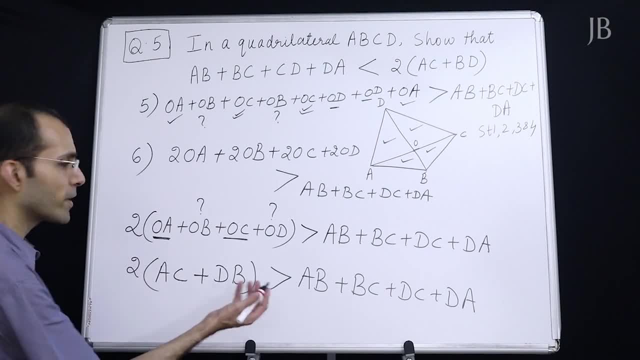 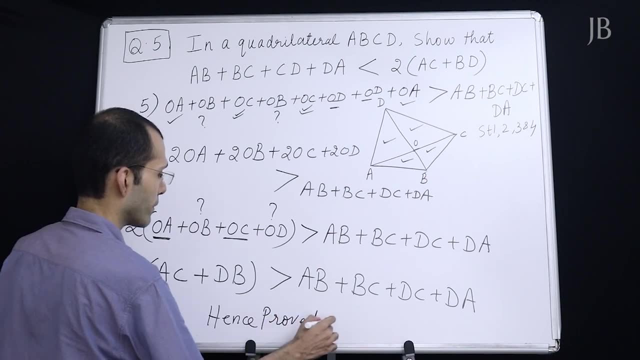 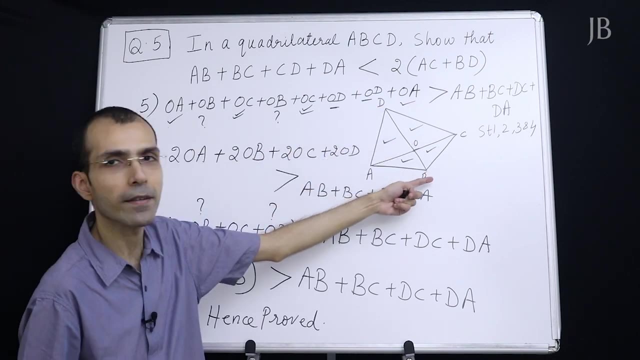 Here also, open mouth is towards this. So we have proved it, Hence Proved. And if you want to write any reason for this replacement, Then you can write D dash O, dash B. That is straight line. And A dash O, dash C. 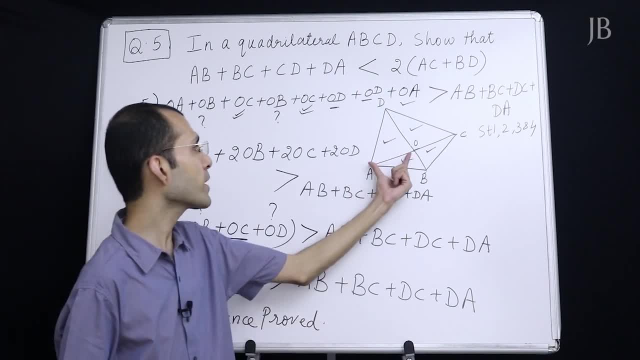 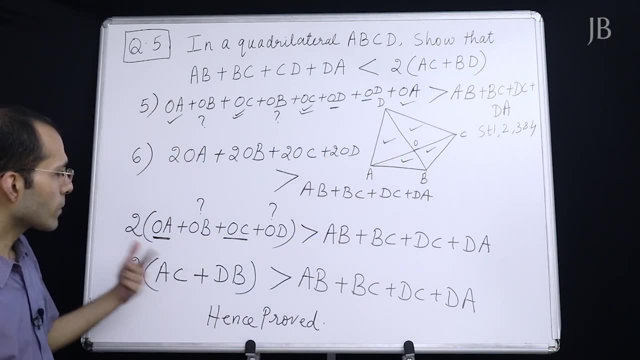 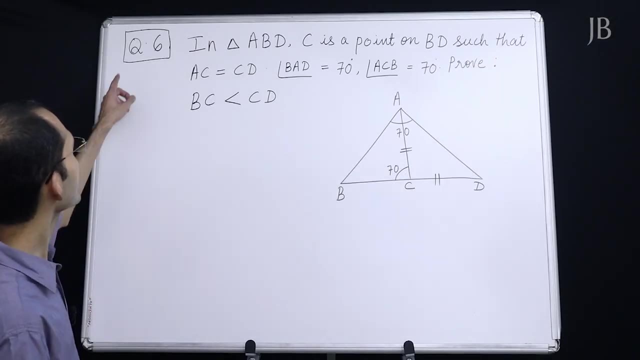 Straight line Points are collinear. Therefore AO plus OC will give us AC And DO plus OB will give us DB. That is what we have used And we are done with this. Question 5.. Question 6. In triangle ABD. 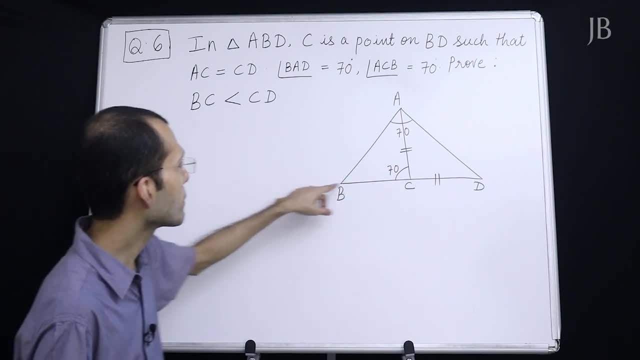 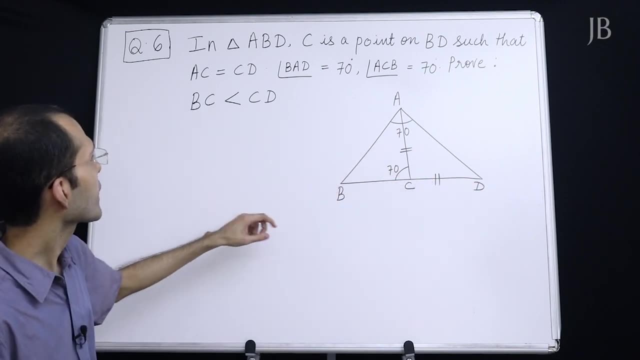 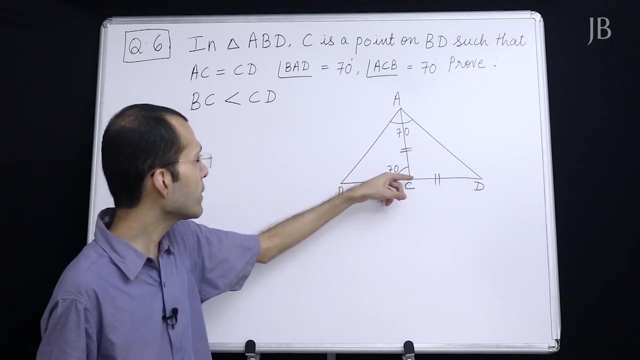 C is a point on BD, Such that AC is equaling CD. Okay, Angle BAD is 70.. The full thing, Angle BAD is 70. And angle ACB is also 70. See: angle BAD is 70. And angle ACB is 70. 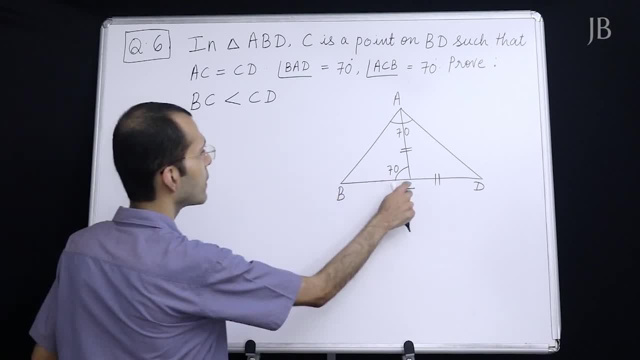 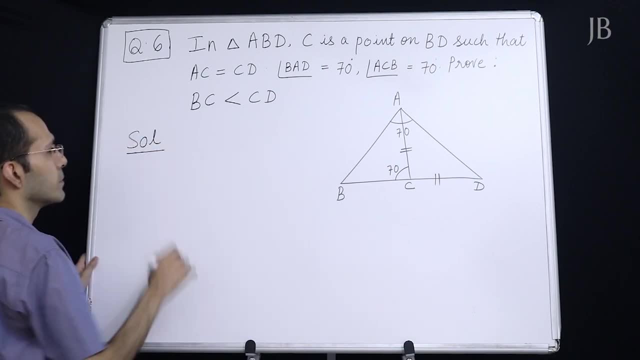 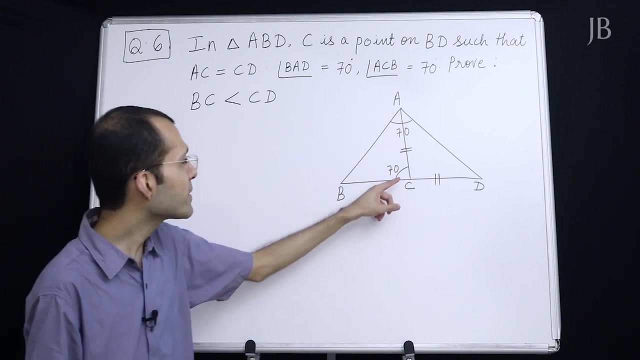 Prove that BC Lesser than CD. Okay, Prove that BC Lesser than CD. Now, if you go to see It is not such a straight forward sum Because BC comes in triangle ACB And CD comes in triangle ACD. 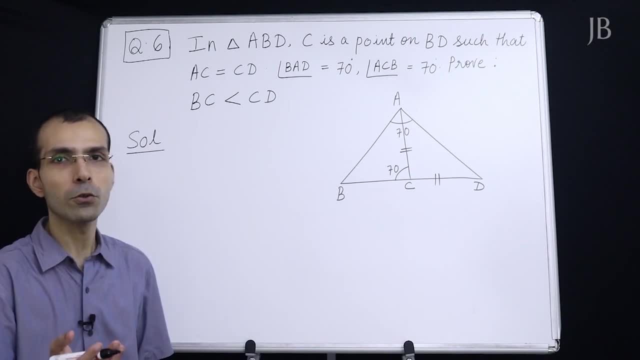 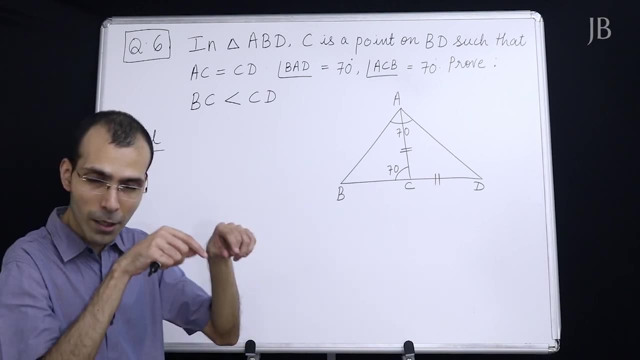 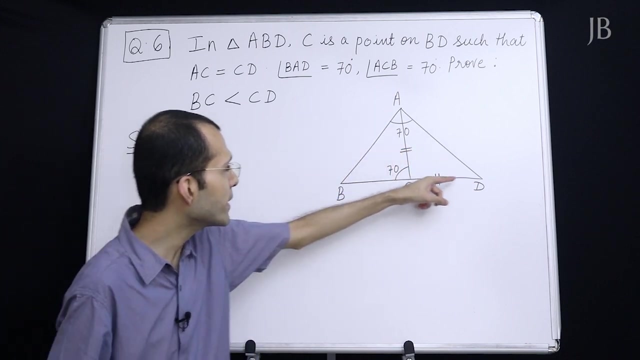 So that concepts, What you, What have been taught to you, That side opposite to greater angle is greater, Or angle opposite to greater side is greater, That will work in A particular triangle, Not two different triangles. So we see, We realize that AC and CD are given equal. 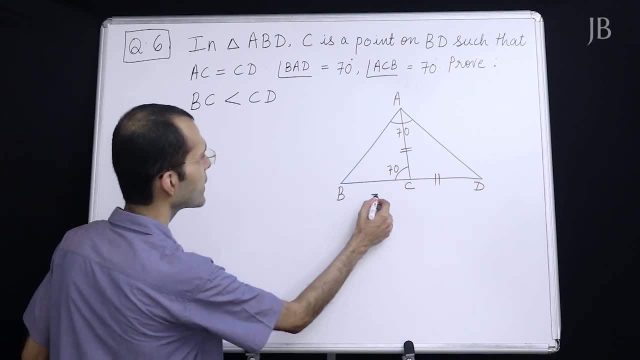 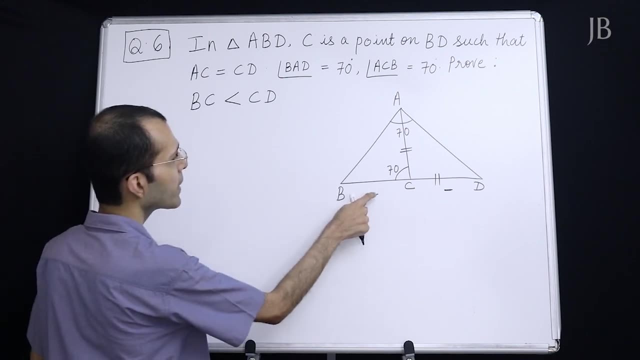 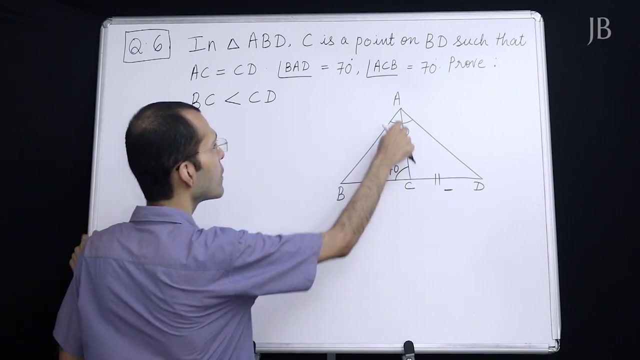 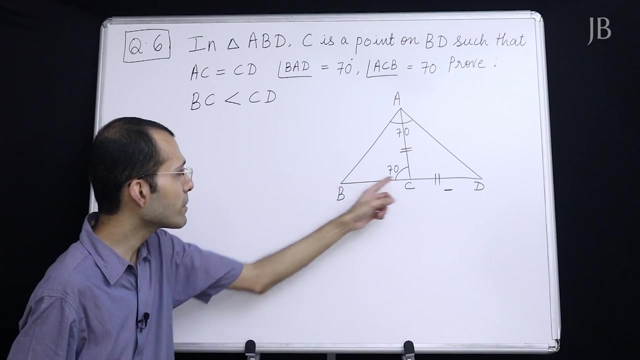 Right. So we are supposed to compare now BC With CD. So what we will do is We will compare BC With AC, We will compare BC With AC, And then AC and CD are equal. So the relation between BC and AC. 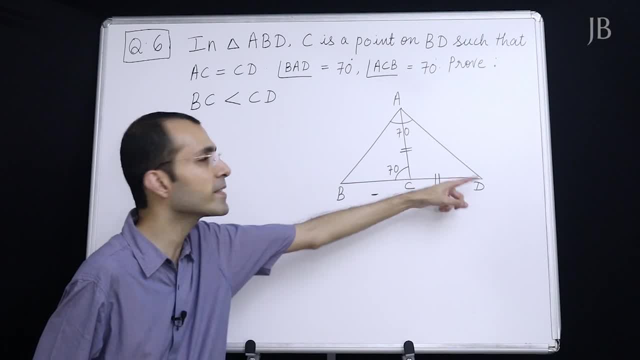 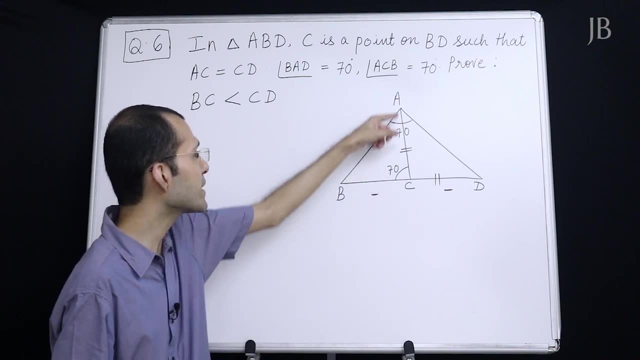 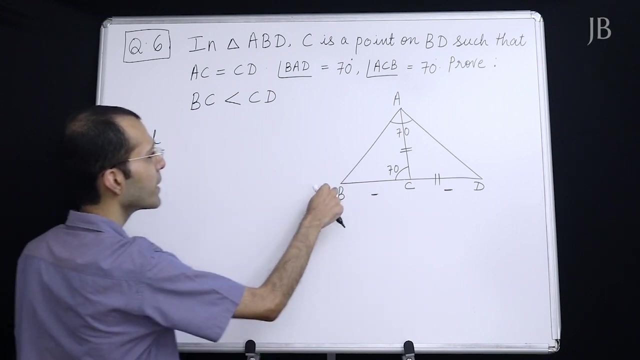 Will be same as between BC and CD, Because AC and CD are identical That way, And it is sensible To compare BC with AC Because both of them come in the same triangle. Right, You got the crux of it. So we will compare BC with AC. 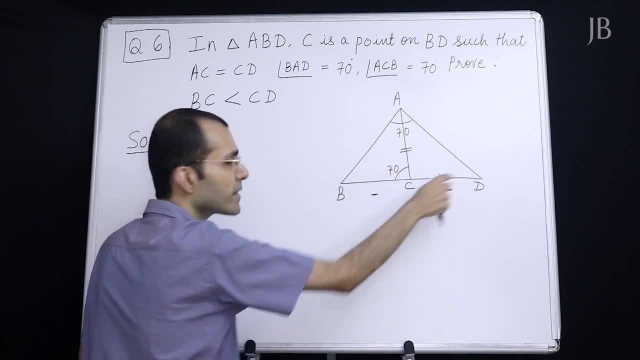 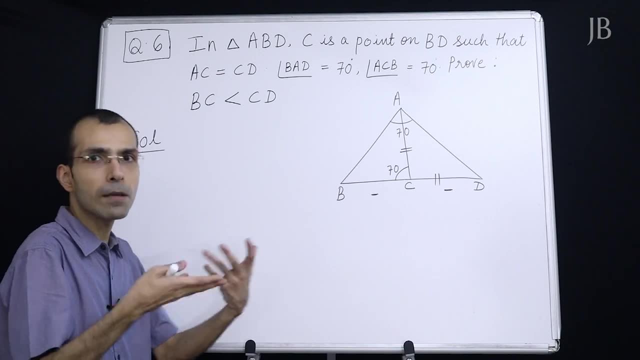 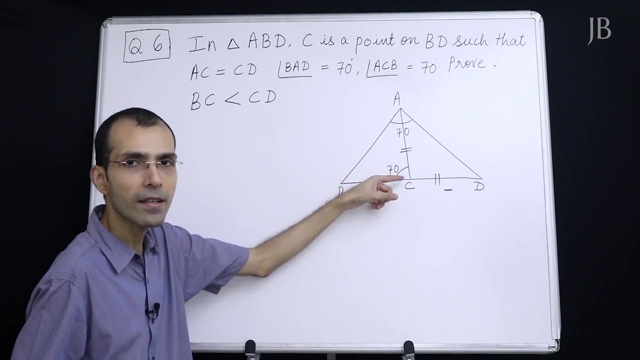 And then jump over to CD, Because AC and CD are same And BC and AC They come in the same triangle So we can compare also. And AC is given equal to CD. So whatever relation will happen Between BC and AC, 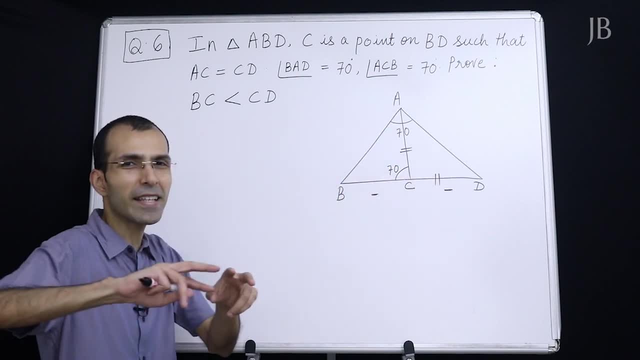 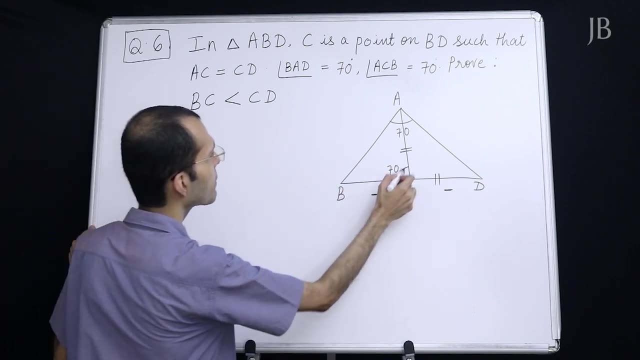 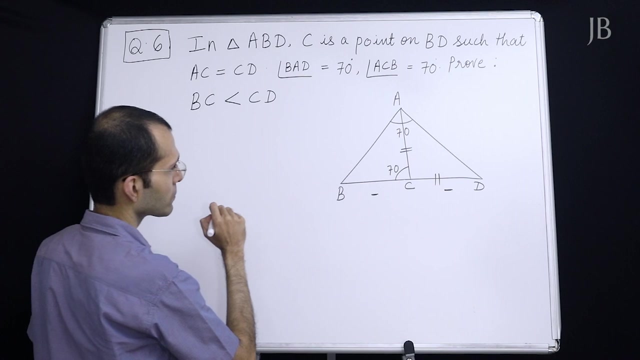 Same relation will hold between BC and CD, Because AC is getting replaced with CD On account of it being equal. Fine, If I have to compare BC with AC, We will have to find the angles. Now. this is 70.. This is 110.. 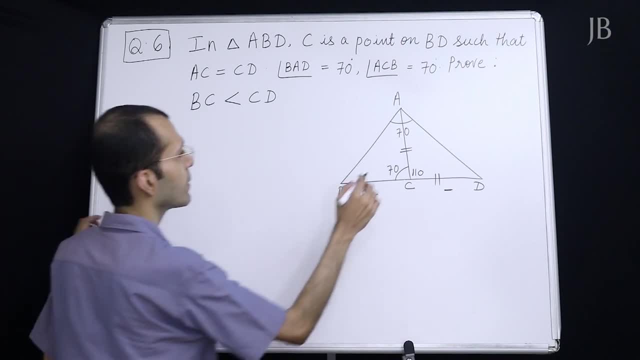 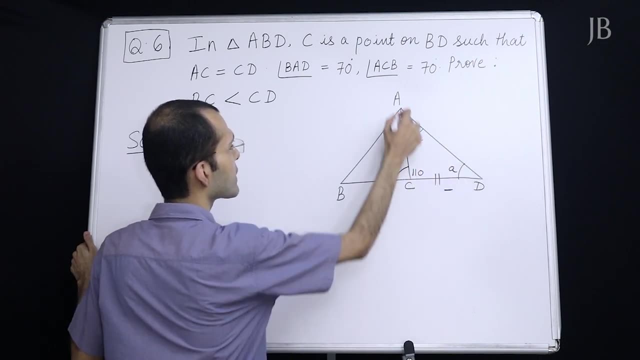 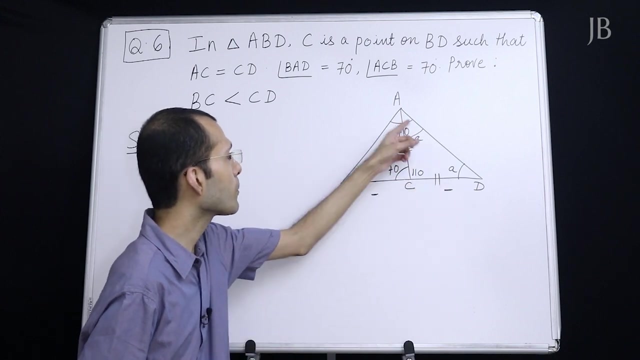 That is linear pair. Then this angle and this angle, Let it be say ANA, Because CA and CD are equal. If CA and CD are equal, The angles opposite to them also will be equal. Isocellus triangle concept: Fine. 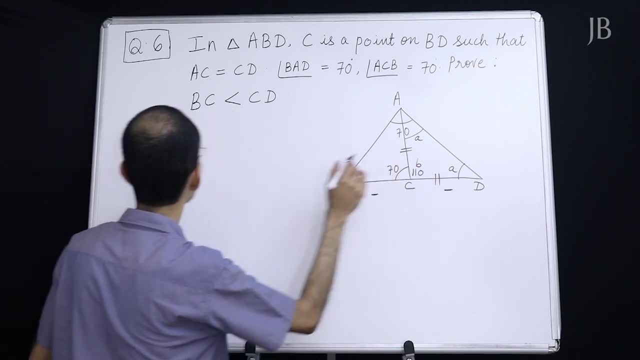 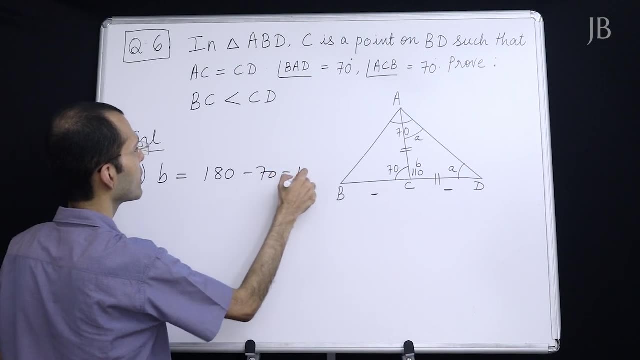 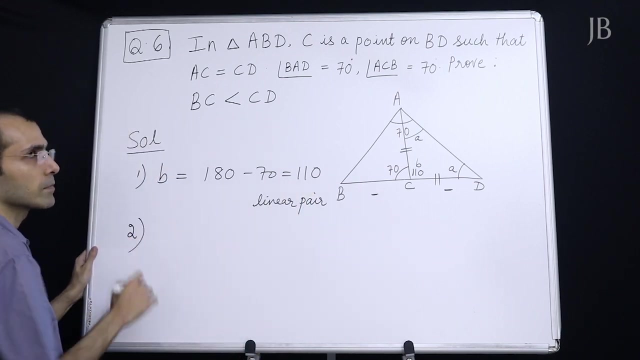 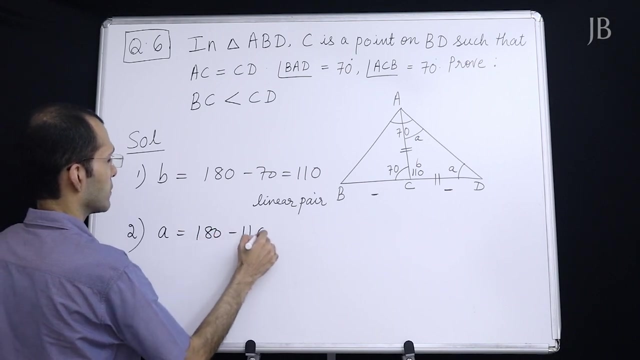 So now what we will do This: we will mark it as B, So it is easy. So B will be 180 minus 70.. That is 110.. Okay, What is the reason here? Linear pair. Now A will be. 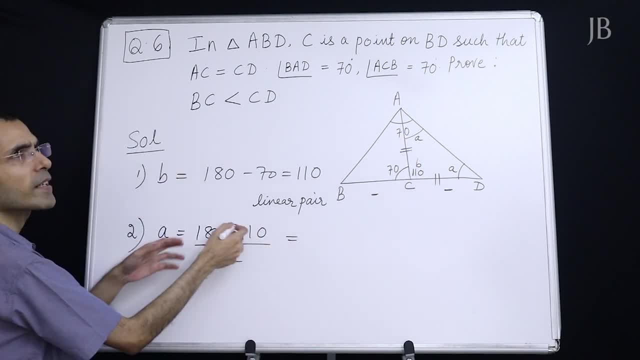 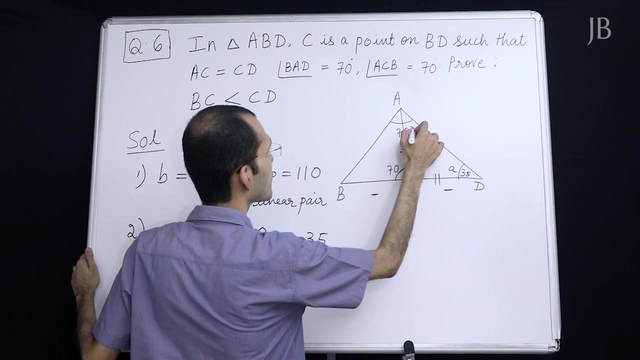 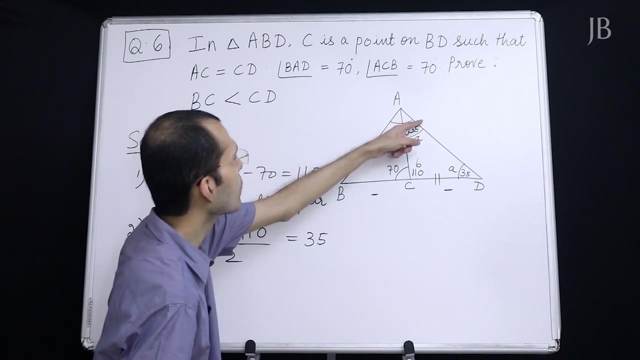 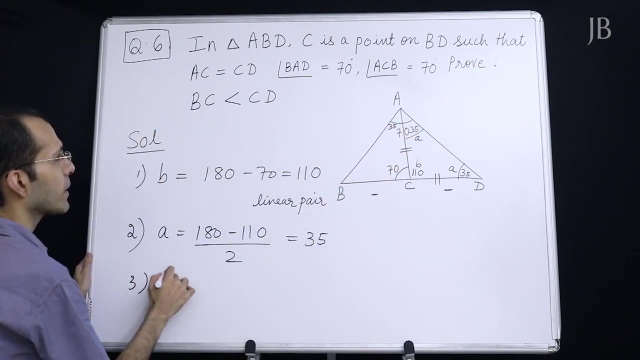 A will be 180 minus 110 upon 2.. So that is 35.. This is 35.. This is 35.. Okay, The full thing was how much? 70.. So this also will be 35.. Angle BAC will be 70 minus 35.. 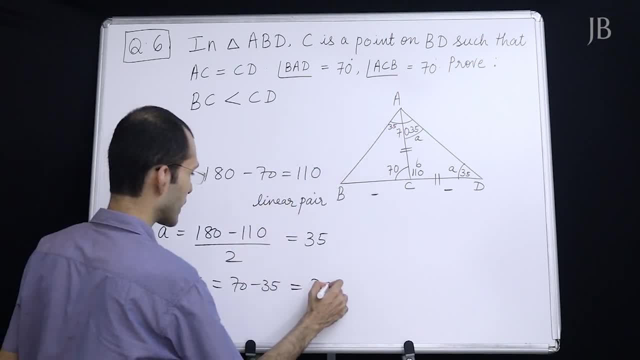 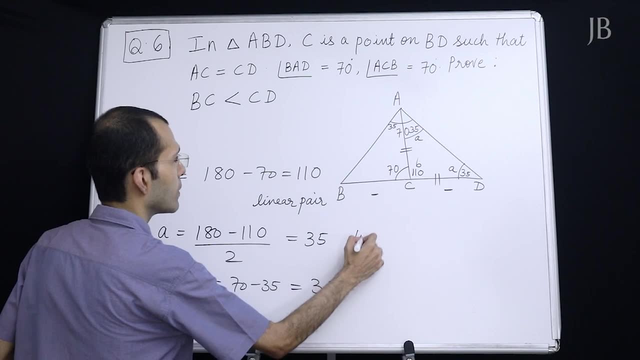 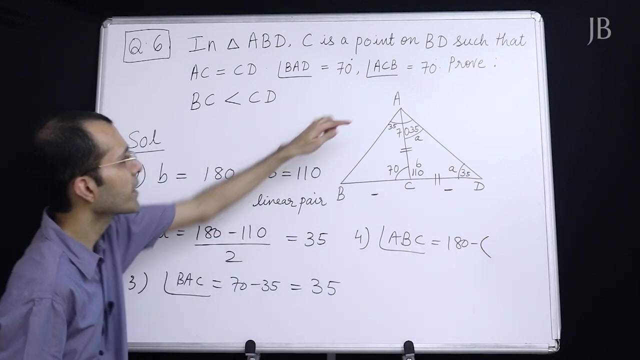 Because the entire thing was 70. So this comes to 35.. Okay, 35 and 70.. Now let us work out this angle: Angle ABC. Angle ABC will be 180 minus 35. This angle is 35. Angle BAC. 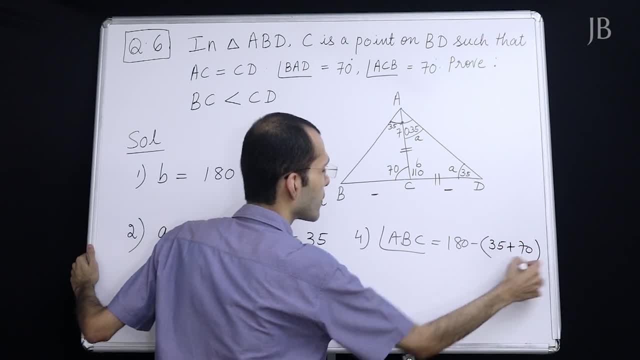 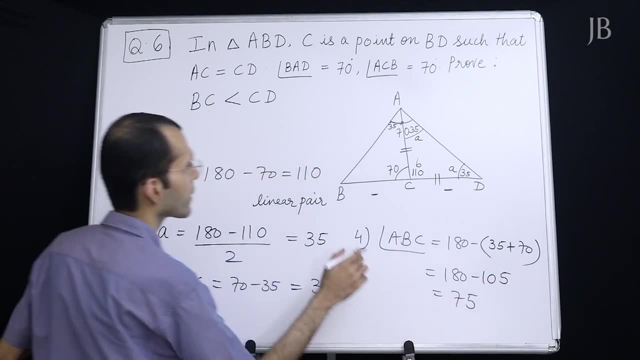 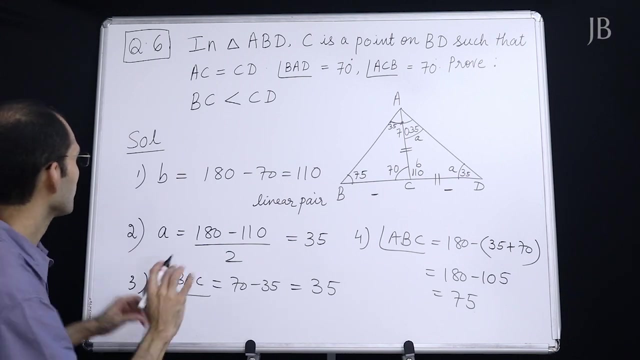 So 35 plus 70.. So this is 180 minus 105.. That is 75.. So this angle now turns out to be 75.. So we have worked out these angles, So now we can compare, So where we will take it. 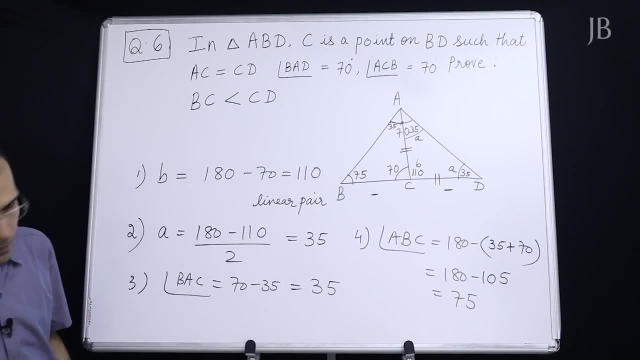 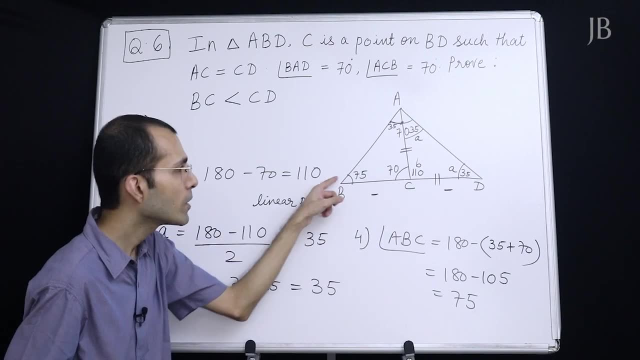 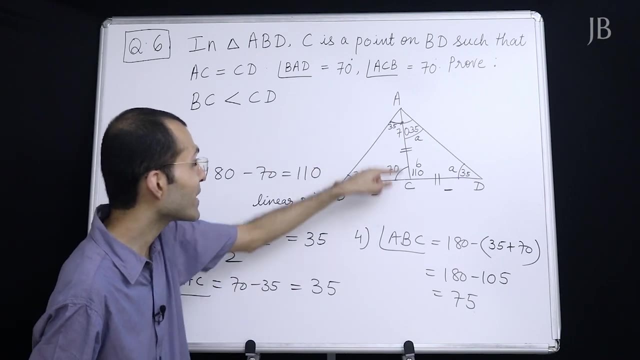 We will take it here only Statement number 5. We are supposed to compare BC with CD But, as I told you directly, we cannot do it Because they belong to two different triangles. So we will compare BC with AC And then cross over to CD, as AC and CD are equal. 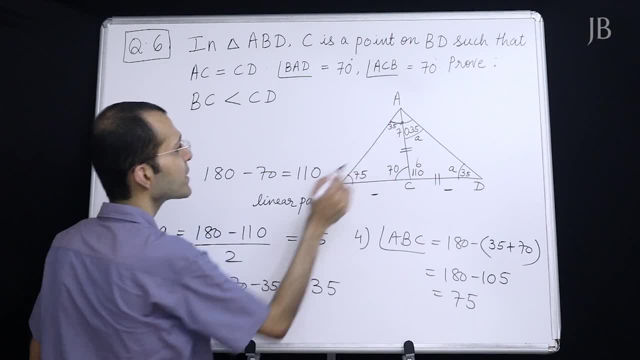 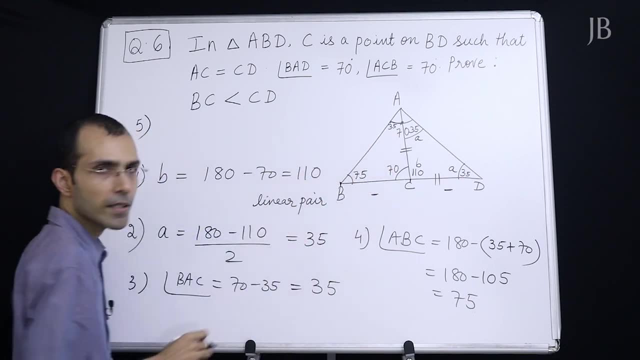 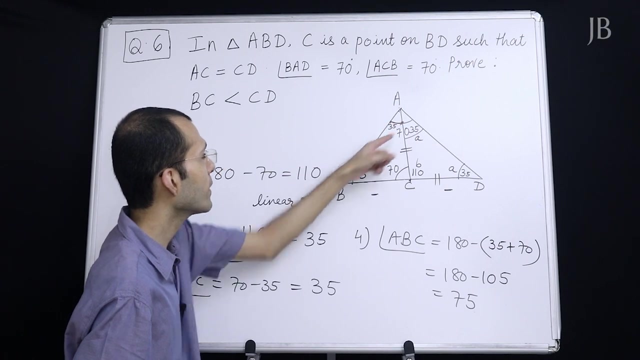 Now see BC is opposite to which angle? Observe carefully: BC is opposite to 35. And AC Now. we are comparing BC with AC first, And AC is opposite to 75.. BC is opposite to 35. And AC is opposite to 75.. 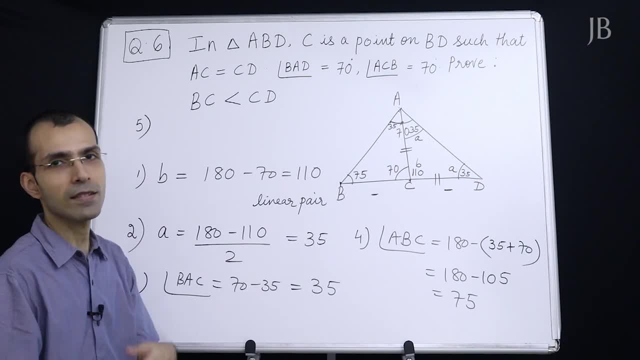 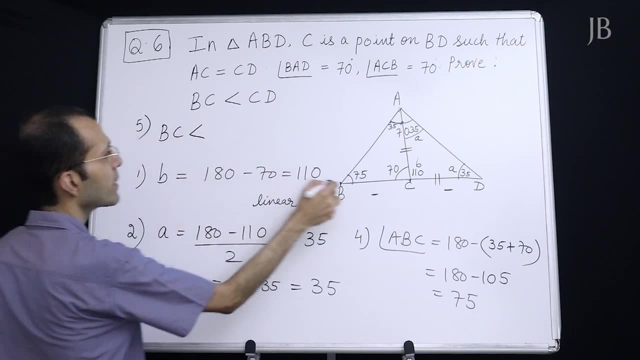 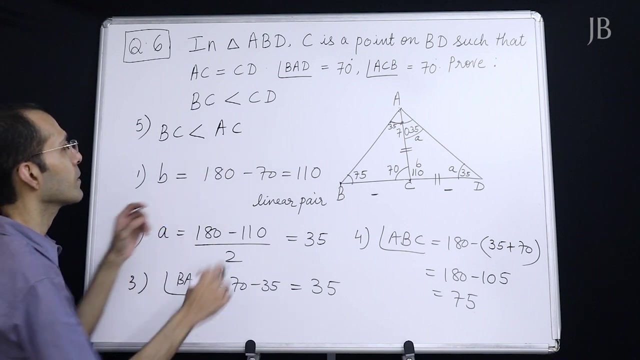 In the same triangle. So which is greater or which is lesser? BC will be lesser. So here BC will be lesser than AC. Agreed, What reason will we write for? here We will write side opposite to smaller: angle is smaller. Or we can write side opposite to greater: angle is greater. 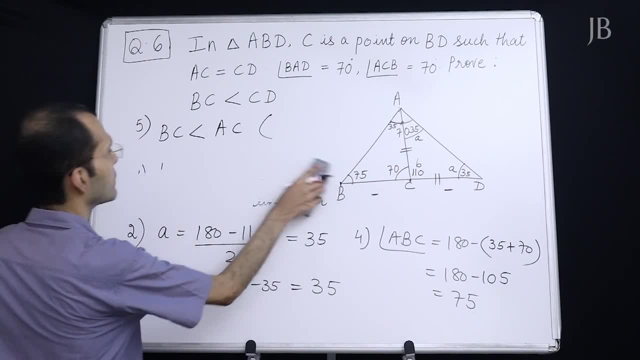 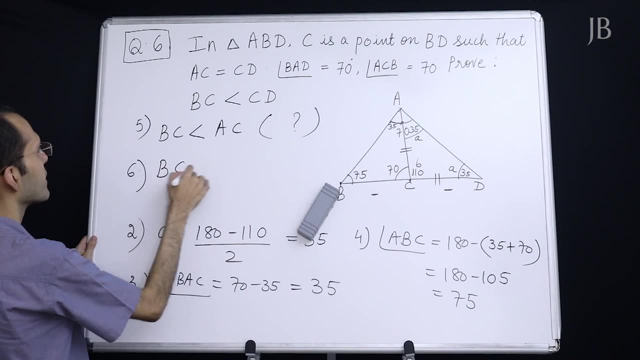 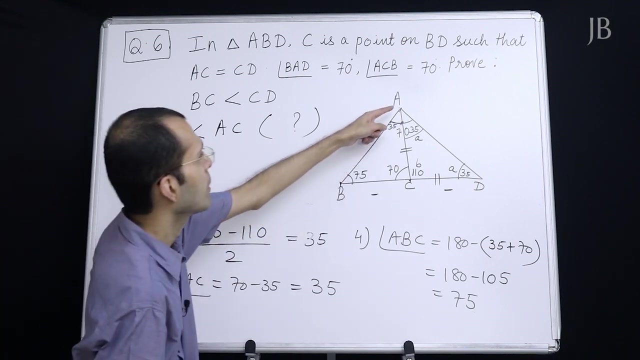 I mean one implies the other. This reason you will have to write it Now, BC. you keep it as it is, Because that is what we want. It is lesser than AC. This has now been established. But AC and CD are equal. 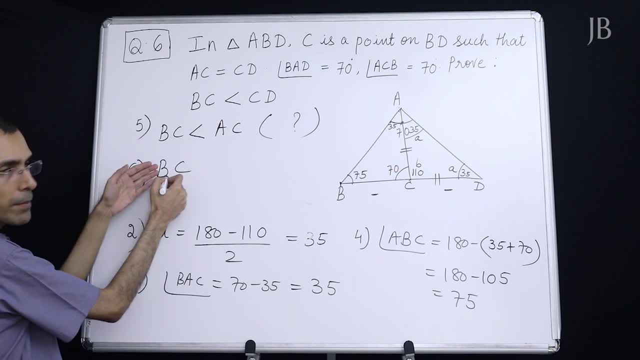 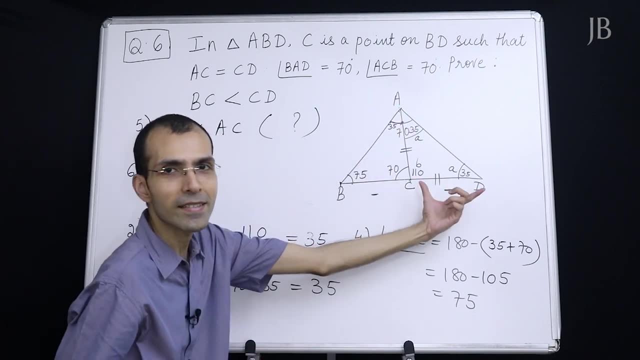 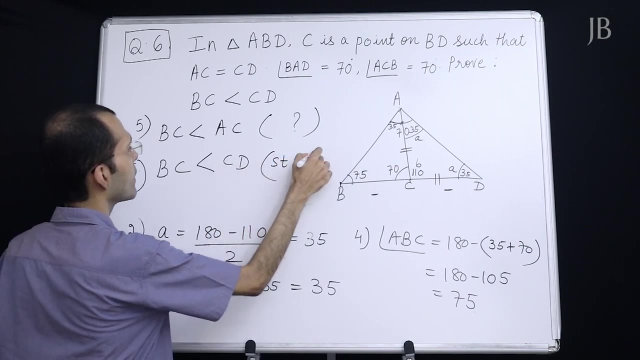 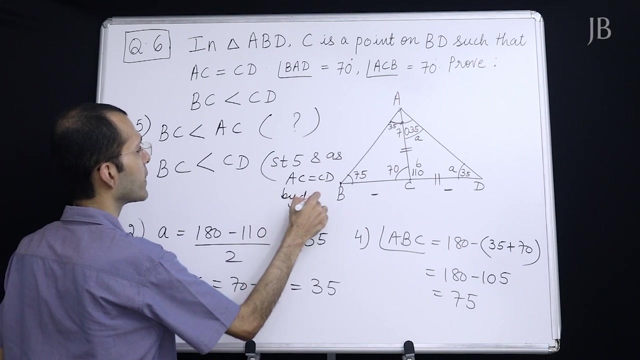 Why Already given. So I copy BC, Same sign. I copy This AC. we replace with CD, As both of them are equal. Here the reason will be Statement phi and as AC is equaling CD by data. So that is what we had to prove.